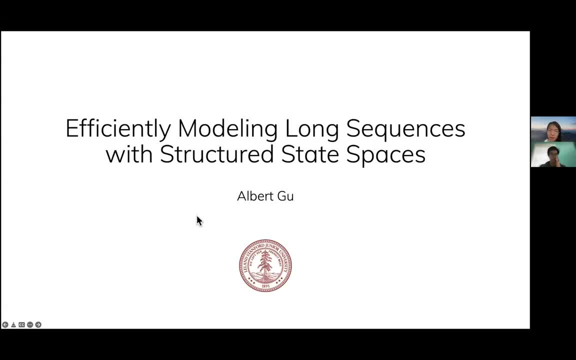 Okay, Hi everyone. Welcome to our 41st session of the MAIT AI Group Exchange. This week we have Albert Gu from Stanford here with us to present his research on efficiently modeling long sequences with structured state spaces. Albert is a final year PhD candidate. 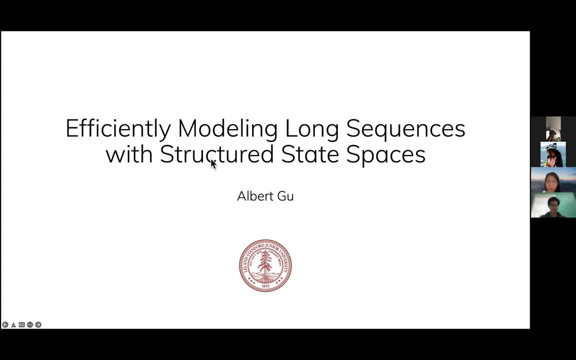 in the computer science department here at Stanford University. advised by Chris Ray, He's broadly interested in studying structured representations for advancing the capabilities of machine learning and deep learning models, with focuses on structural linear algebra, non-Euclidean representations and theory of sequence models. Thank you so much, Albert. 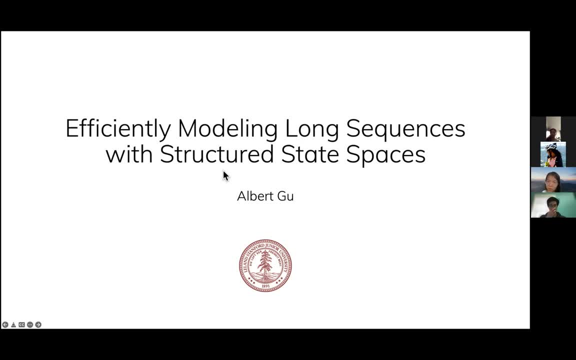 for joining us today. Before we start, do you have any preference on how you want to take questions? Yeah, Thank you. Thank you for the introduction For this talk. I think I'm not sure usually the level of formality, but I'm very happy. 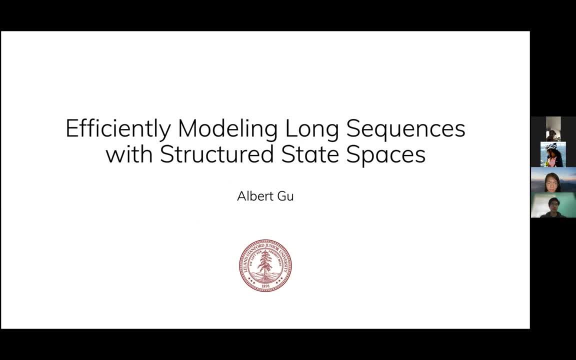 to have it casually In terms of the conversation and the questions. I think there's some time. It's not going to be a full hour talk, so I'm more than happy to take questions during it and I'll watch the time in case it gets too long. And then I'll also pause a few times to pause for potential. 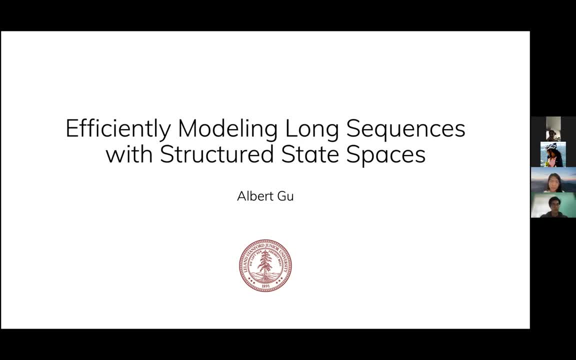 questions during some sections. Okay, Sounds good. Let's try to make this session as interactive as possible. Without further ado, let me hand it over to Albert. Thank you, All right. So this talk will be about a new sequence model called S4, or Structured State. 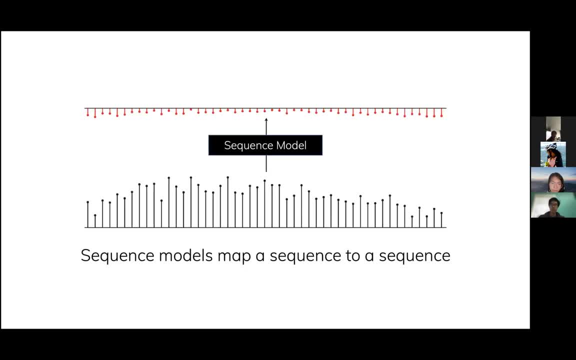 Spaces. Now for the purposes of this talk. when I mention sequence models, we will think of them as a black box, sequence-to-sequence map composed of primitive layers, where each layer simply takes an input sequence and returns a sequence of the same shape. 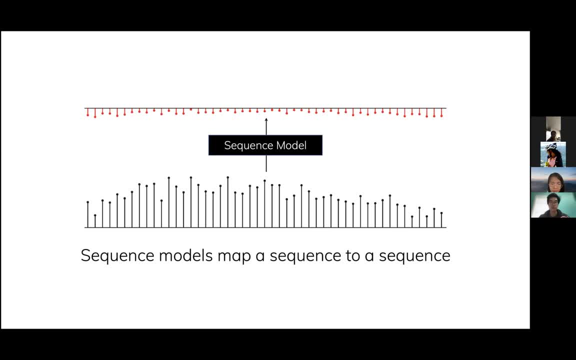 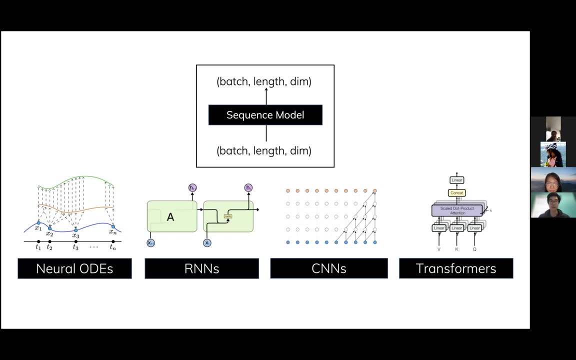 For our purposes right now, we will think of them as just being a one-dimensional to one-dimensional map, but this can be easily converted to higher-dimensional features. Many sequence models have been developed that satisfy this interface, particularly in the context of deep learning. These include many classical deep learning models such as recurrent. 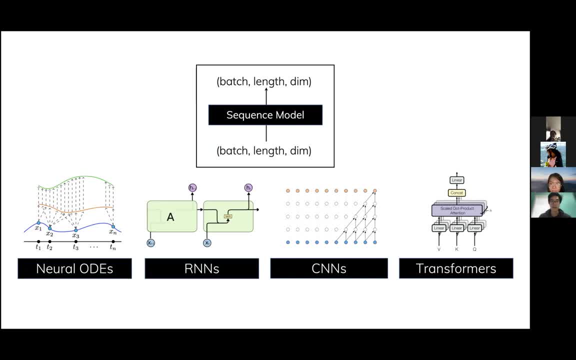 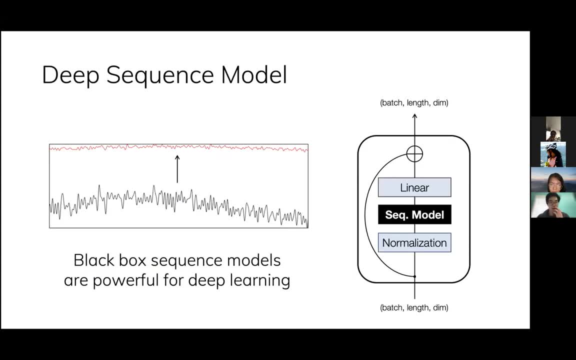 neural networks or RNNs, and convolutional neural networks or CNNs, as well as many more modern models such as transformers or neural ODEs. All of these models kind of satisfy the same interface. They map a sequence to a sequence. 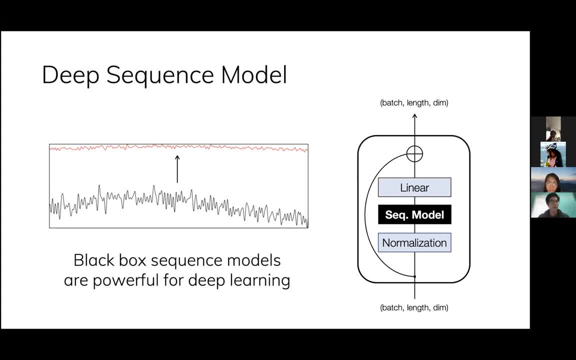 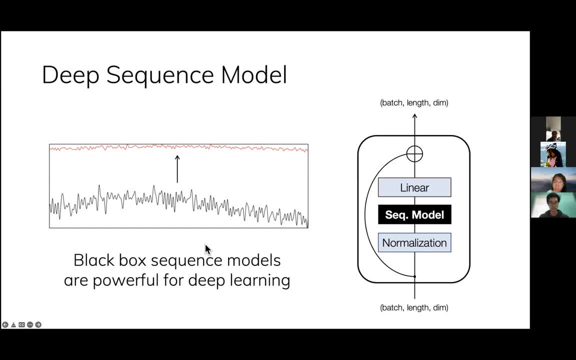 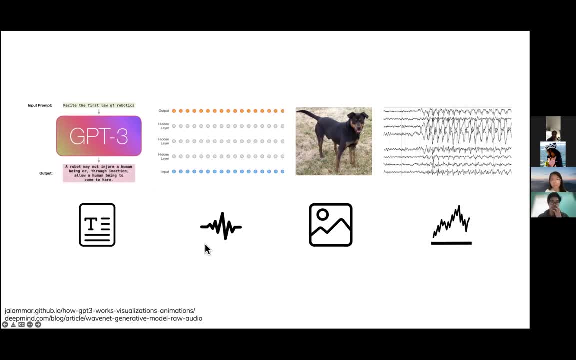 Okay, Okay. And the other core component of all of this is the core sequence model, and that's what we'll focus on. And this generic deep neural neuro architecture based on sequence models can be used to solve many types of problems with many types of sequence data from modalities such as text. 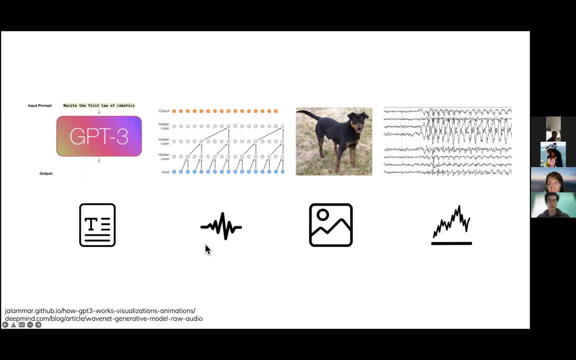 in audio, to images and videos, to general time series data or biosignals, for example, which is depicted here. Okay, Okay, Bye, Bye. In this talk, I'm going to draw a very rough distinction between different types of sequence. 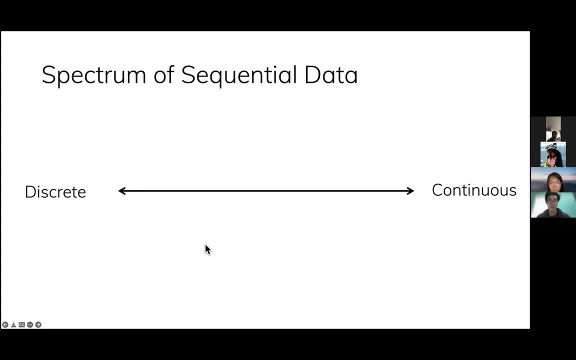 data. Now, much of modern sequence modeling in the context of machine learning focuses on data such as text, And very roughly I'll classify this as being a discrete sequence, because the input comes in the form of discrete tokens And other types of data like this includes things like graphs or things like DNA-based. 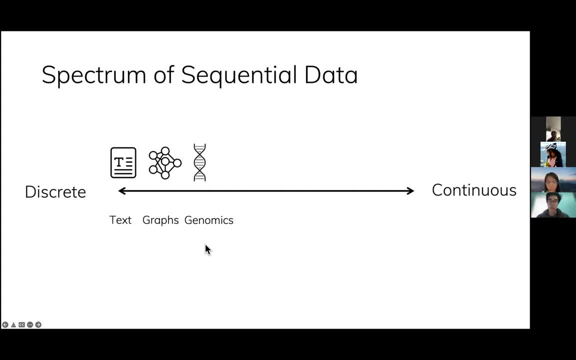 pairs. In contrast, what this talk will focus on is data that's roughly more continuous things, such as video or time series or audio, And what's common to all of these is that there's an underlying notion of time from which this sort of data is sampled from. 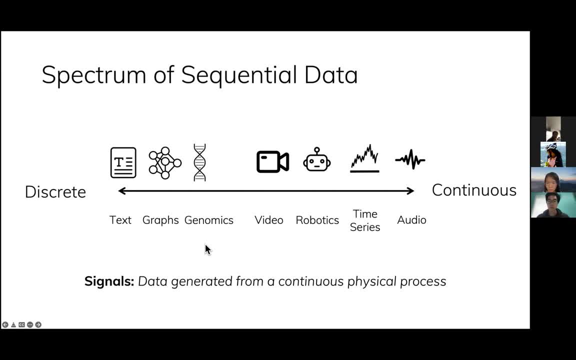 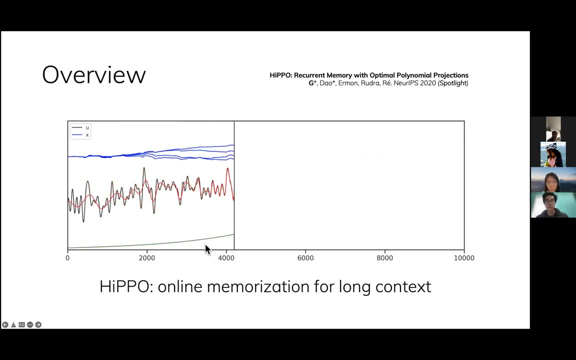 And so I'm going to very broadly call this type of data signal data, as opposed to sequence data, And, roughly speaking, signals can be defined as data that's generated from an underlying, continuous physical process. Including all these examples here, This talk will be composed of two parts. 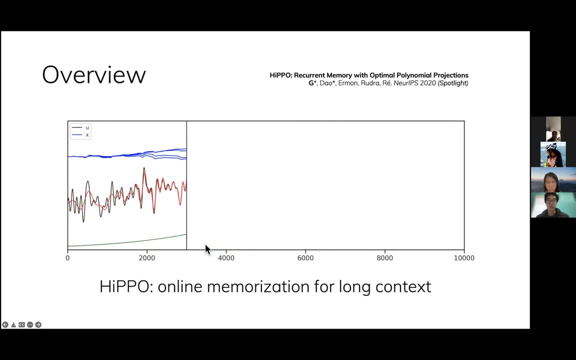 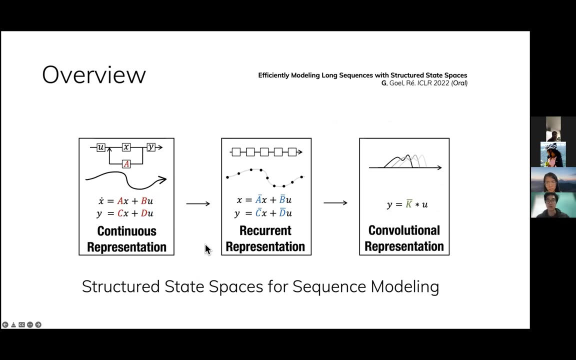 The first part covers a method called HIPPO which was the predecessor to S4. And it's a new conceptual framework for the online memorization of signals and led to a new method for modeling signals and sequences. And then the second part will be S4, which built right on top of HIPPO. 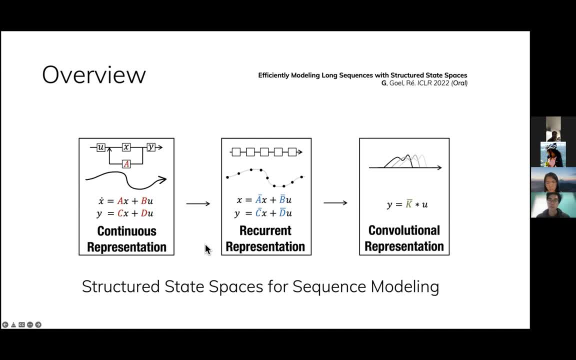 And it has a lot of important properties that have been very effective for addressing some types of sequence modeling. And before I get into the technical stuff, I'll give a quick preview of experimental results to highlight the types of improvements that we'll see and what it's good at. 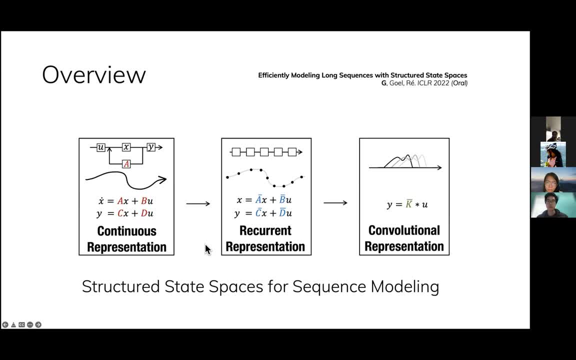 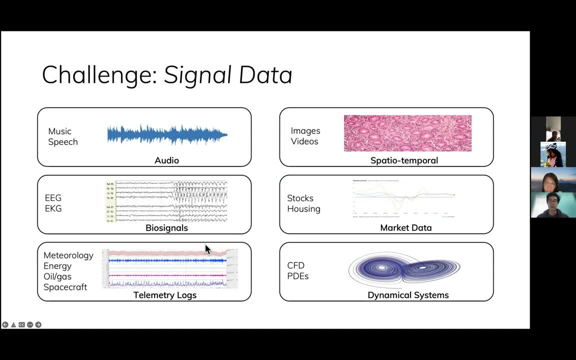 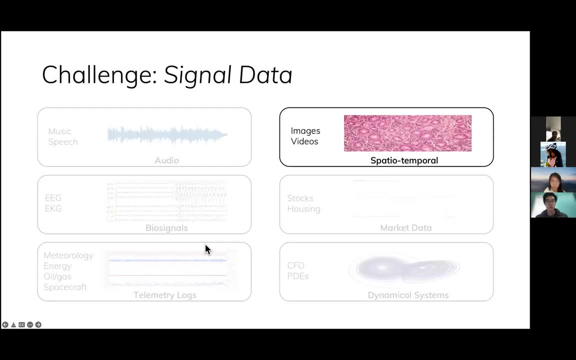 And this will kind of illustrate the types of challenges that we'll hope to address with these new models. The first challenge overall is just going to be to signal, or general temporal data that I just defined, And this data is really everywhere. So some examples include audio waveforms, spatial temporal data like videos, biosignals. 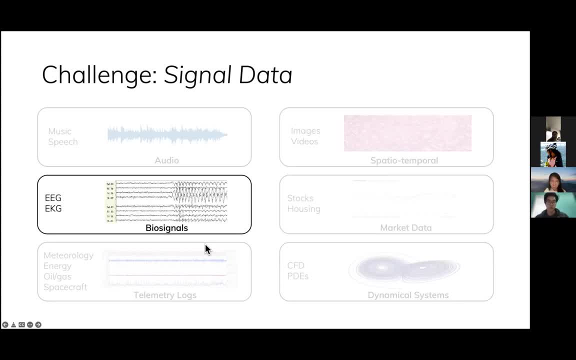 like electrocardiograms, which have important applications in medicine. all market and financial data, all time series logs being generated by every major industry and many other types of scientific modeling problems, And we'll return to these experiments later, with a particular focus on some biosignal. 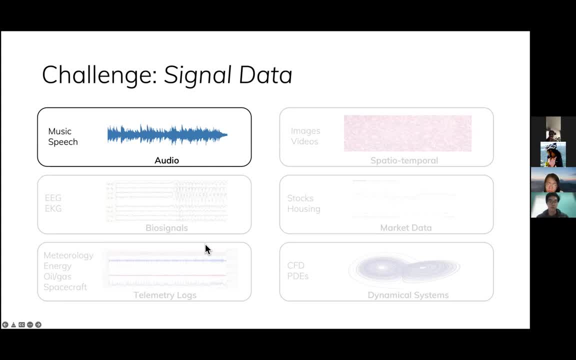 data, But for now I will just use one example to illustrate which is audio, And audio is actually one of the most common types of data, Because it's just raw sound, It's everywhere, And so to illustrate machine learning right now is really all about text. 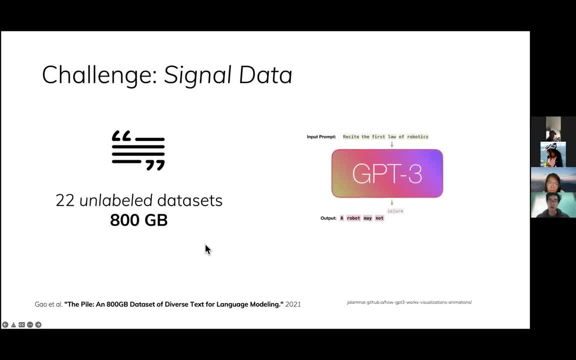 And so many headline results recently have been about people scraping together all the raw text data they can get, creating massive models on them, And that's led to very impressive results, like GPT-3, which I don't know the audience, but hopefully many of you have heard of this model. 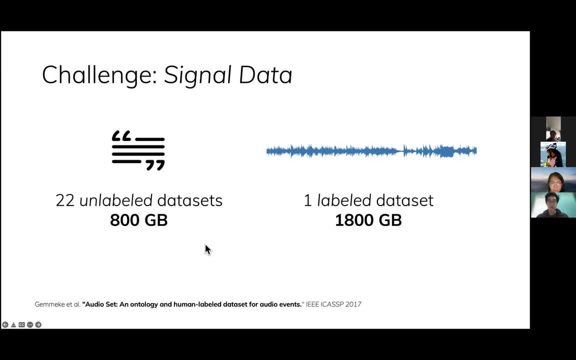 In contrast, audio actually has orders of magnitude more data than text. For example, a single labeled data set has more data set than text, And that's because the data set has more data than text, And that's because the data set has more data than text. 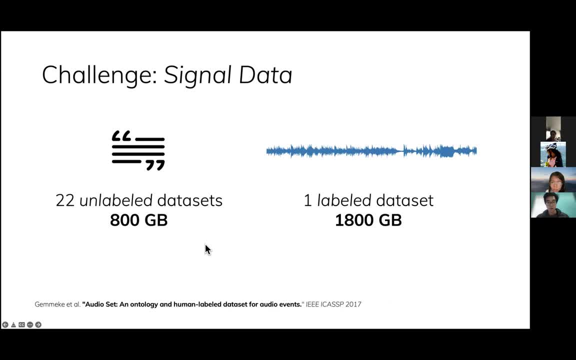 And I'm sure you've heard of this too, But it's less data set than all of the data used to train those massive language models. But you don't hear about benchmarks in this domain nearly as much, And I think part of the reason is just because audio models are. 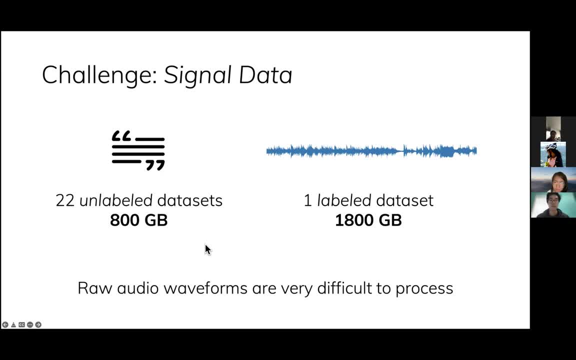 Audio is very challenging and current models see much worse in comparison to text, And so here's a concrete example where we considered basically a very general and hard audio generation setting of generating spoken digits 0 to 9.. using a completely unconditional autoregressive model. 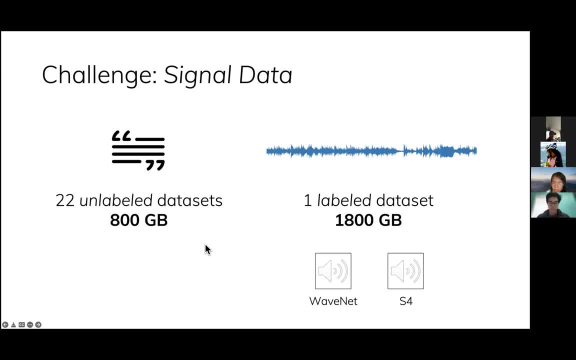 And the gold standard. here is a baseline called WaveNet, And here's what it sounds like trying to say these numbers. So it's it's not very good. And here's the results for S4, which was just. these results are just from. 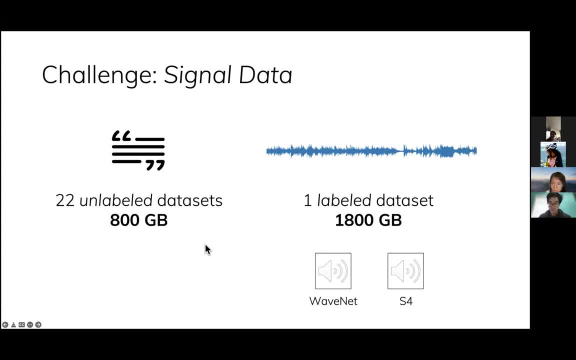 the past two months or so ago: 1,, 2,, 3, 4.. So that's, that's a pretty concrete example, And so in this talk we'll see how models like S4 are kind of designed for signals, in a way. 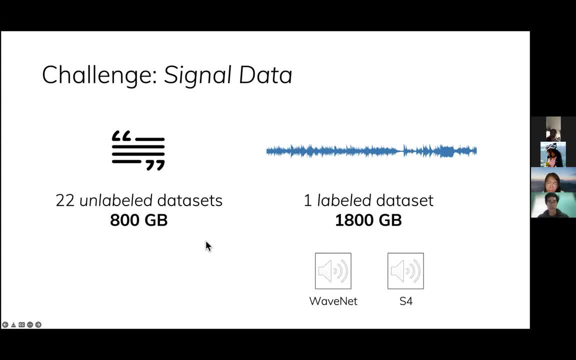 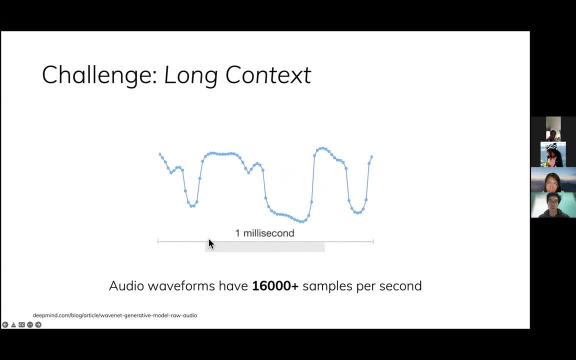 and can have significant advantages for this type of data. And the second example up front. the second example of a running challenge will be: can be motivated by examining audio more closely, And one reason why audio is so hard is because it's sampled at such an extremely high rate. 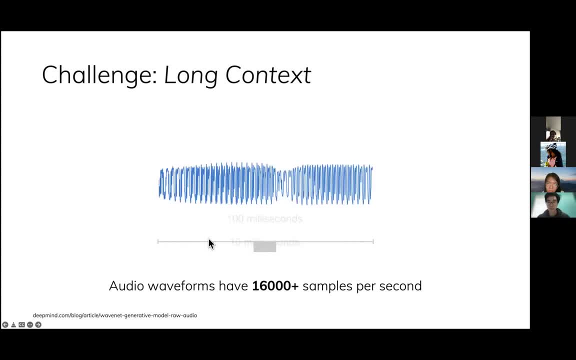 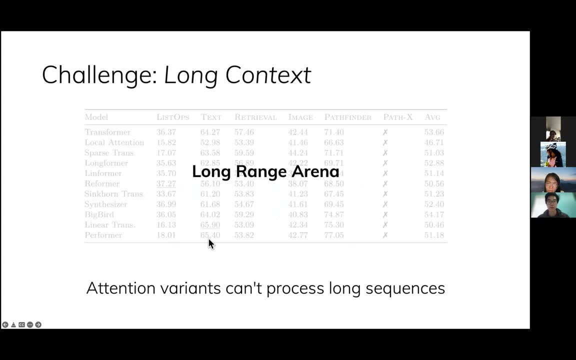 where a single second has 16,000 or more samples. Well, in contrast, most sequence models can't deal with more than a thousand or so. And to illustrate, there was a benchmark in the past year called Long Range Arena that measured the performance of models. 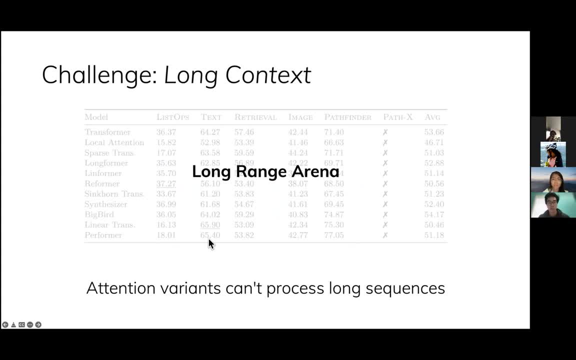 on a suite of long range tasks And the most popular sequence models these days. transformers were the main focus, But despite their many successes, they don't do so well on long context, And so there were dozens of variants that were tried. 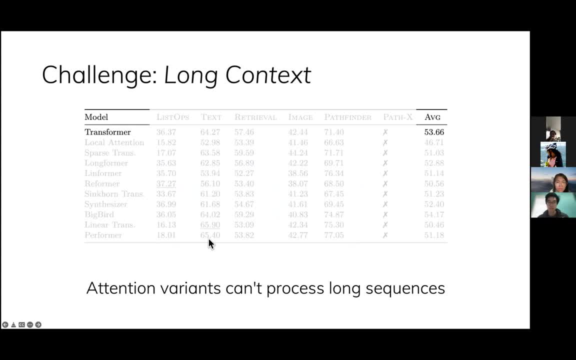 and they all get to around the same performance, which is actually not much above random guessing. In contrast, S4, we'll see, is explicitly designed to be effective on long context, which leads to a huge improvement on this benchmark, And it's the first model to ever make progress. 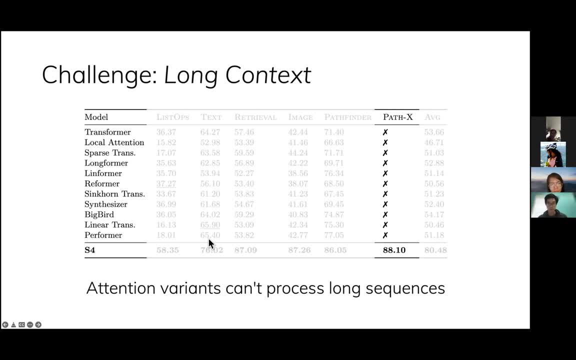 on some really difficult long sequence tasks. Can I ask a quick question here, Albert? Yeah, So in the previous task that was a generative process And in this the long context challenge. is it a classification or what kind of task is it? 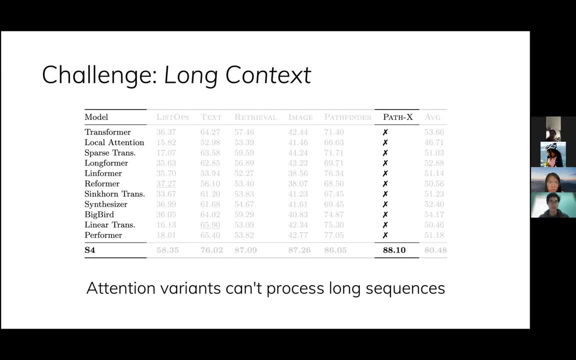 These are all classification problems And they're on data. that includes several data modalities, such as text, images, some sort of symbolic processing stuff like that I see, And so you can use S4 both as a generative model to actually generate sequences. 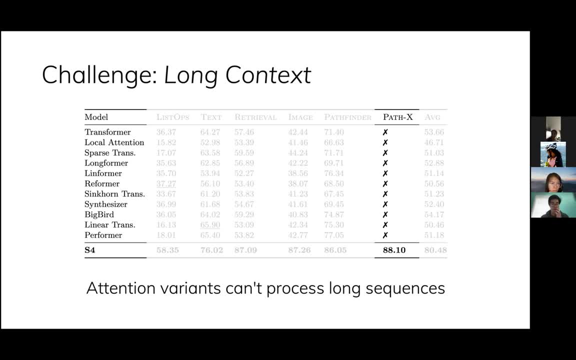 Yeah, So a lot of sequence models. again, a sequence model I'm defining, as this is a black box interface, really that's just a sequence to sequence map, And many of these can be used in many ways, both for classification and generation. 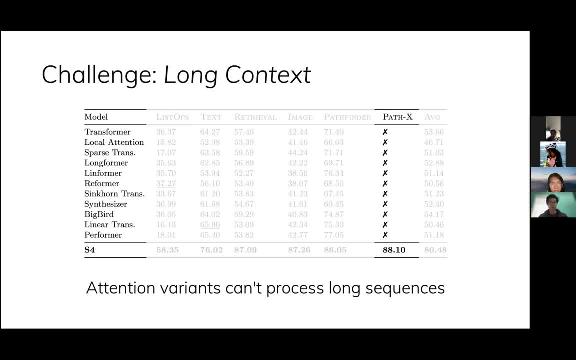 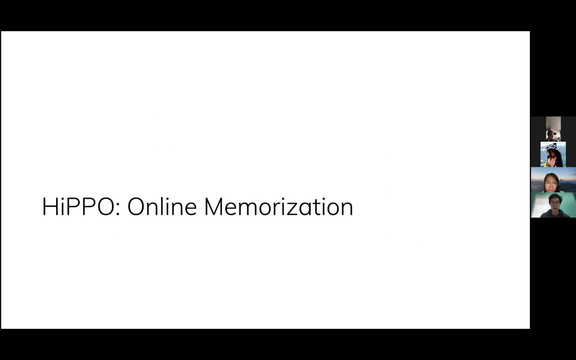 For example, transformers or RNNs are similar things that satisfy the same interface and can be used in many ways as well. Gotcha, Thank you, Yeah, Okay, so now I'll get into the technical portions, And the first part will be about HIPPO, as I mentioned. 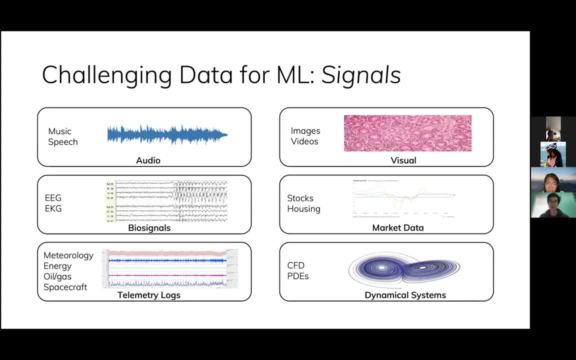 And to motivate what HIPPO does, I'm going to use a little bit of code. HIPPO's goal was: I gave a bunch of examples of data that machine learning models currently struggle with, particularly things like time series, And to highlight why this is hard. 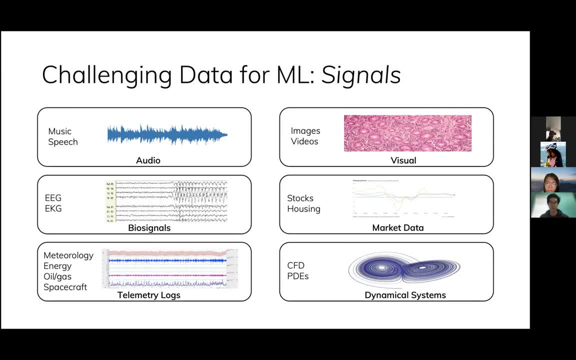 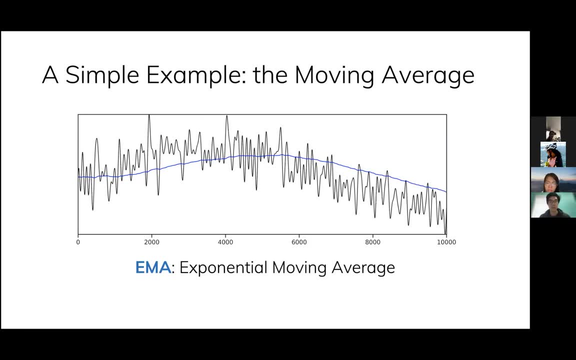 I'm going to use a running example to illustrate a very basic capability that's difficult for modern models And that's the moving average, which is perhaps the most basic method in modern time series analysis. So this figure depicts the exponential moving average, or EMA, which is the blue line. 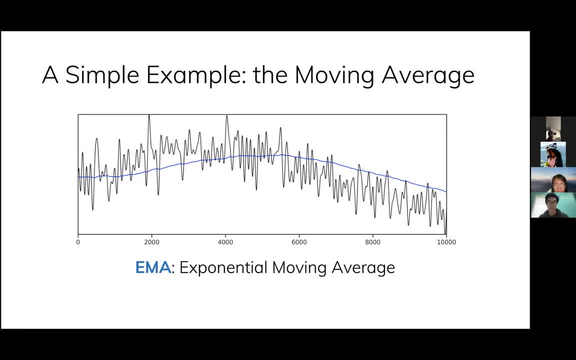 And the way it's used is that it's the fixed. it's a fixed, non-learnable feature. that's often the first pre-processing step that's performed in any sort of time series analysis pipeline. Now, in the context, in the spirit of machine learning and deep learning, 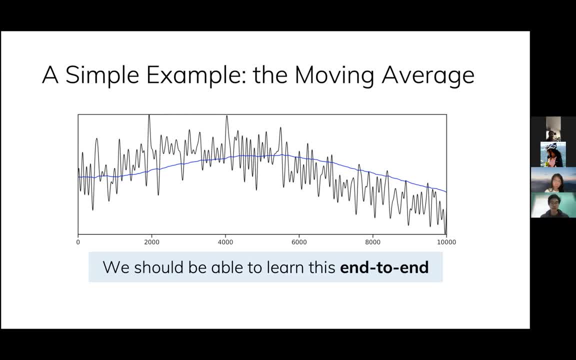 instead of doing manual processing like creating these features, we really would like to be able to learn these sort of things automatically from the data, And so, in particular, here's a very simple, concrete task. is suppose you have a model and you're feeding it this black input signal. 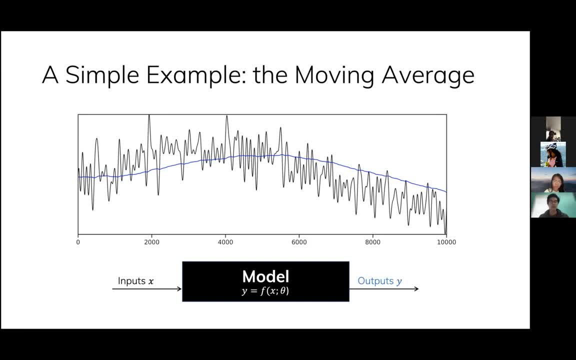 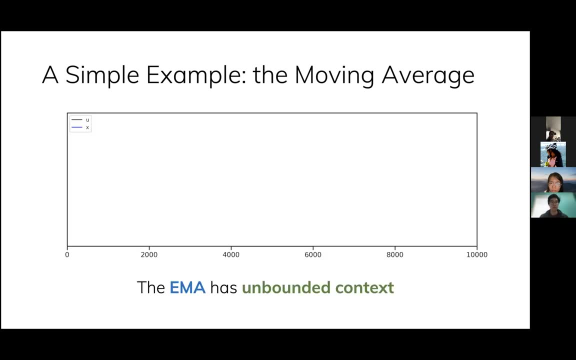 and you want the model to predict the EMA or the blue signal as the output. Unfortunately, it turns out that standard sequence models, such as attention and convolutions, cannot do this at all, And the reason why is essentially because the EMA has unbounded context. 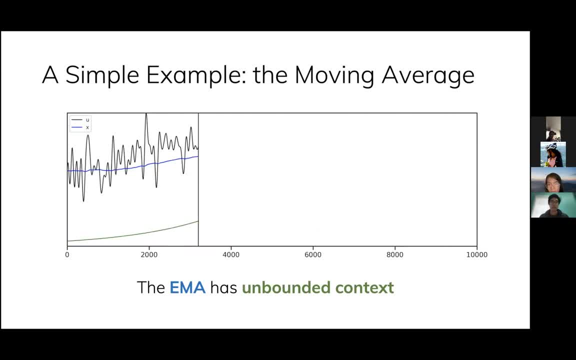 It's actually just a weighted average of the history of the signal, with an exponentially decaying weight that stretches back infinitely, Whereas, in contrast, most modern models such as attention or convolutions have finite context windows. Some people wonder about other things, like RNNs. 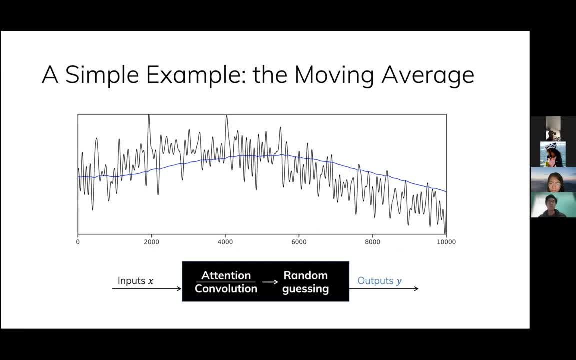 and the short answer is that RNNs are better than attention convolutions here, but they still aren't that good due to empirical problems with optimization and other things. So we'll see that the methods that are introduced in this talk will be very 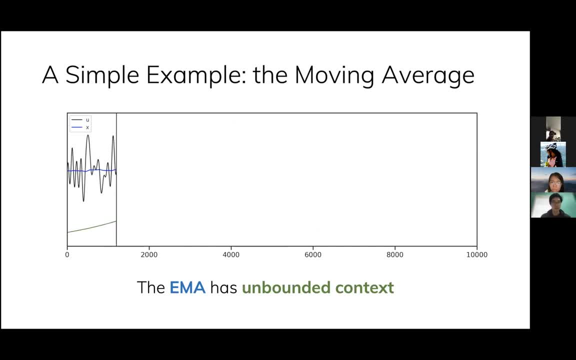 very naturally suited for this and are much stronger versions. But going back to the EMA, the way that, one way to think about it is that it's a very simple summary of the entire history of your signal. In other words, it's a state X. 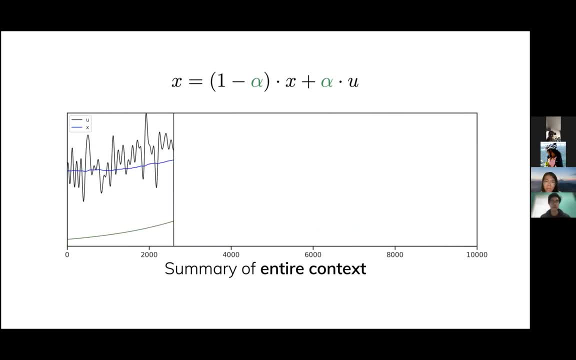 which is a single number that summarizes the entire history of the input U, And the reason why it's useful is that it's easy to compute, because if you get new data, you can update the EMA in constant time using this weighted average. 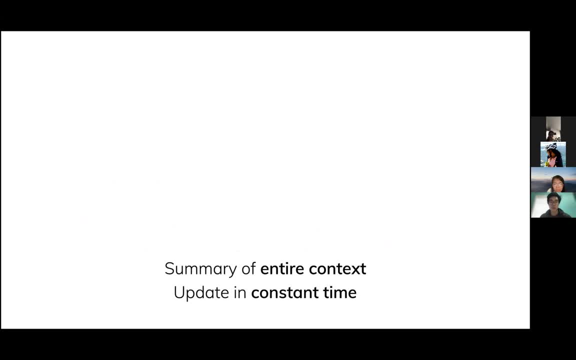 And beyond the simple example, though, I think these two properties are actually conceptually really important. For example, they're exactly the properties that you need in any sort of real-time decision-making problem And, really abstractly, you can even imagine that your brain is a state. 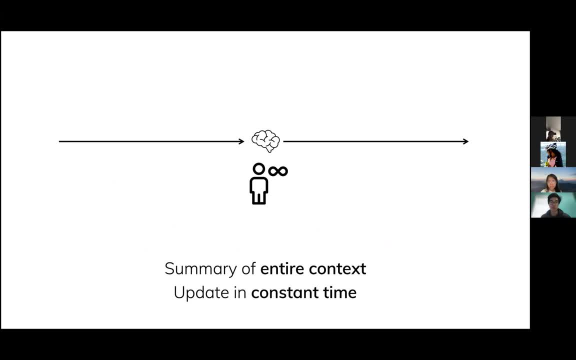 that's summarizing the entire context of your life and it's constantly updating as you acquire new information. So I think that's actually a pretty general, important question, and this was a direct inspiration for HIPPO In the context of machine learning. 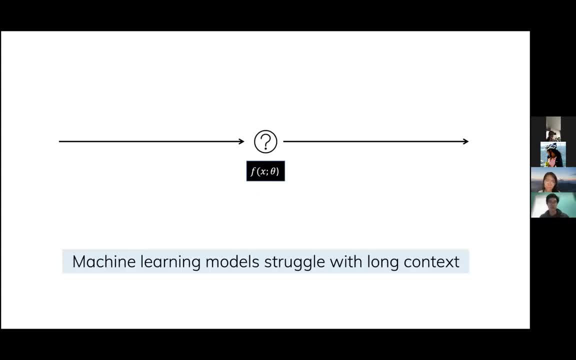 this question has a lot of direct impact on our models because, as I mentioned, they struggle with long context. For example, text models it's been shown to typically have a context range of about 100 to, at most, a few thousand tokens. 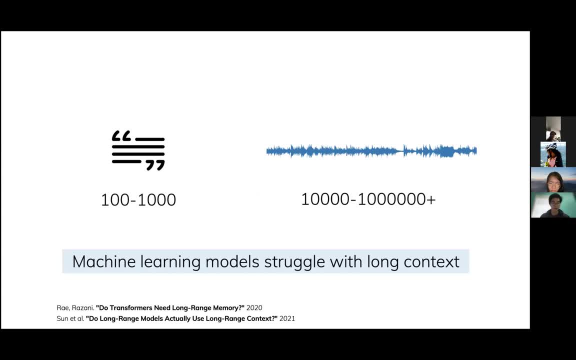 Whereas if you want to deal with data such as speech and audio, a single word in speech is a sequence of length more than 10,000, and this can really stretch to unbounded length, And so this is the question that I was thinking about. 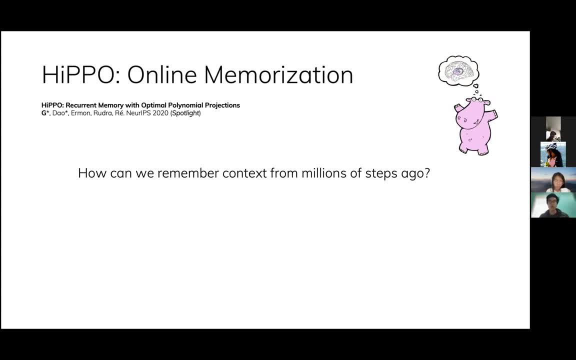 And what I did was I tried to convert this vague goal of long-range memory into a more formal mathematical question, And the conceptual idea is that if you can compress the past into a smaller state that's accurately remembering it, then you should be able to reconstruct the past. 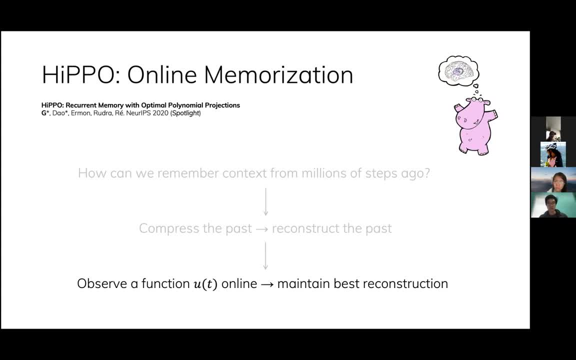 And we can then attempt to turn this into a technical problem. So the idea is that we're going to observe an input signal online and try to maintain a good representation of it that allows us to reconstruct it, And so okay, so first in this section, 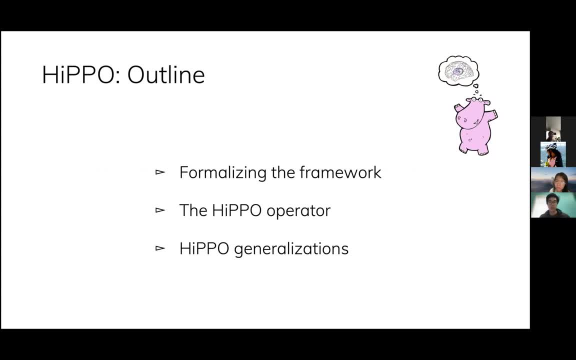 I'm going to formalize this And then I'll define HIPPO and visualize it and then talk about a couple of generalizations. So the first thing is that let me formalize this idea that I just mentioned, And so the idea of HIPPO is that again, 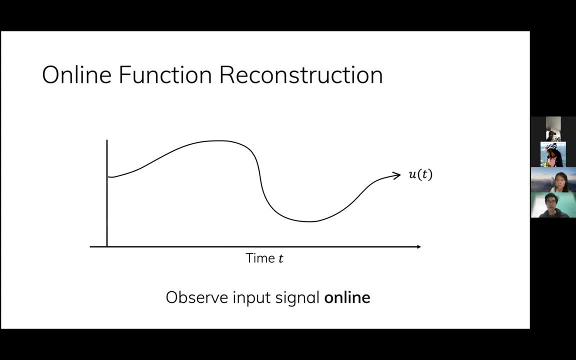 we're trying to observe an input signal online and we're going to try to encode it as well as possible, given a memory budget. So concretely, you can think of it like this: So suppose, at some initial time, t0,. 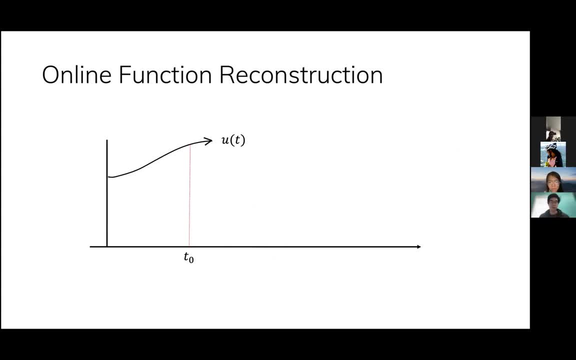 we've seen part of the input and we're going to try to compress this input, So all you can do is store the best approximation to what we've seen so far. For example, we can create the best polynomial approximation and write down the coefficients of that polynomial. 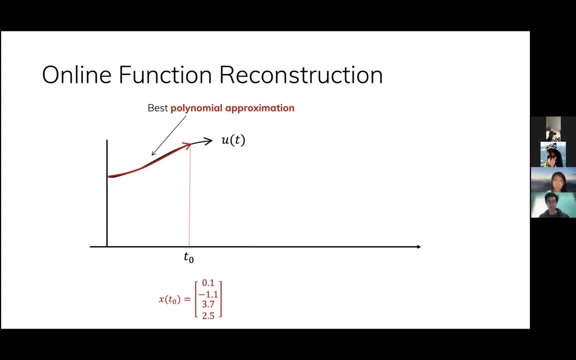 So now the degree of the polynomial, or the number of coefficients, is the memory budget, And we want to do this continuously, at all times. So as we keep seeing more data, at some later time- t1, we'll have to update our best approximation. 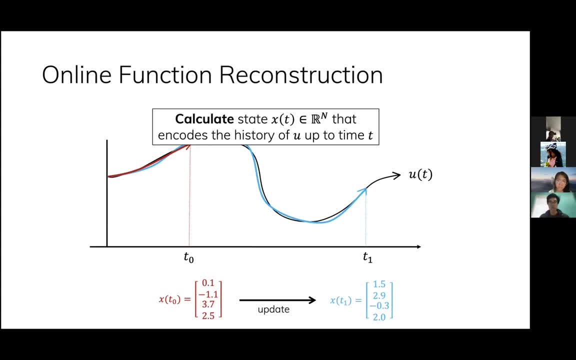 and write down the new coefficients, And now the central question is is, first of all, how do you actually find these optimal approximations And, moreover, how can you update this representation efficiently, as you keep seeing more information? And so this is the main conceptual idea. 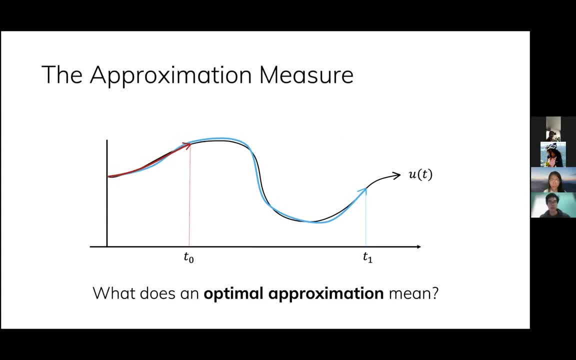 It needs a little bit of work to formalize a little more, And, in particular, I've been talking about optimal approximations, but that's actually not well-defined, And so what we'll need is to find a measure that specifies the quality of approximation. 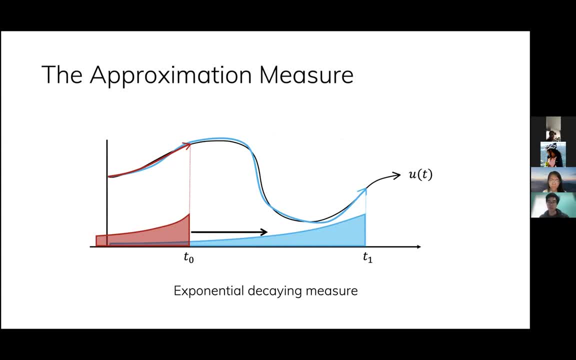 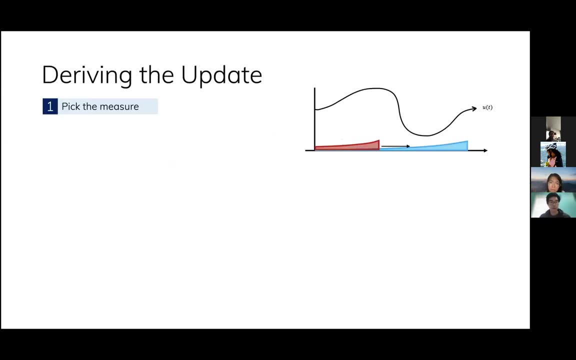 For example, we can choose the exponentially decaying measure, which says that we care about approximating the recent past of the input more than the far past, And this will relate back to the EMA. But given this, the problem is more or less well-defined. 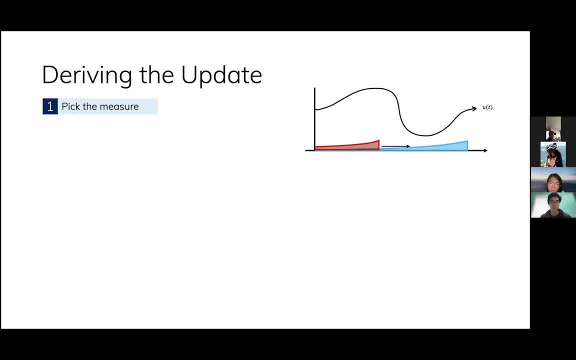 So basically we have to pick the measure as a hyperparameter or a prior for now. Later I'll talk about how you can actually learn it, But for now we need to pick a measure up front, So say the exponentially decaying measure. 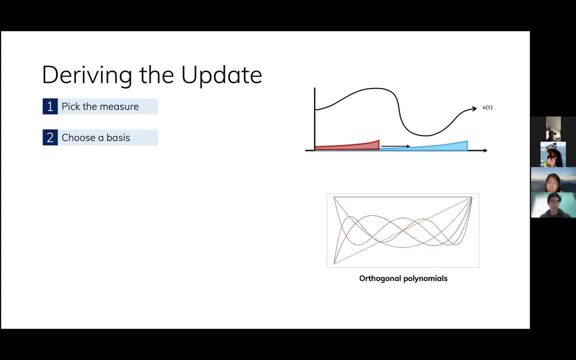 And then you need to choose a polynomial basis And then the problem is completely defined And you can write down the coefficients in closed form And you can figure out how they evolve through time. So I'm going to skip the details of the derivation. 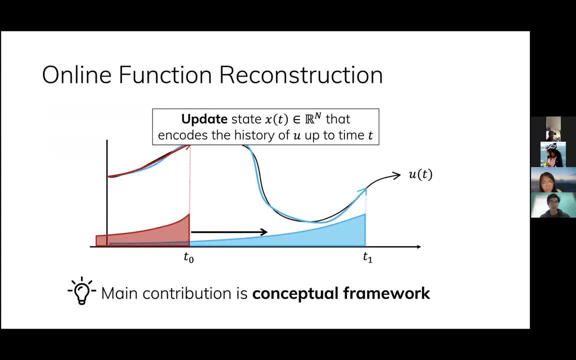 But you end up with the closed-form method And what I want to emphasize is that the derivation has some technically interesting new ideas, But the most interesting and important part of this, I think, is just this simple conceptual idea- All right idea of the online compression and 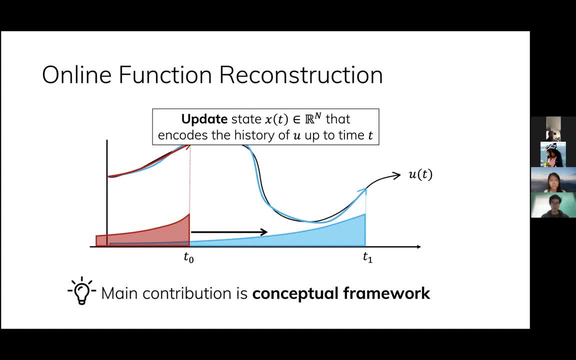 reconstruction and how to formalize that mathematically. So that's the main point, Okay, And now? now with the definitions out of the way, things will become a lot more clear with some visualizations of what it does. So first of all, let me just be. 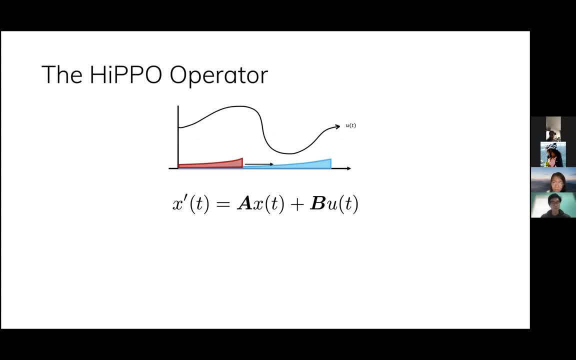 really formal about defining what hippo is So. so I mentioned the problem was that we're encoding, So x of t is going to represent a vector of our coefficients at all times, And the question is: how does this evolve through time as we see more data in the input? u. 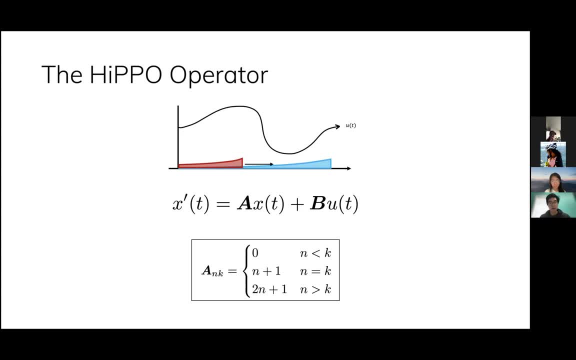 And it turns out that it just satisfies a simple differential equation. By going through the derivation, you can write down this differential equation in closed form and write down closed-form formulas for these, this transition matrix involved here. So to be concrete, the ODE is called the hippo operator. 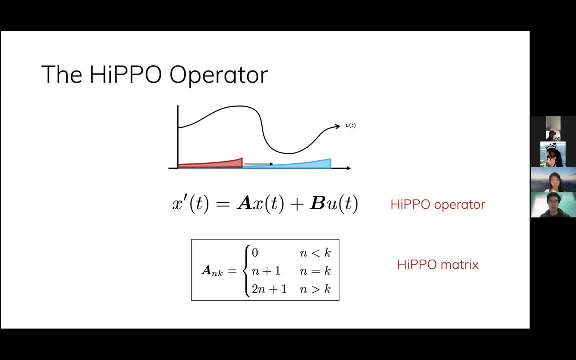 And the matrices- the matrix in the operator- are called hippo matrices, which have closed-form formulas. In fact, the actual matrix is this matrix. It's actually it's an extremely simple matrix, which is a special type of structure matrix. 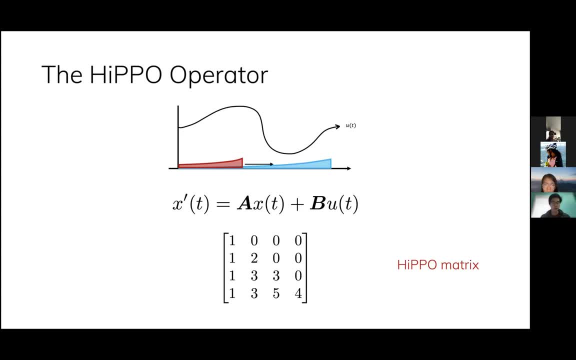 And yeah, so it's just a simple formula, And then we write down a closed-form formula for this differential equation And that's how our coefficients evolve over time And now right, so this equation again is called the hippo operator, or. 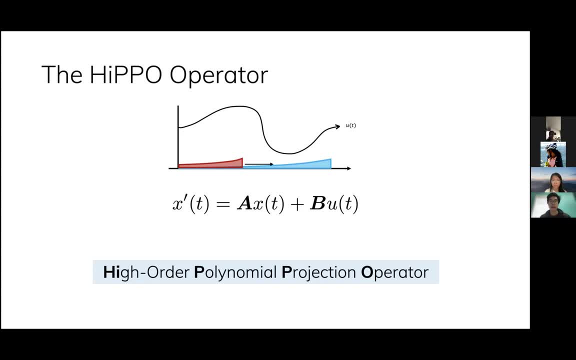 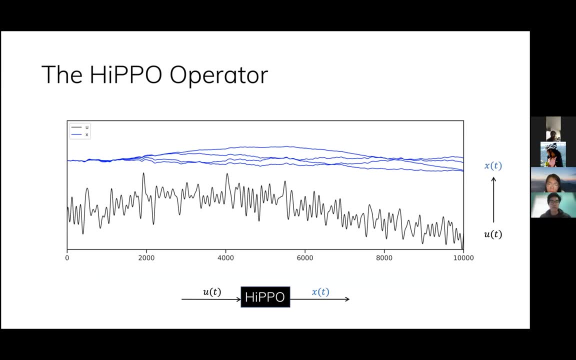 the high-order polynomial projection operator because we're projecting onto high-degree polynomial basis functions. Now, visually, the way to think about it is like this: The reason I call an operator is because it maps a function to a function, So it's an operator that maps. 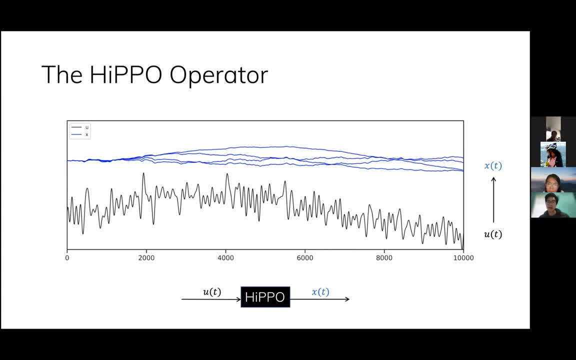 this black input signal u to these sets of coefficients, x in blue, where every time x of t compresses the history of the input. signal u And you can compute x online. as you see. u like one input at a time. So the black line represents: 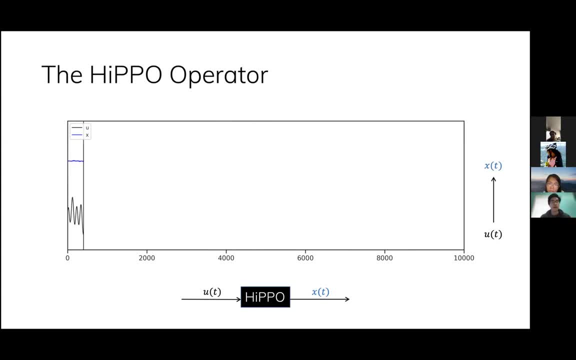 our current time step. We're gradually seeing more of the input And we're updating our coefficient vector, which is depicted in blue. Here I've. this is visualizing, visualizing just the lowest order: four coefficients of the best polynomial approximation. 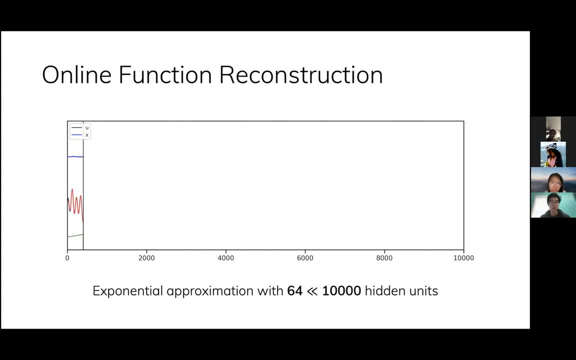 And and. now here is what the reconstruction looks like. So, as I move along through time and update my coefficients, the coefficients that that polynomial defines, in a sense, is actually just this red line. So it is reconstructing the input just like we wanted. 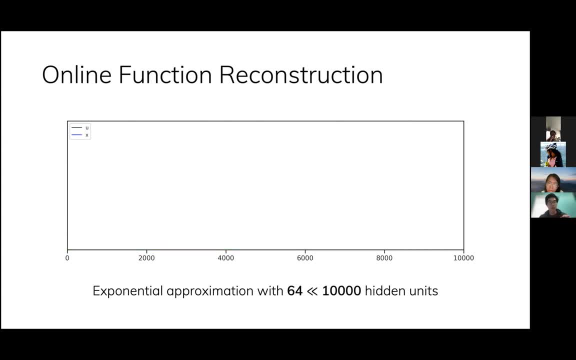 Note that we are using only so here I've only visualized four coefficients, but I'm actually using 64 coefficients, But the whole function was linked to 10,000.. So I'm compressing it a lot And this here's a static image that kind. 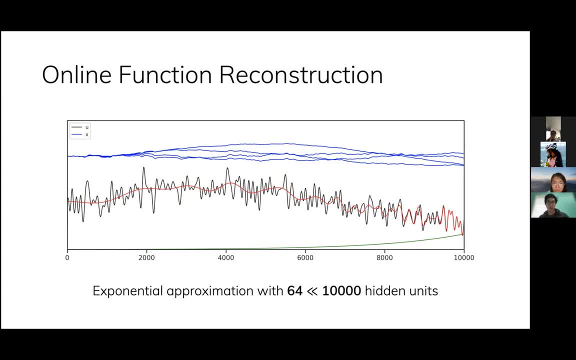 of illustrates the effect of the reconstruction. So because I'm compressing it, I can't perfectly reconstruct the input. And so how good is the reconstruction then? Well, it depends on the measure. So the green, the green line in this figure, 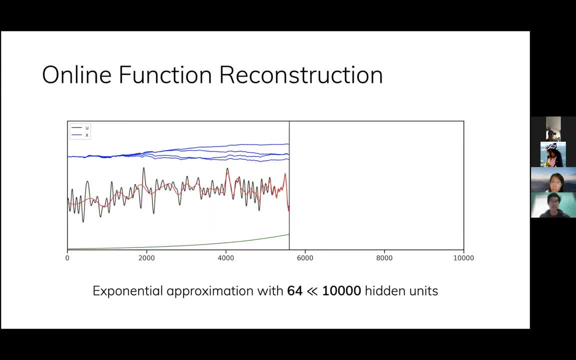 was the exponentially decaying measure that we are basically projecting onto And and so intuitively you can see that the red reconstruction line is really accurate for the recent past and degrades farther out in history, but still maintains some rough information about the whole signal. 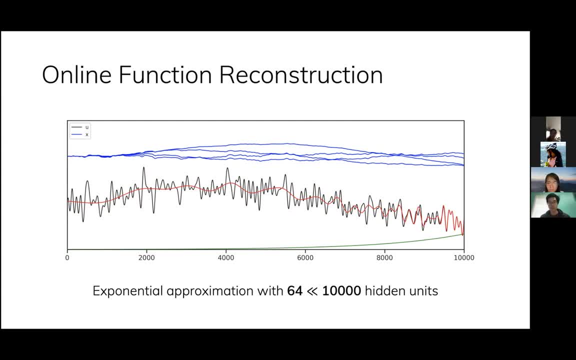 And so that is, that's HIPPO. Now, oh one one. oh okay, a question here. Oh no, you can continue. I just had one clarification, but I can ask after you finish. Here is fine too. 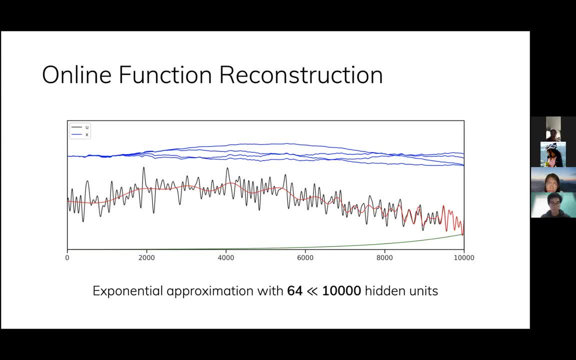 Oh, okay, So is it fair to think about X as being the state at each time point And then, essentially, the red line is trying to reconstruct the signal given the current state, or do you also use all the past states to reconstruct the current state? 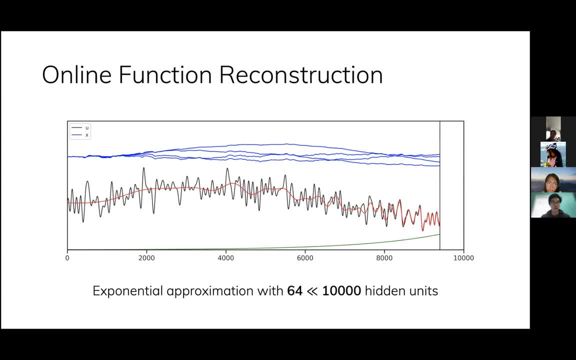 That's exactly right. So, yeah, so the reconstruction is happening using only the coefficient vector at the current black line. So every single time I'm using, I'm for, yeah, the blue line, I'm visualizing the whole thing, but at any given point in time, 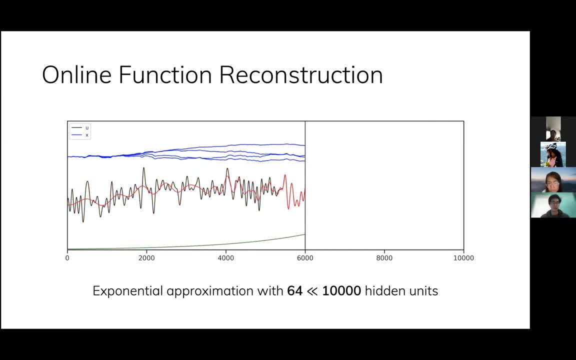 I'm remembering only the current vector, which has length 64.. Here I'm only visualizing four of the components, but it has length 64 and using those 64 numbers I'm reconstructing what I've seen so far in red. 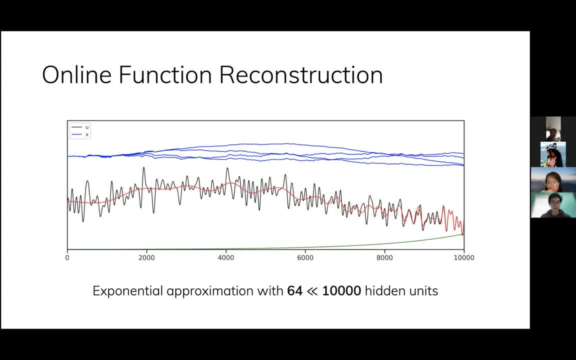 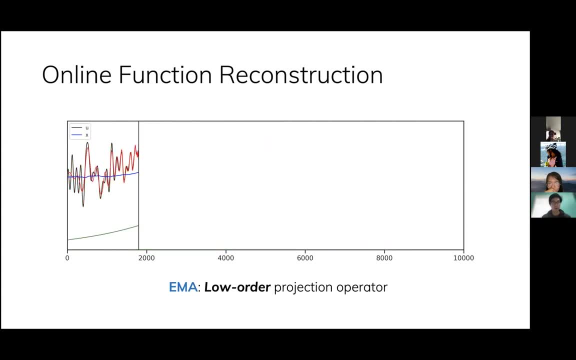 Oh, awesome thanks. Right now in that previous figure, if I just take one of the blue lines- actually the lowest order coefficient- and overlay over the function, you can see that it actually turns out to exactly be the EMA. So it turns out that moving averages can be viewed. 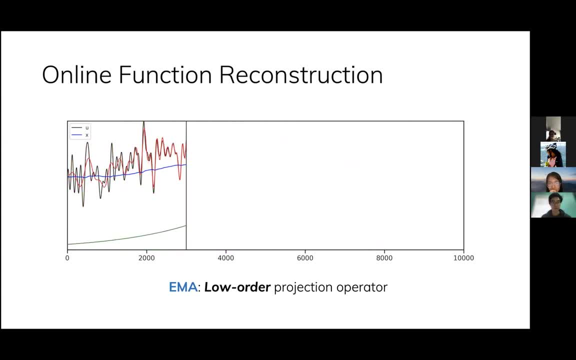 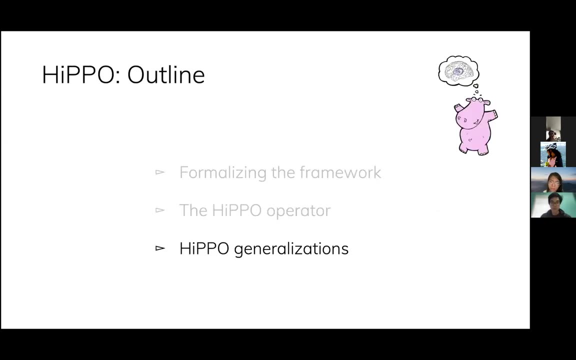 as order zero or low order projections. On the other hand, HIPPO is essentially a very strong generalization of this that solves a natural mathematical question and gets back things like the EMA for free. So that's what HIPPO is, And now I'll just talk a little bit. 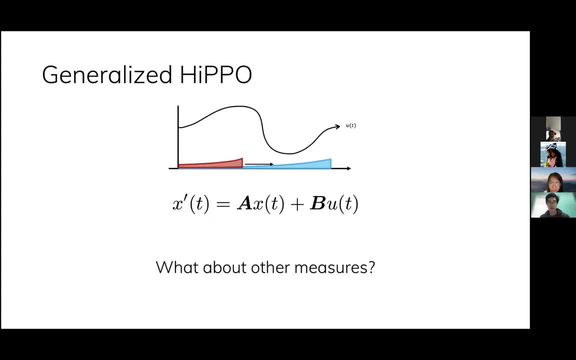 about some extensions of it. So, first of all, a natural question that may be wondering is that I've been using this example of an exponential measure. but what about other cases? Well, it turns out that HIPPO can be derived for any measure. 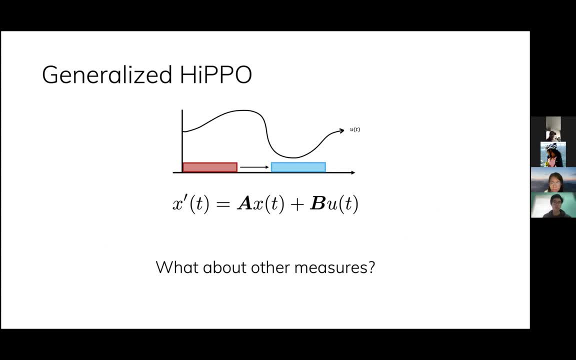 For example. here's a case that is pretty natural as well. which is what if I wanna reconstruct along a uniform measure? In other words, I only care about remembering the recent past in sliding windows of my function. And this is possible. And here is so you would get a different ODE. 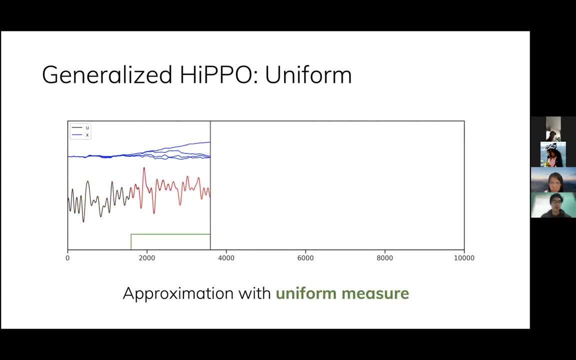 and here's a reconstruction in effect. So, again, using just 64 numbers in memory, I'm trying to reconstruct the last 2000 time steps of this function uniformly, and it's doing this quite accurately. Now you can generalize it even further to, for example: 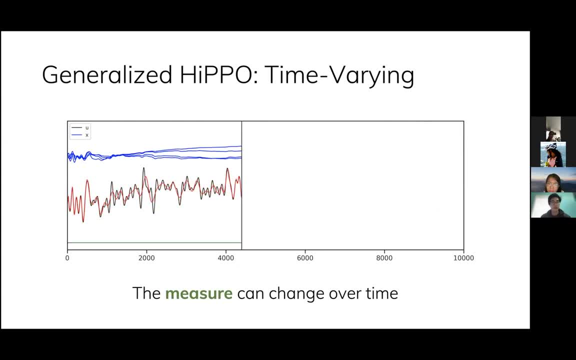 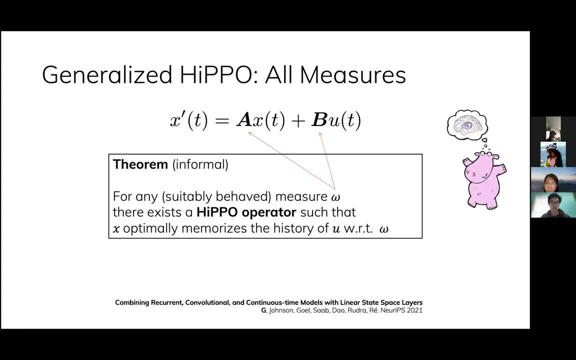 when the measure is changing over time instead of just sliding along, And so there's a very general framework here that can do lots of things. A lot of this was in follow-up work to the original HIPPO paper, And what we showed was that for any- essentially any- measure, 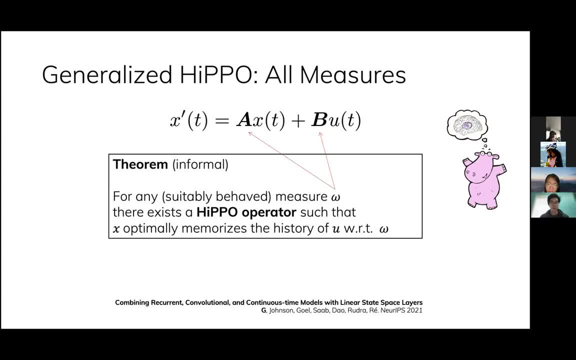 there exists a corresponding HIPPO operator where the HIPPO matrices A and B depend on the measure and you can write them down in close form. And this is important, I think, because it draws an equivalence between measures and these ODEs, where this means that we don't 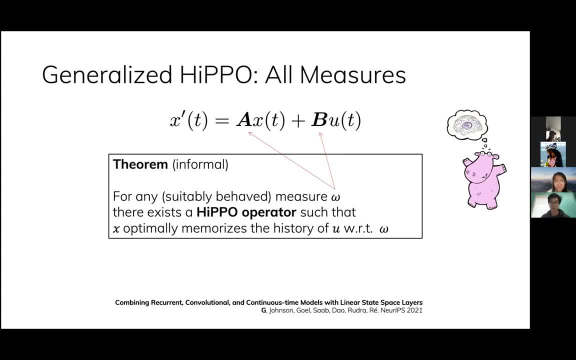 I mentioned earlier that we had to choose the measure upfront as a prior, such as the exponentially decaying case. but actually, just by learning these matrices A and B, it's in some sense the same as learning the measure. Okay, so now even better. 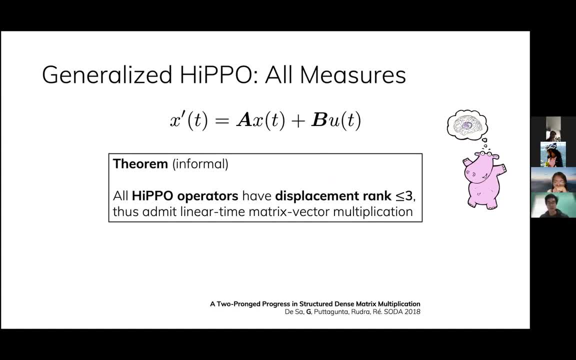 not only do these operators always exist, but it turns out that the matrices are always structured. So previously we saw for the exponentially decaying case, the matrix was actually extremely simple In general. they're going to be more complicated than that And they satisfy a structure. 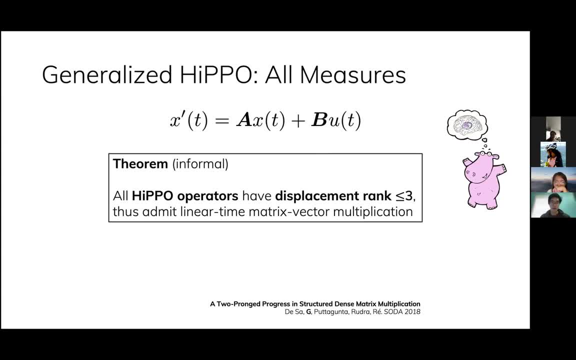 which was something that I introduced in much earlier work. but they are all structured in some way And that means that you can. how do you actually calculate this, these updates through time? You can actually update the state or the coefficients in nearly optimal time. 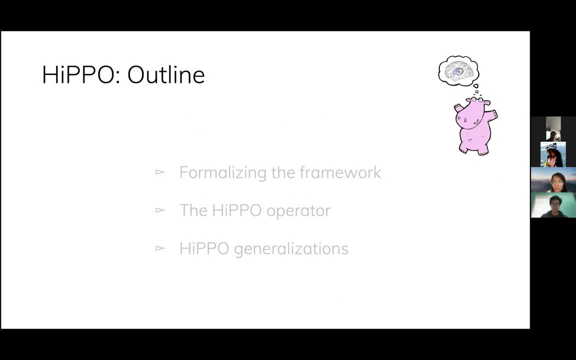 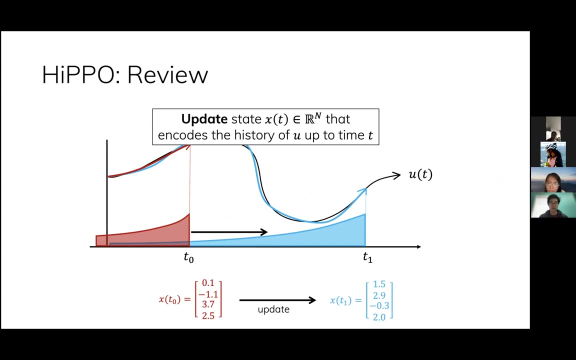 Okay, so that was the main takeaways from HIPPO, And so, just to recap, we were inspired by these very basic, these simple but important properties of trying to maintain a state- that's summarizing the entire context, And we formalized this into a mathematical problem. 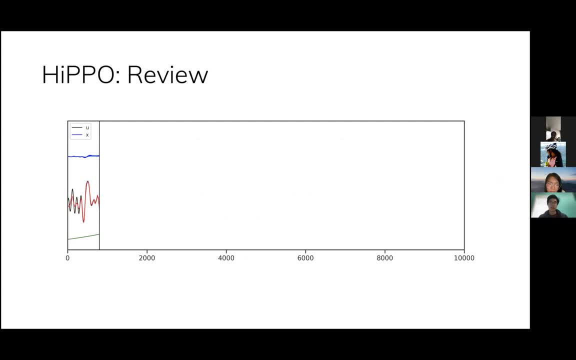 which was pretty intuitive, And we were then able to solve analytically, And this resulted in a nice class of methods for addressing long contexts and signals. Okay, so I see a question in the chat, So can these operators be expressed in terms of Z-transforms? 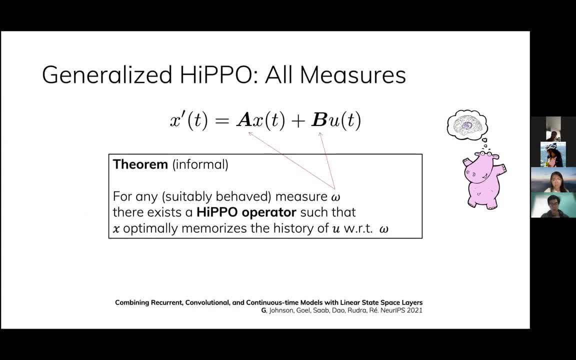 I'm not quite sure what you mean here. To my understanding, Z-transforms are like the discrete version of Laplace transform. I'm not sure if that's the one you're referring to or another notion. Yes, that's what I was thinking about. 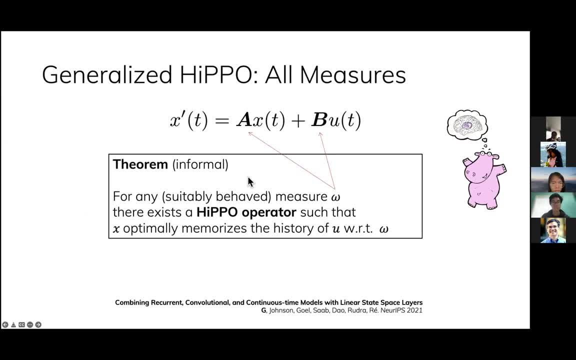 You know, it seems like, as though you know, just as you can express, like exponentially exponential decay in terms of Z-transforms of the functions, that there seems like there's likely to be a link. Yeah, I mean, I think all of these things 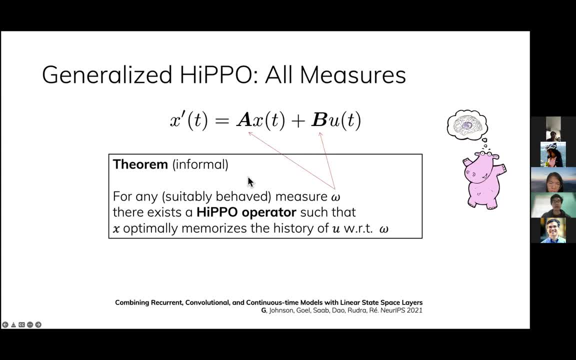 have a tight link and they're connected to each other. It turns out, actually, that the way that in the next part, when I talk about S4, there's going to be some difficult computational issues- that for computing certain things that I'll introduce, 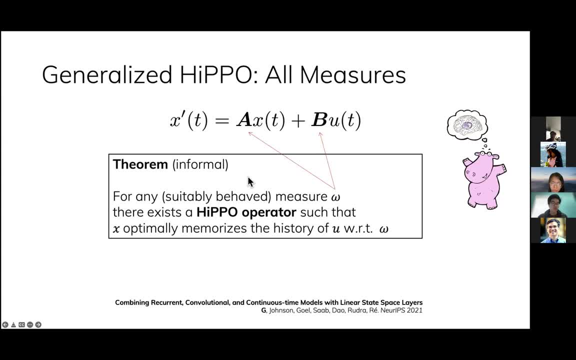 And to actually compute them I essentially actually go through Laplace space or frequency space. So essentially I actually take the Z transform of this equation and calculate that transform at several values and then invert it to get the hippo matrices back or to get a certain thing back. 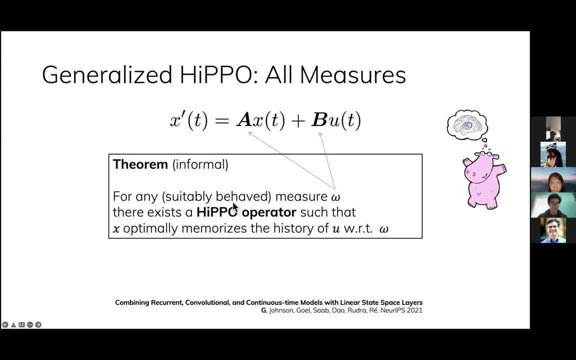 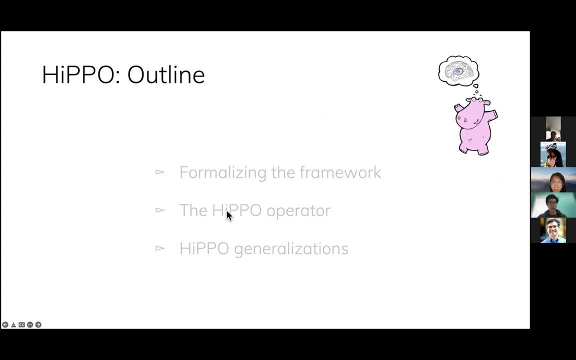 Sounds good. That makes sense to me. Yeah, Yeah, great question, And yeah, so I wanted also just to stop around here at the summary for any other questions, And if there's none, that's great, because usually this is a pretty complicated. 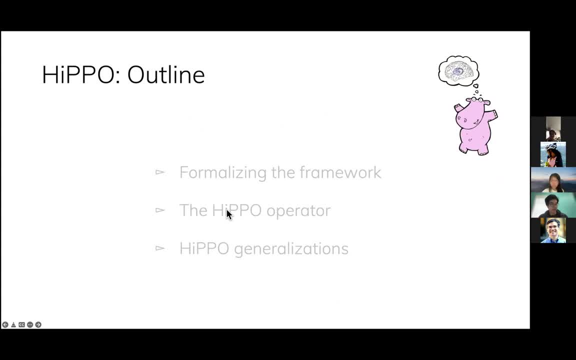 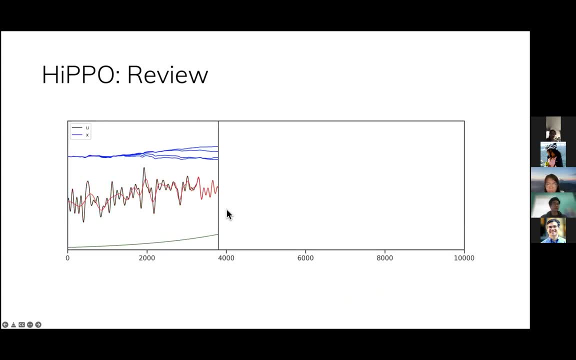 framework mathematically, but hopefully the visualizations help explain it a lot. Okay, So I'll move on to the next part, where so one thing I didn't include in this section was any experiments. So the way we evaluated this is kind of just like. 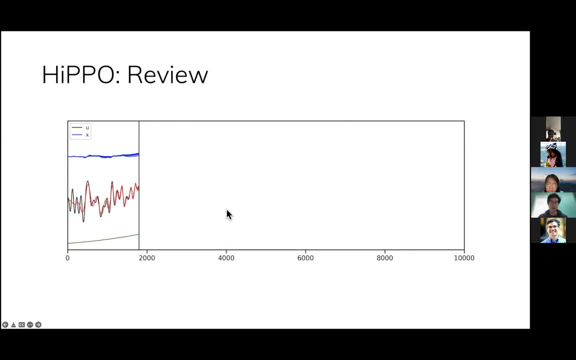 how good is the reconstruction? And actually using this method in machine learning models did pretty well. just naively, but where it became really effective was when incorporated into a model in a particular way, And so that's what S4 will be. And so to first I'm just going to define S4. 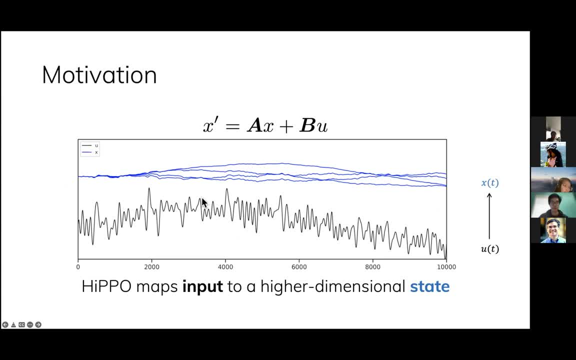 And I'm going to define it through HIPPO, which was the original motivation, And the motivation here is going to be very simple. So, to refresh your memory, this is what HIPPO does: It maps an input signal which, in our case, they're thinking of as 1D. 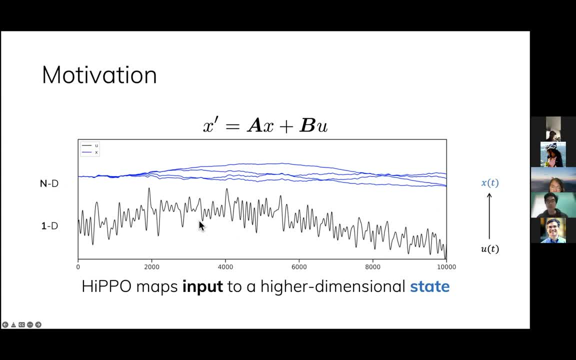 to a higher dimensional signal. Now the problem is that we've blown up the dimension of the input from one dimension to n dimensions, where n was our memory budget or the number of coefficients, And typically this is going to be at least 100 or so. 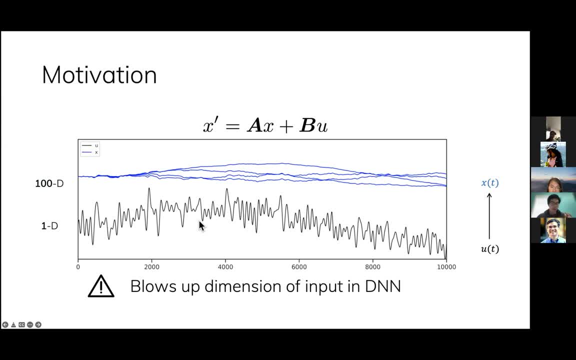 Okay, So the motivation for so? I work in deep learning and I just wanted to incorporate HIPPO into a deep learning model. But this is a problem because you can't just stack layers of this, because you just keep increasing the dimension, And so a very simple motivation to fix this is just: 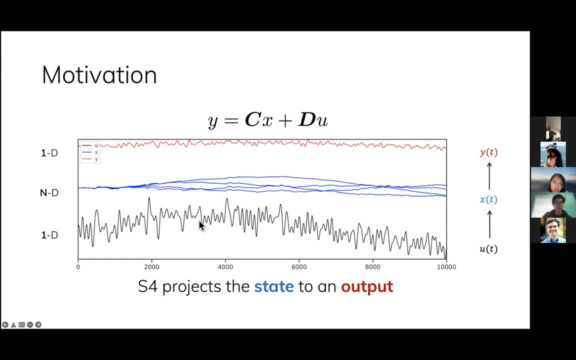 let's just decrease the dimension again, And the way to do this is that you can just take a very simple linear projection. So what we'll do is that we have a state X, which was like a hundred dimensional vector, and we'll just hit it with a dot product. 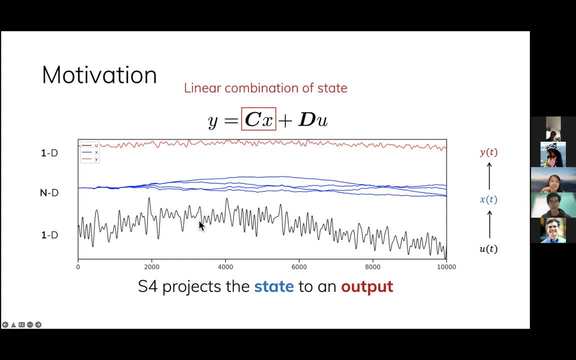 that can be learnable- to get back a single number, which is essentially taking a linear combination of the blue lines to get the final output, which is the red line, And then we'll add a multiple of the original input, which can be seen as a skip connection. 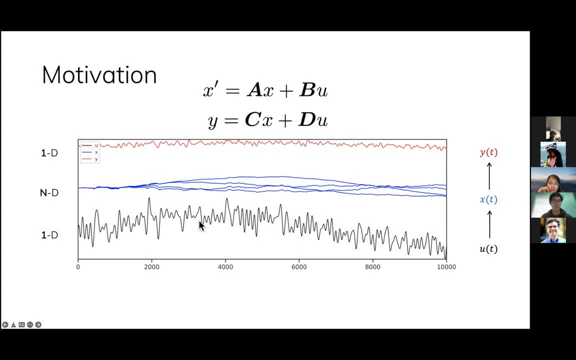 And that is the entire definition of S4.. It's finally these two equations where the first one is the HIPPO equation, which takes the input to a state, that's kind of memorizing it, And then the second equation just combines the state linearly. 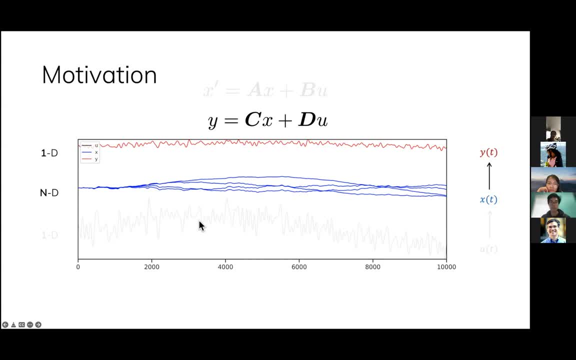 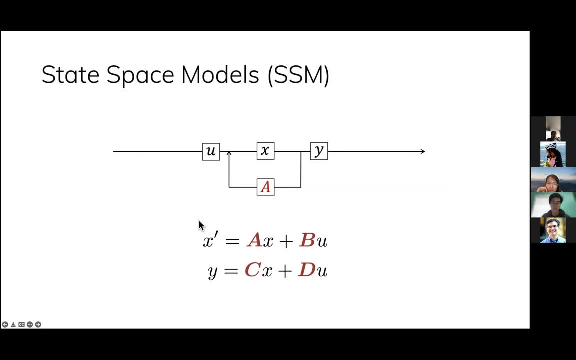 linearly back into a single output. Now, for those of you with a background in engineering, this definition may look really familiar, And this is because this is a well-known model called a state space model, or SSM, which is sometimes depicted with this simple control diagram. 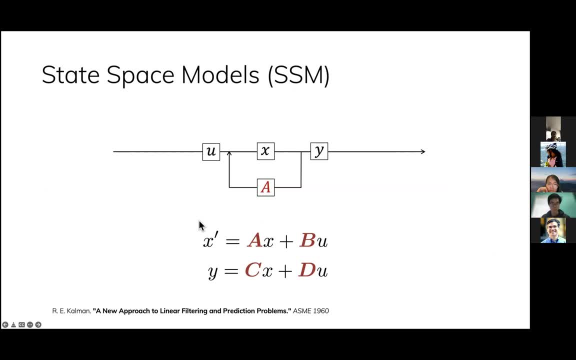 And they've been around for decades, such as the famous Kalman filter, and use in many scientific fields. I think, outside of controls and statistics, they're also pretty commonly used in, perhaps, computational neuroscience and in many medical problems as well. Now, what the theme of this part will be is that we'll see that 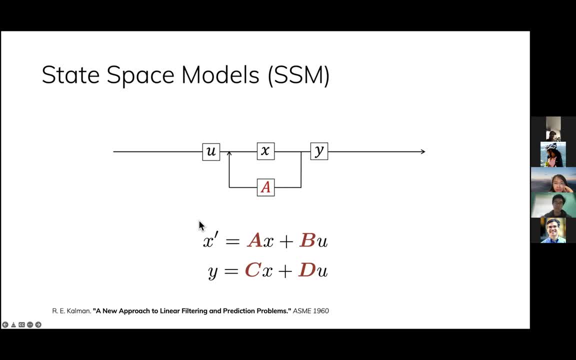 SSMs are a really elegant and natural model, but they haven't been used in deep learning before in this way And for underlying reasons that we'll see and that S4 will address. But for now just to define S4 in terms of this model. 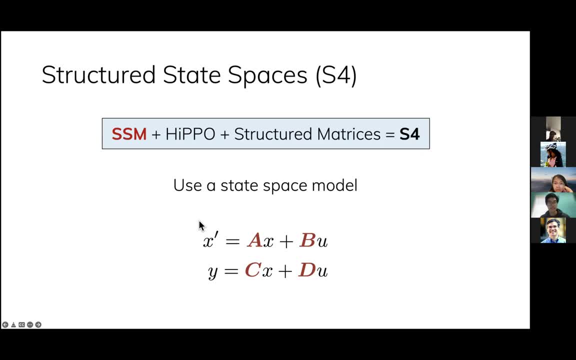 the way that we will define it is that it's just an instantiation of an SSM, these two equations where we'll plug in specific values of matrices in, and, although it turns out that, although this model is simple to define, actually computing with 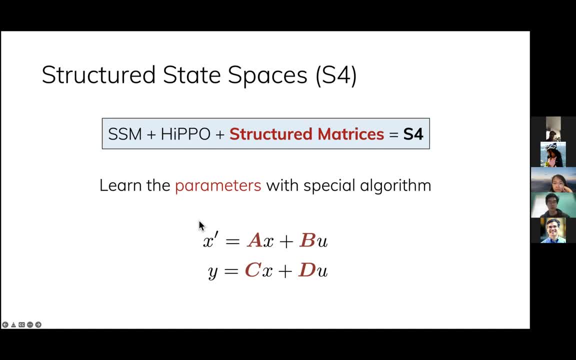 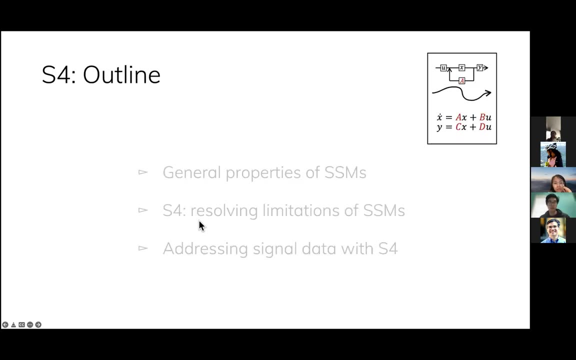 it turns out to be difficult and will require new ideas and algorithms, And so my goal of this in this section, is to convince you that this is a really elegant and fundamental model, And so, first of all, I will talk about some general 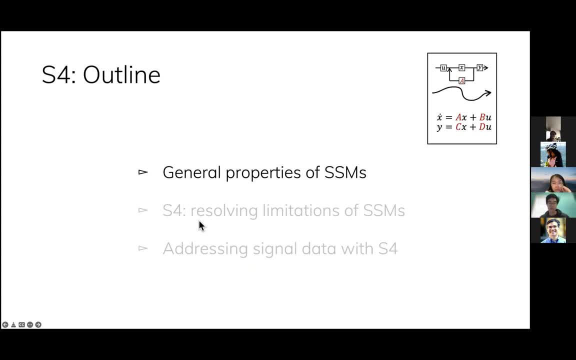 more properties of SSMs that would have a lot of benefits in machine learning and deep learning that are independent of S4. And then I'll show how those come with associated trade-offs that prevent them from being really good in deep learning, And S4 will solve those problems. 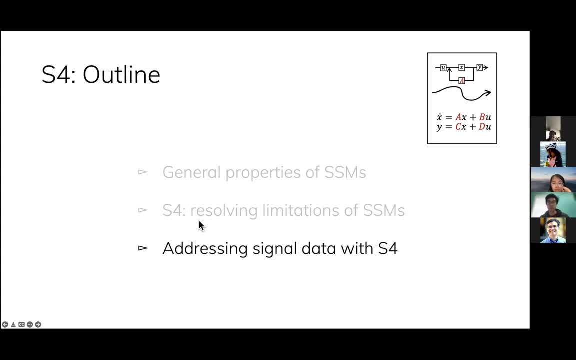 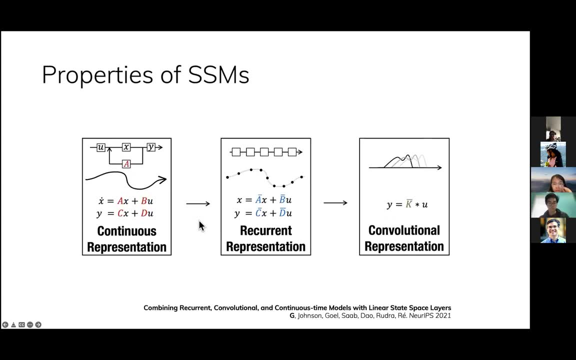 And finally I'll show several real world experiments that show S4's effectiveness in a bunch of settings. So in this first part I'm actually going to describe three different ways to think about SSMs, which give them a lot of nice properties. 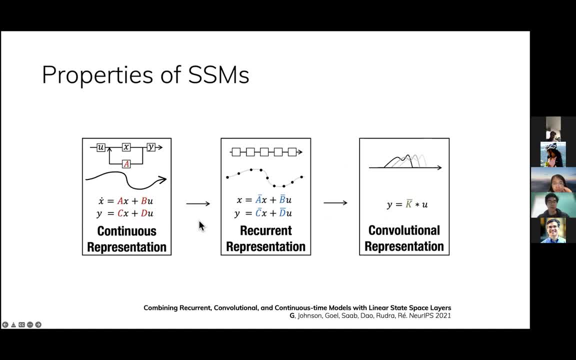 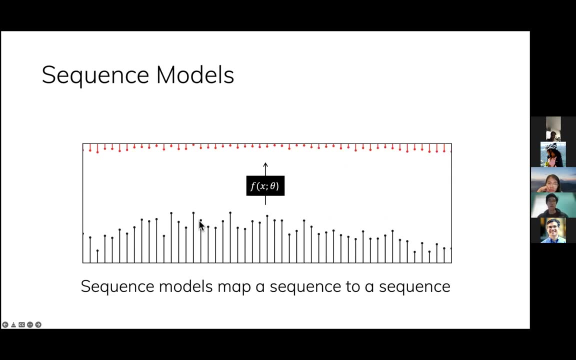 And this was theory developed in the predecessor work to S4- that and will have empirical, concrete, empirical benefits. And so the first way to the first property is that SSMs inherently operate on continuous time signals instead of discrete time sequences. So here's how to think about it. 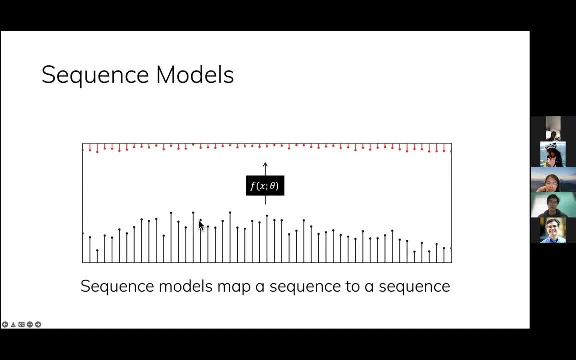 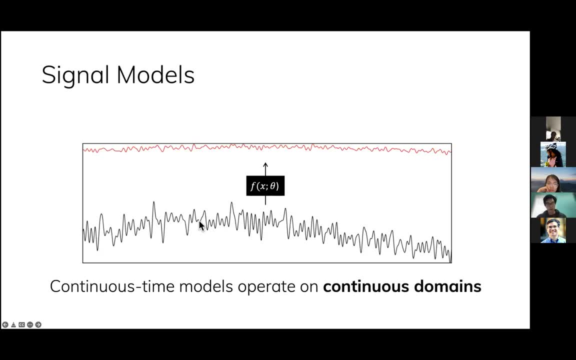 So in machine learning, we usually work with sequence models, which I defined as a parametrized map from an input sequence to an output sequence. Now, what if, instead of mapping a sequence to a sequence, I coined this term signal model to denote a parametrized map that maps a? 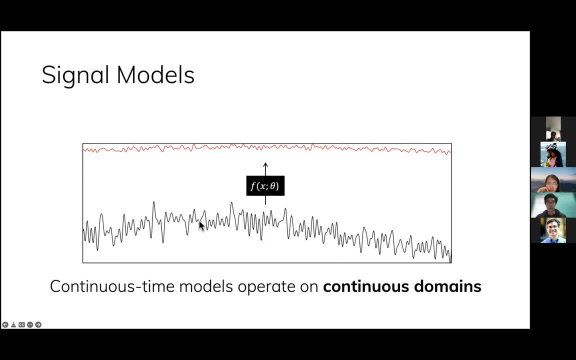 function to a function or a signal to a signal, And, given one of these maps, you can essentially discretize the inputs and outputs however you want to get back a sequence. So essentially, the upshot is that signal models are in some sense a generalization of sequence models. 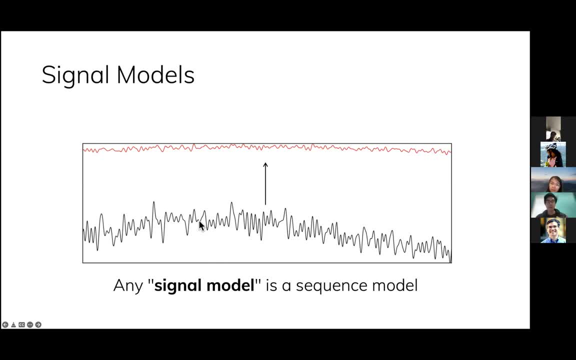 where they actually map functions to functions, but by discretizing them you get back a sequence model, And so the first way to think about SSMs is that they are just a simple parametrized signal model, where the parameters were matrices A, B, C and D. 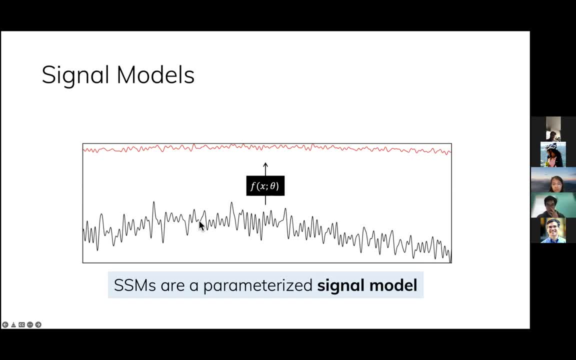 and they map an input function to an output function. That's it Just in terms of the interface or the API of the model that this is what it does. The reason that this property is important is because, even when we're working in discrete time, 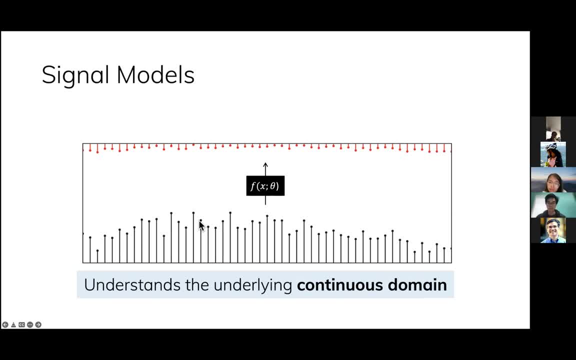 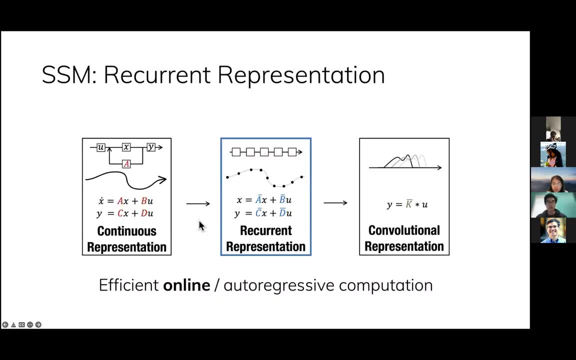 the model in some sense understands the underlying continuous domain. So I will show what I mean completely by this later. empirically All right. So that's the first representation. The next perspective relates back to the original motivation of HIPPO, which was about online computation. 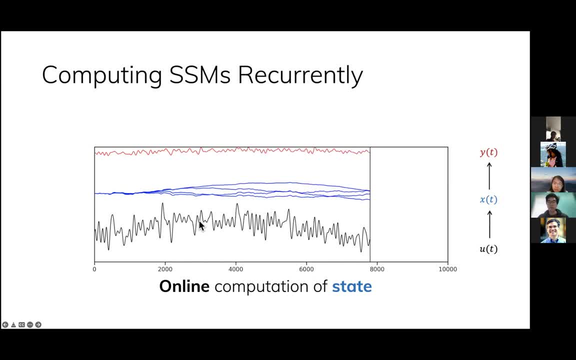 So how do we actually compute the output of this SSM? One way to do it is to process the input one at a time, just like HIPPO did, in an online setting, And so this is a recurrent computation, because each, each update can be computed efficiently from the previous one. 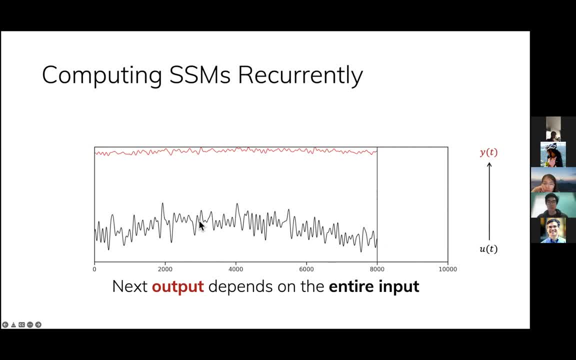 And just to unpack a little why this is non-trivial: Imagine we're processing this very long input and we're, at this current time, step denoted by the vertical line, and we get just one more data point. So just like a single number for the input. 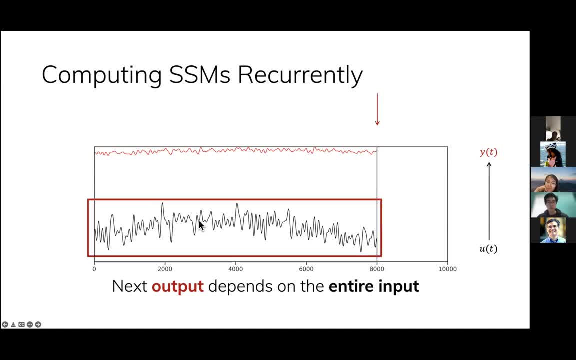 and we want to compute the next output. So this output depends on the entire history of the input, And so you'd expect it- the computation of the next one- to scale with the length of the sequence. But actually we can compute it in constant time. 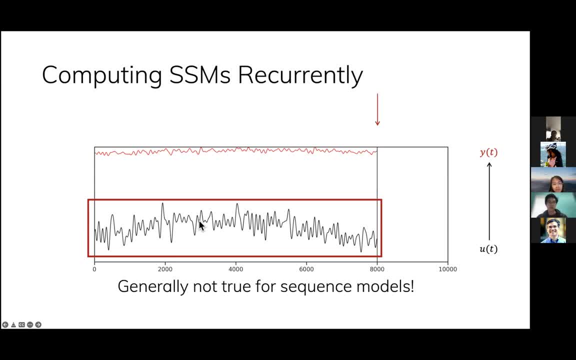 And this is a non-trivial property that most sequence models don't have, For example, in a transformer or a convolution. if you were to do this in an online or autoregressive fashion- computing mapping one input to one output- each computation will scale with the entire length of the context window. 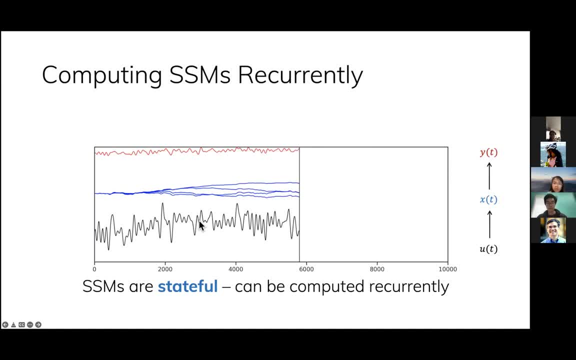 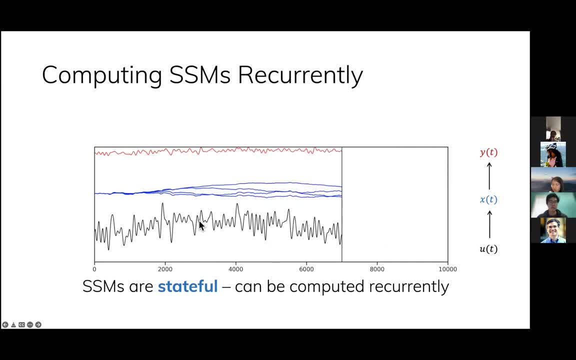 which is a single vector that's summarizing the history and can be updated very efficiently. This makes them really efficient in any sort of online setting, as we've seen, And yeah, so we'll see again why this matters. But there's one main drawback. 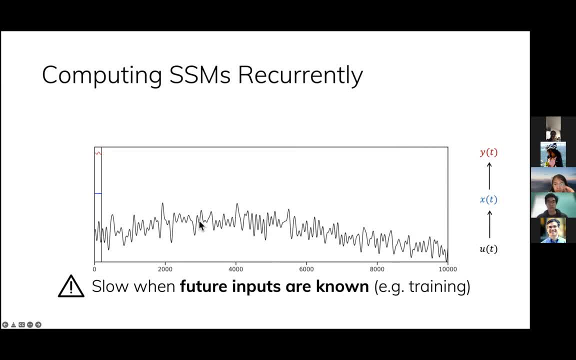 which is that if they're not in an online setting, this is slow because it's sequential. And so what? if you actually know all the future inputs, Then ideally you wouldn't do this step-by-step and you could do something faster and parallelizable. 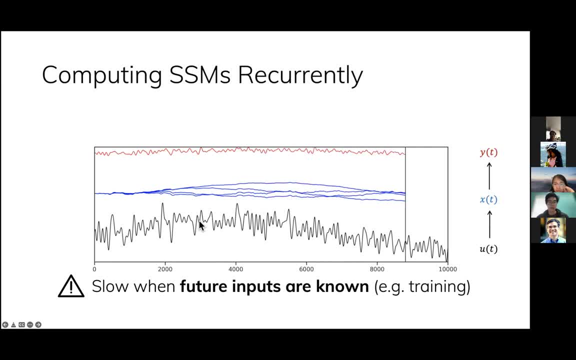 And so that was actually basically the main problem with RNNs and why they've recently fallen out of favor in machine learning, because they're sequential and not parallelizable when you see a lot of data at once, And so that motivates the final representation. 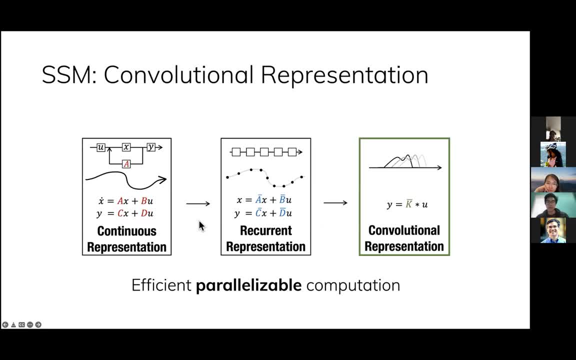 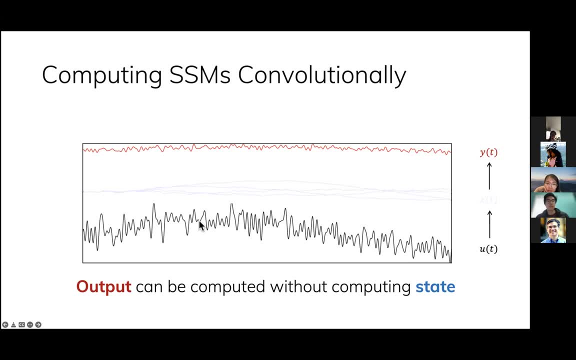 which is the convolutional representation which allows them to be parallelized, And so the idea is that, instead of mapping going from the input to the state to the output, you can actually go straight from the input to the output, bypassing the state. 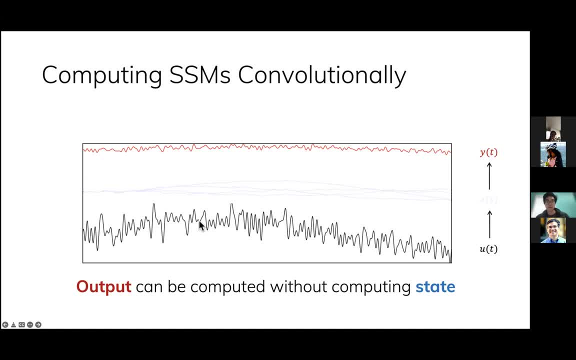 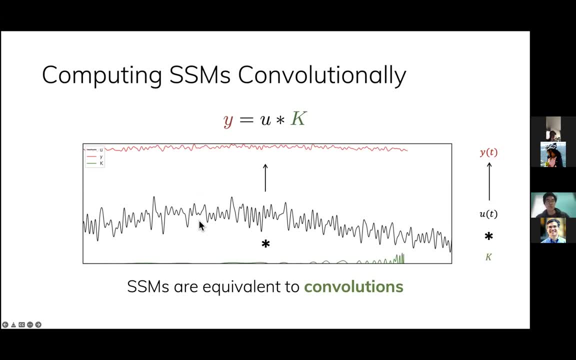 and doing the entire computation in parallel over the sequence length. The reason is that SSMs turn out to be equivalent to convolutions, where computing the map from the input u to the output y is equivalent to convolving the input by a particular convolution filter. 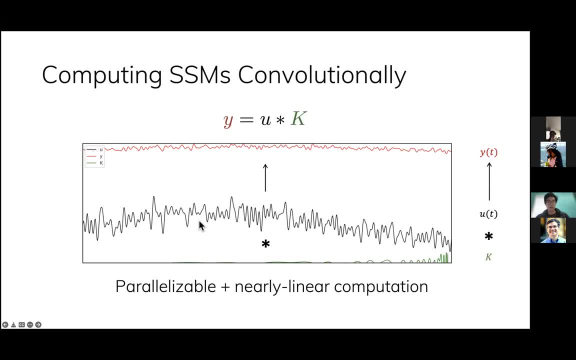 which is depicted in green here, And so to compute this map, it's just: y equals u, convolved with k for this convolution kernel, And so this can be done very efficiently using known techniques. So, for the practitioner, one thing I want to emphasize is that 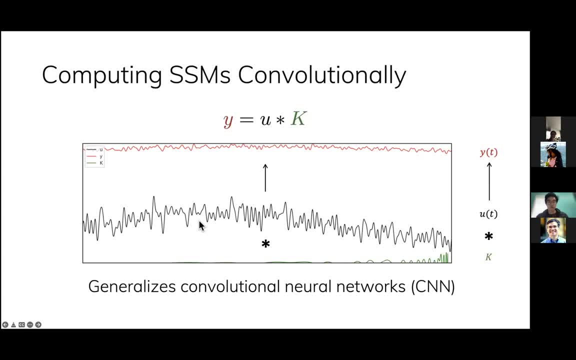 I think the most useful way to think about SSMs potentially is as essentially a very fancy CNN, where you're parametrizing the convolution kernel in a different way And, um, notably, this kernel can be infinitely long. 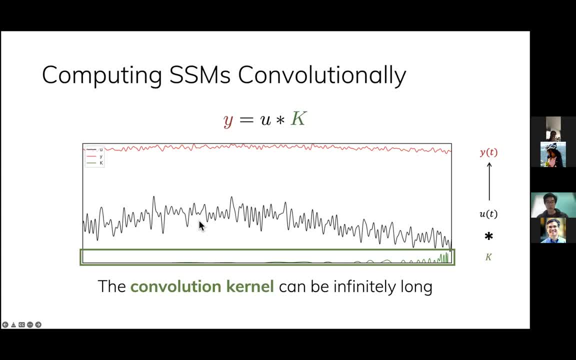 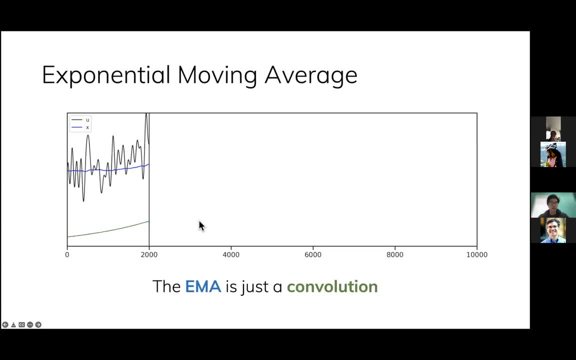 which again points to one reason why this is very good at long-range dependencies. Um so, just to call back to this example again, the EMA. the EMA is actually literally just a single convolution where you convolve the input by an exponentially decaying convolution kernel. 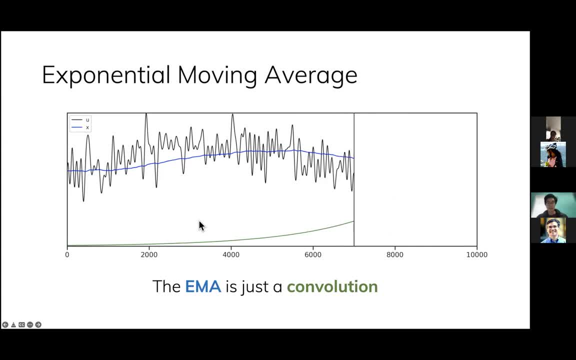 And, as I mentioned, although things like CNNs are also literally convolutions, they can't represent the EMA, because CNNs are finite window and the EMA is infinite window. On the other hand, SSMs do represent infinitely long convolutions. 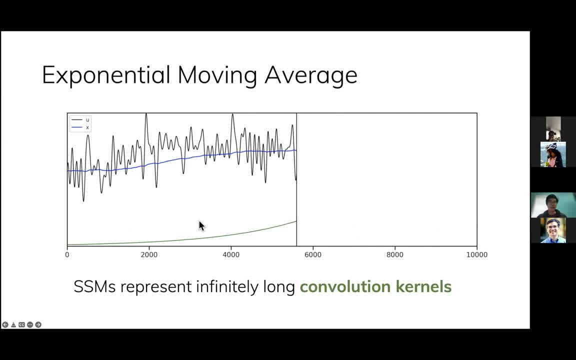 And in fact there's a very, very simple way to write down the EMA as a directly as an SSM, And I think Chris kind of pointed to that earlier. Um, so that's, those were the three properties of SSMs that I wanted to mention. 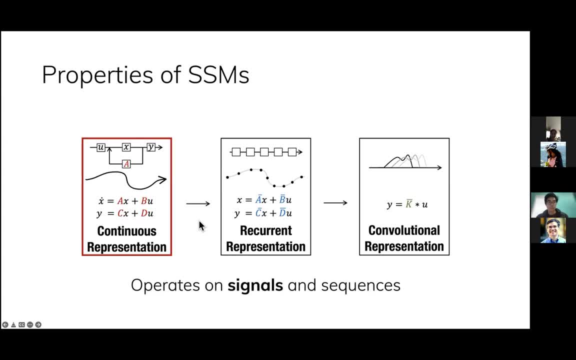 Um, and just to recap, first of all, we're going to think of them as maps that operate on continuous signals, not just sequences. if your model is deployed in a setting where it sees inputs in real-time or online, it can compute these efficiently. 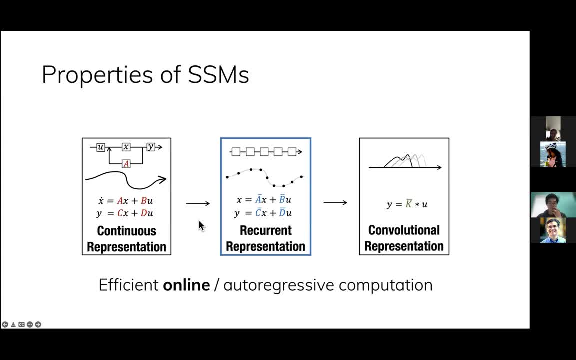 um, uh, recurrently. And if you see an entire input at once, such as usually during training time, you can compute it even more efficiently and in parallel. Um, I have a quick question here, Albert. Um, this is super cool. 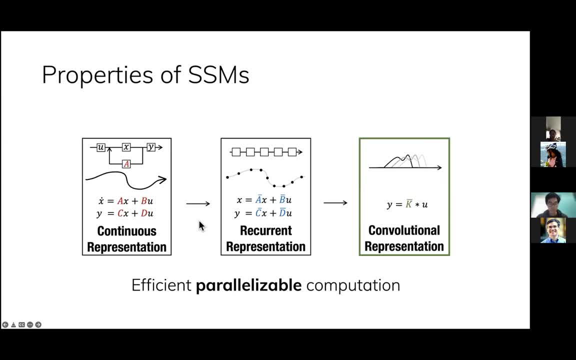 Um, I was just wondering if, if the goal is actually to get a representation of your signal so that you can perform different downstream tasks, isn't it better to actually have the state space representation rather than directly going to the outputs? in that case, 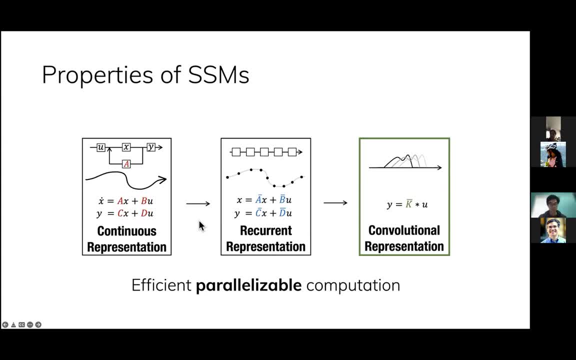 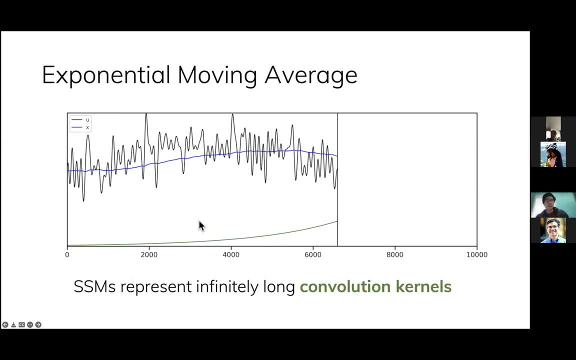 would we have to stick with HIPPO instead of going to S4?? Great, great question. Um. actually, no one's asked me that, but that's a great question. Um, so the way that I think about this is that um. 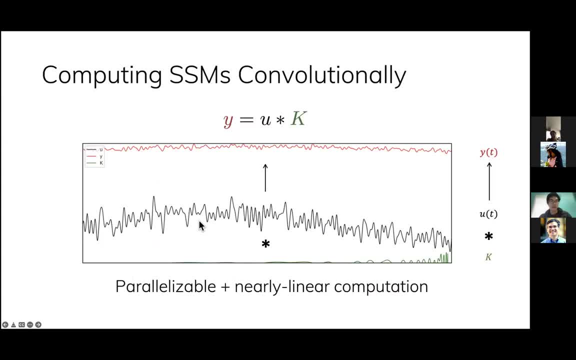 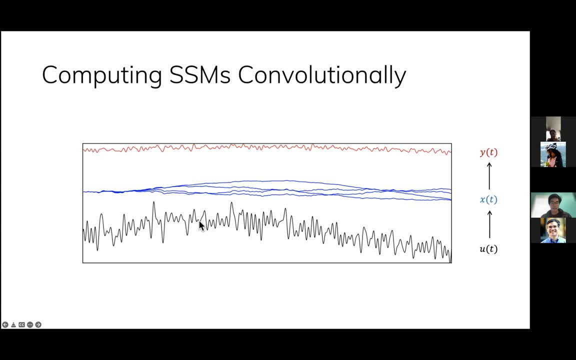 the what's happening is that, uh. so essentially we have this like this nice, uh, this nice state, which is very meaningful, And then the, the second part of the SSM that projects. it is kind of like the learnable thing. 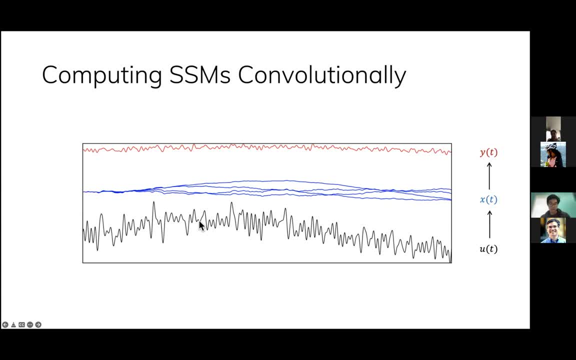 That's figuring out how to extract the right features from this state. Now, I mentioned that everything I've done so far, So so that's a learnable part That's actually using the entire state in a sense. Um, and I mentioned that I've only 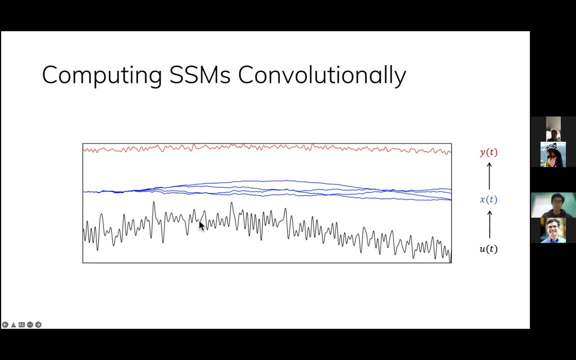 I'm only considering the one dimensional case so far, with one: the inputs and outputs, Um, but actually what's going to happen in practice? in our uh, our actual deep learning models? we're going to have multidimensional inputs and outputs. 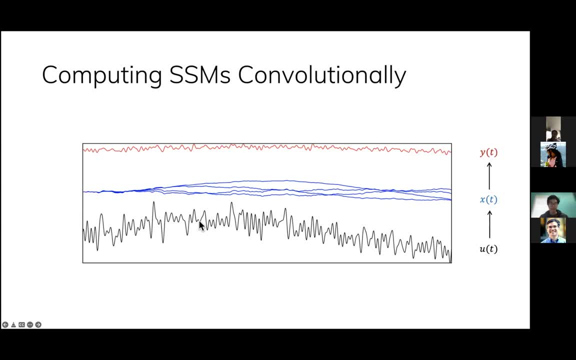 And um, we'll essentially run an SSM on each one of them And each one of these will learn how to use the state in a different way. So this, so we'll have essentially men w, w you can think of as like. 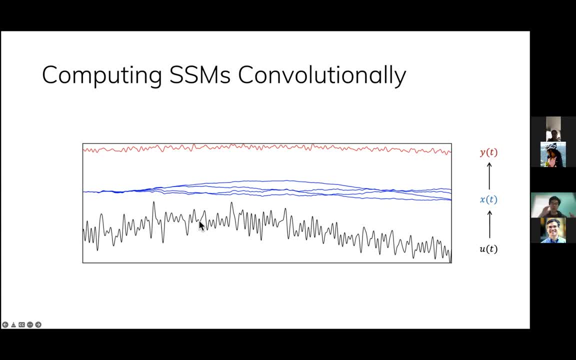 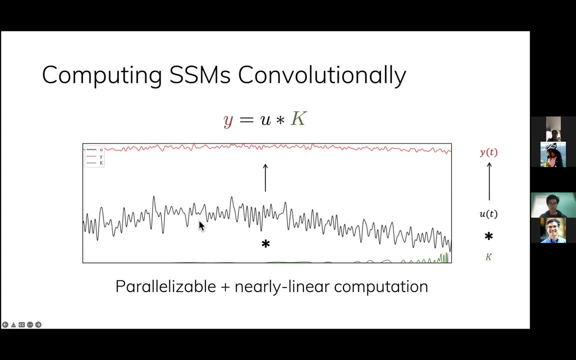 maybe we'll have many. we'll have like a single state, but many, many possible outputs that are all learnable and we'll extract different features from that state. So we are going to get a lot of different features that utilize the state in however they want. 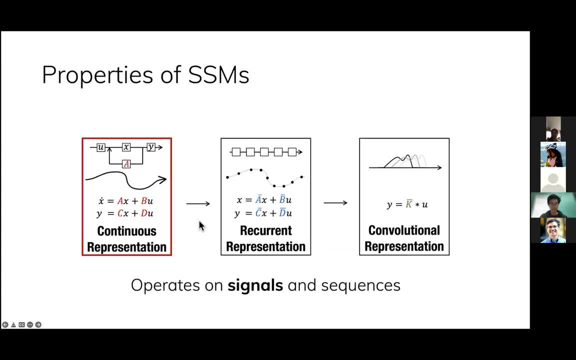 I see, Okay, Thank you, Sorry. Sorry, John led. uh, isn't it like all these dimensions are also have um correlation? So do you also? if you run the space independently, don't you want to also preserve the correlation? 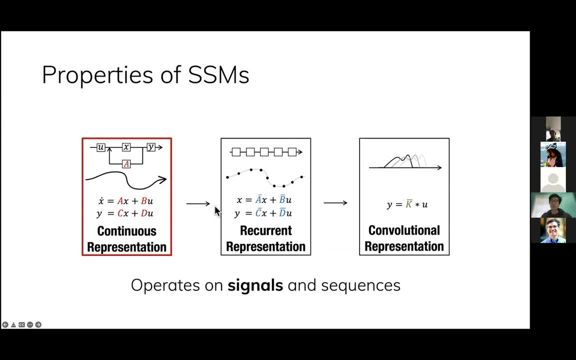 So this is something that I think a lot of people working with time series um are concerned with, and somehow in deep learning we don't normally consider that aspect and we kind of just throw in a really big model and a lot of these independent layers. 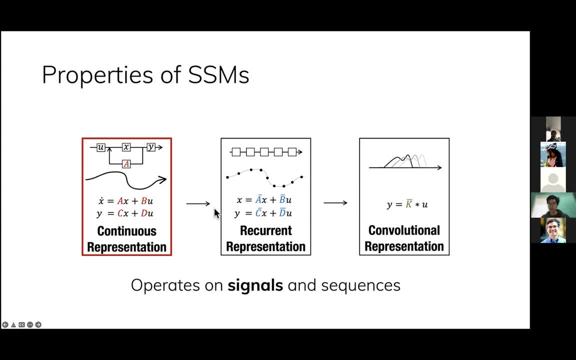 And um kind of, I think, in practice. I think that's a really good example of how the model learns to. it learns whatever it needs to do for the final prediction task, And um, this often does involve like. 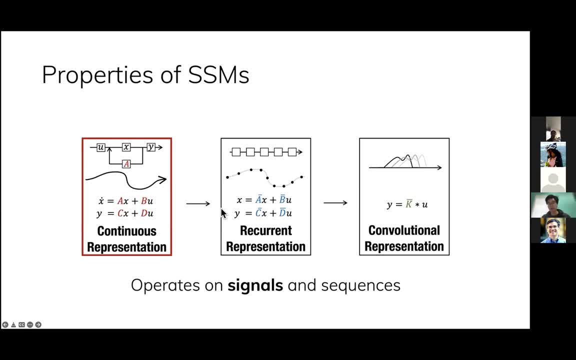 I think it does end up decorrelating things. but, um, it's not super clear exactly the dynamics of what happens, And this is kind of a more broad question for deep learning theory in general, That's, that's not well understood right now. 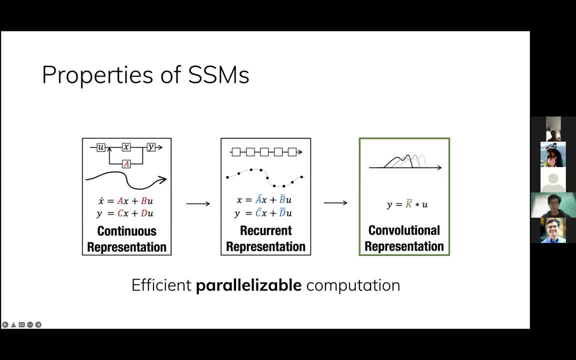 Um, what I can say is that, um we've used this on um many types of like noisy data That usually involve um we can do it on multiple dimensions, or maybe it's one dimension That's easy. d as one dimension. 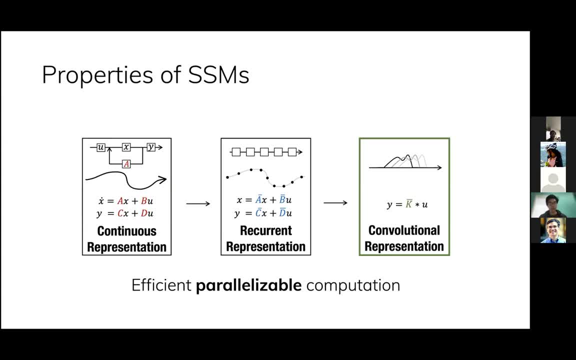 And we can do this on multiple dimensions later. but w? w, we have tried this on many types of like time series and other noisy data like EEG, But it can Right. Uh, well, it can work on multiple dimensions um, which I kind of just pointed to. 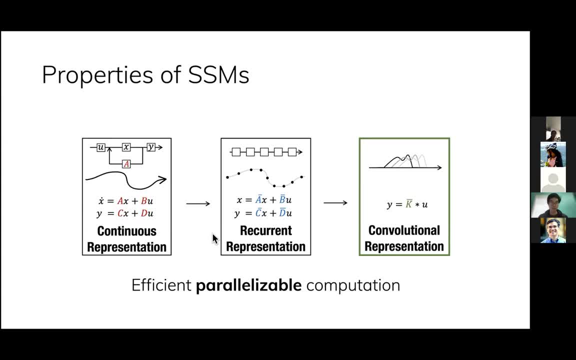 and also I'll- I'll mention again later how we do that- Um, um. but yeah, you can just kind of do it, Do it naively on multiple dimensions and it and it just works out of the box, Okay. 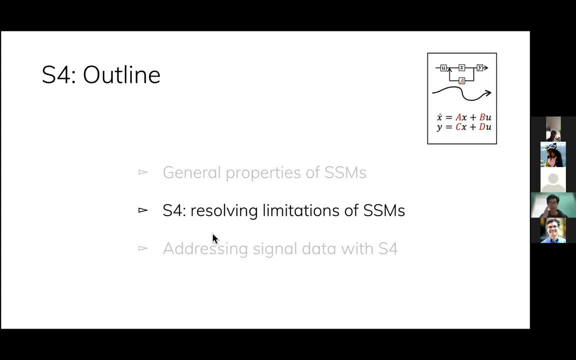 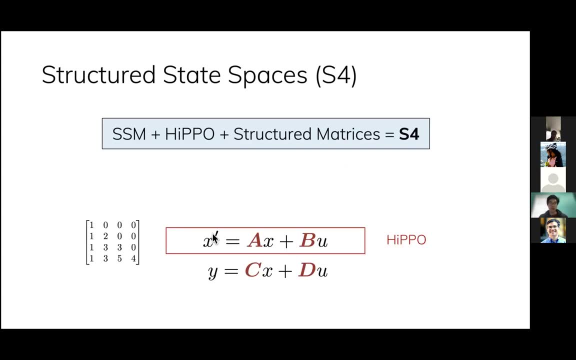 how S4 builds on top of SSMs, And so just to refresh your memory of what S4 is, it's just an SSM where we plug in certain formulas that were based on the theory of memorization and we have special algorithms to compute it. 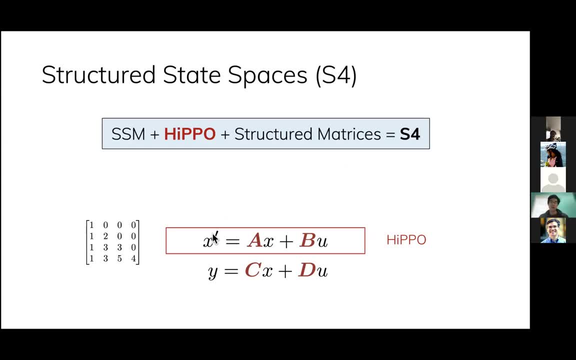 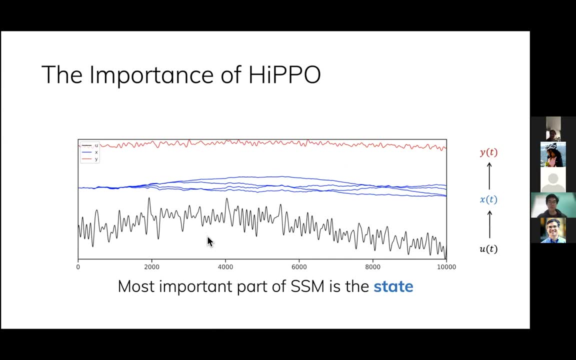 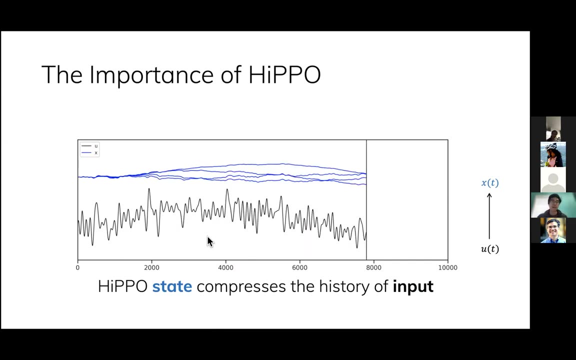 And so, first of all, why are these matrices needed? Well, the most important part of the SSM is the state, as Nandita keeps insightfully bringing up, And so what HIPPO does is essentially what HIPPO did- was that it computed a very particular state. 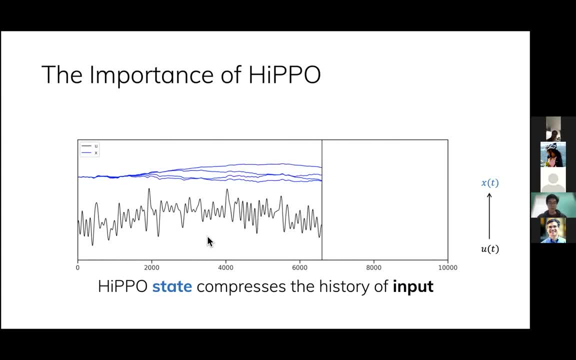 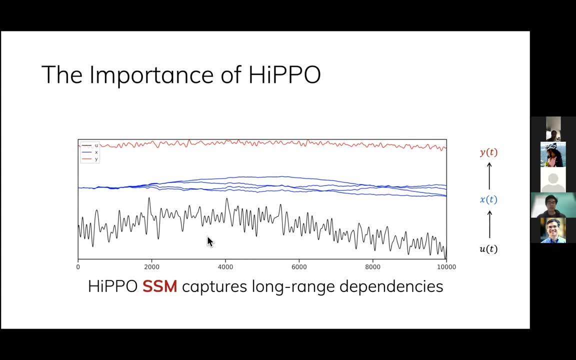 that was mathematically meaningful and compresses the history of the input in a way that captures long range dependencies. And so, basically, just by plugging in that formula into this SSM, it learns a more meaningful state that allows the SSM to address long dependencies better. 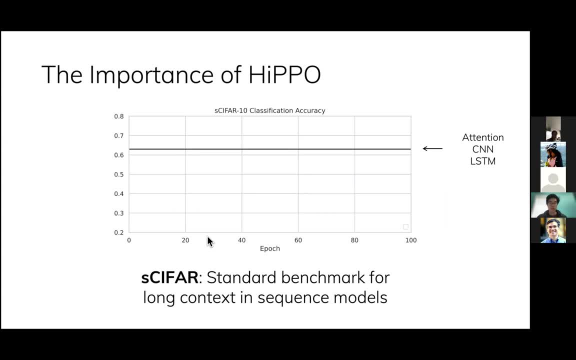 So just to illustrate this empirically, here's a simple experiment on a very standard benchmark for sequence models. The actual task doesn't matter, but it's well-studied and standard sequence model based, such as transformers, CNNs and LSTMs all get to around the same accuracy. 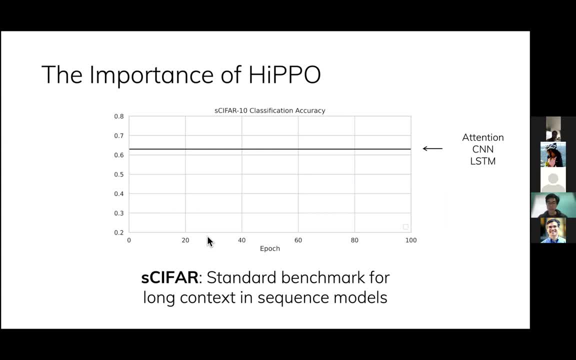 of like 60-ish percent. Now what happens if we use an SSM? If you use it naively by randomly initializing all the parameters, which is what you would typically do in deep learning, it actually does terribly. But what happens if we just plug in this formula? 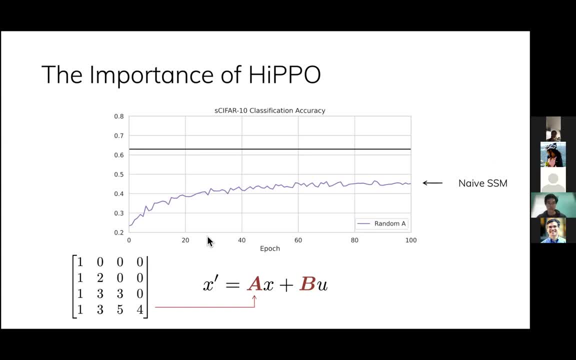 Plugging this in and not even needing to translate it. it's not going to be able to do that. It's going to be able to train. the matrix gives a massive boost to the SSM and goes from much below the baselines to substantially above the baselines. 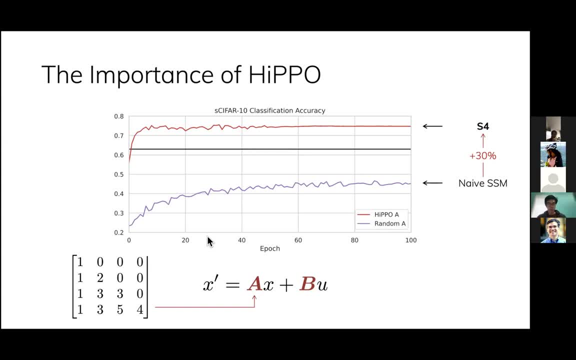 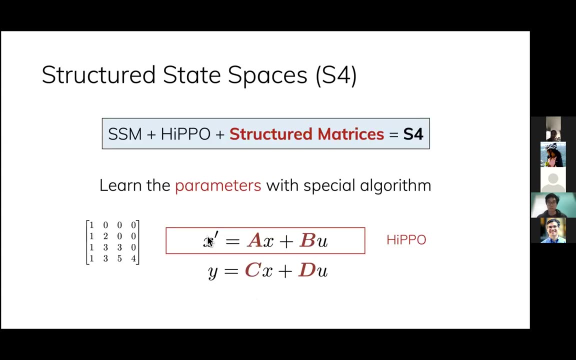 And actually I use the very small models for this ablation here. but the full model as far on this dataset gets over 90%, which is something like 20 plus points better than all of the other C++ models. So that kind of illustrates why HIPPO is so useful. 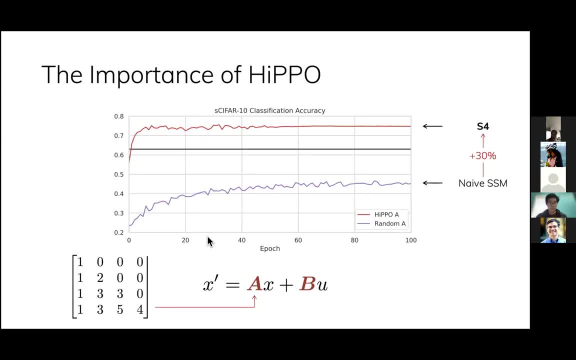 Now the second- A quick question in this example, So are both A and B basically just plug-in matrices or is A alone basically a measure? A is the more important matrix, but actually, yeah, just plugging in A and B, essentially just they're both fixed matrices. 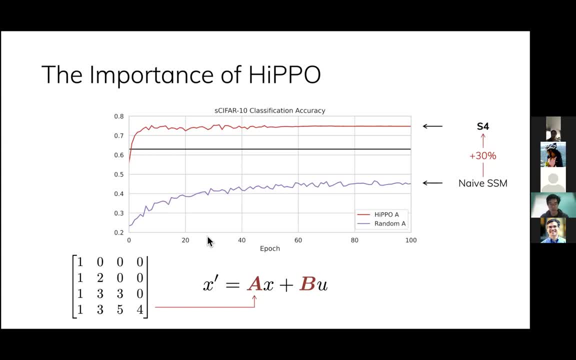 which are the HIPPO operator specifies both of these. I've only illustrated A because it's the more important one, but yeah, this particular experiment froze both of these matrices to specific models. Got it okay, thank you? Yeah, one question people have is that like 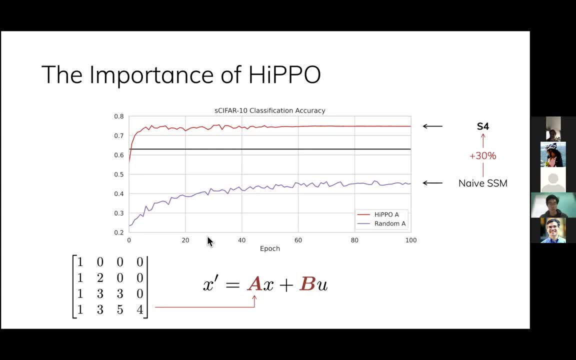 do we always freeze these And actually we can train them as well. This was to illustrate just like even freezing them it does super well And then. but in practice we do train them and it makes it do a little bit better. 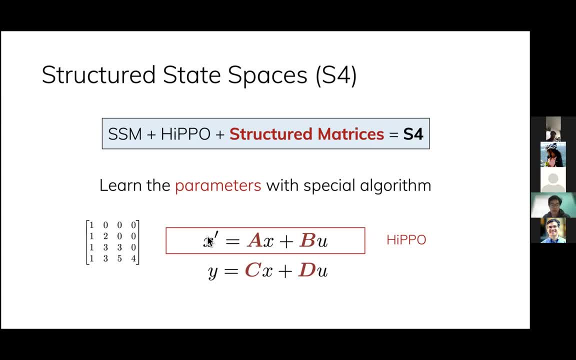 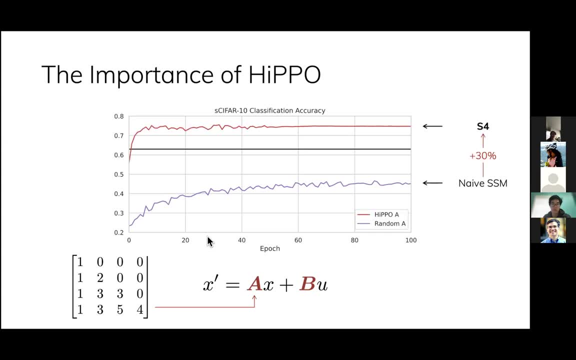 Okay, so that was one thing And that kind of points to. I mentioned that SSMs have not been used in deep learning before in this way And that's kind of one problem. If you do it naively it doesn't work. 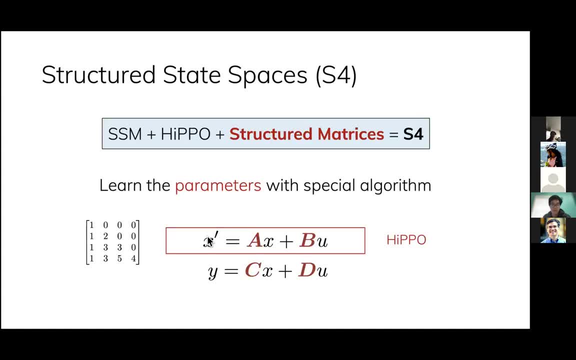 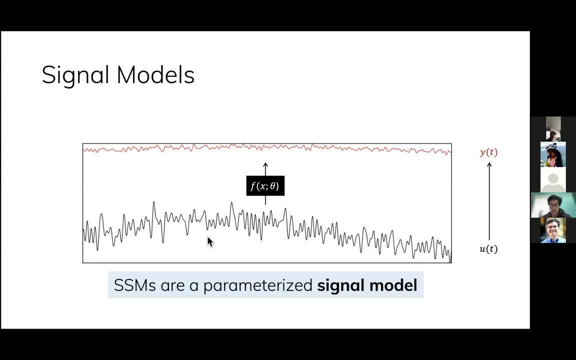 And so you need this new theory. The second reason is actually that they're computationally pretty difficult to work with, And so here's how to. here's to illustrate Again. so to remind you, we're thinking of an SSM as a parametrized map from an input signal. 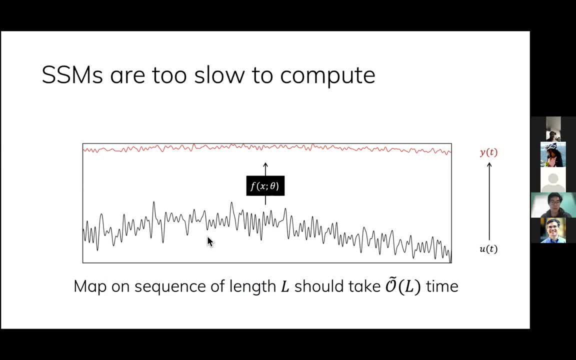 to an output signal. And now suppose that our input had length L, So our input would just gave us a sequence of L numbers. Then the output of this whole thing is also a sequence of L numbers, And computing this map ideally takes around O of L time. 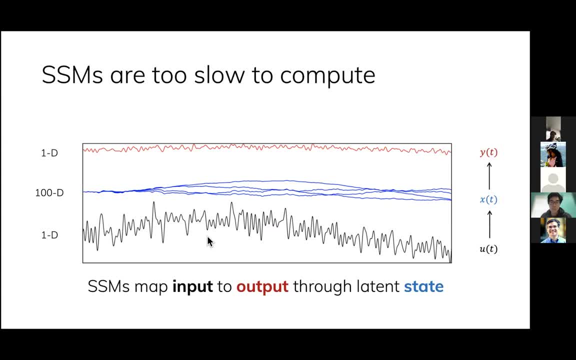 or not too much more. But here's the problem. SSMs map the input to the output through this state, And that state gave them a lot of nice properties, but it's also a hundred dimensions higher, And so computing the end-to-end mapping through the state. 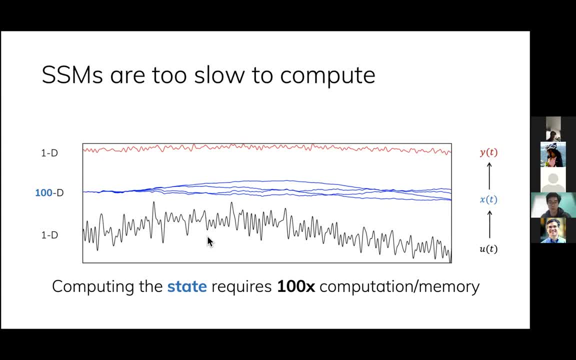 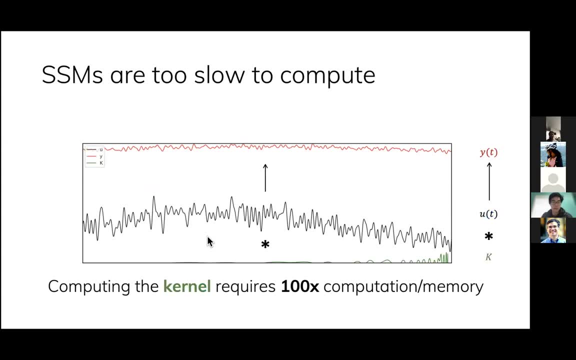 will take a hundred times more computation and memory than what's needed to compute the final answer. And this is actually a real problem. And now, earlier I said that you don't actually have to compute the state. You can compute it using a convolution instead. 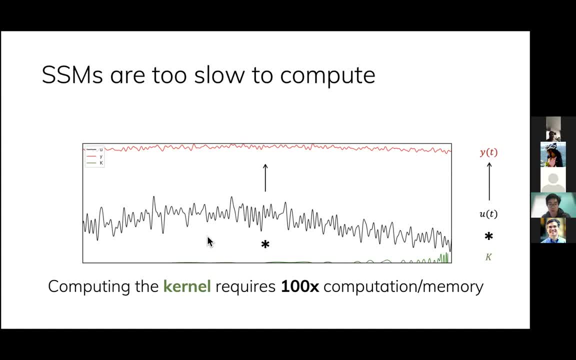 But what happens is that before computing the convolution I have to compute the kernel or the convolution filter in green, And computing that is just as slow as computing the state. And this sort of makes sense because it hasn't changed the computational hardness of the problem. 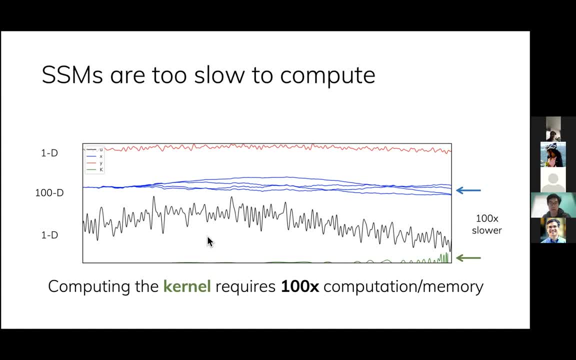 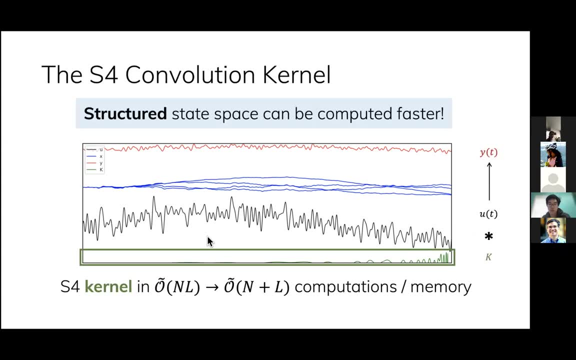 So, essentially, computing it, no matter how you do it is going to be slow and memory inefficient. So the main point of S4 was showing that you could substantially reduce this computation when the SSM is structured OK And, for example, when using the hippo matrix instead. 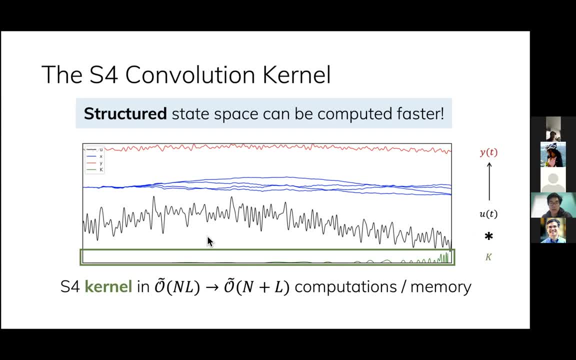 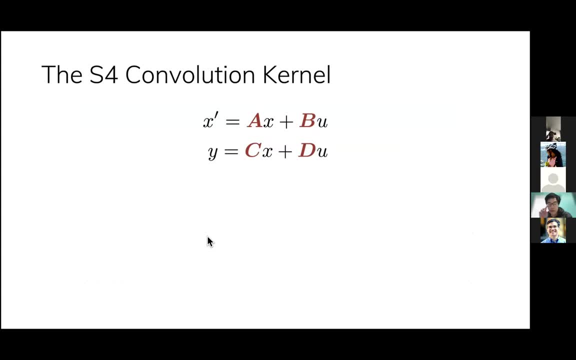 of an unstructured matrix, you can save this factor of 100 and make S4 overall extremely efficient. So this is done through a particular algorithm which I'll just flash up. But basically we're trying to work with this SSM. 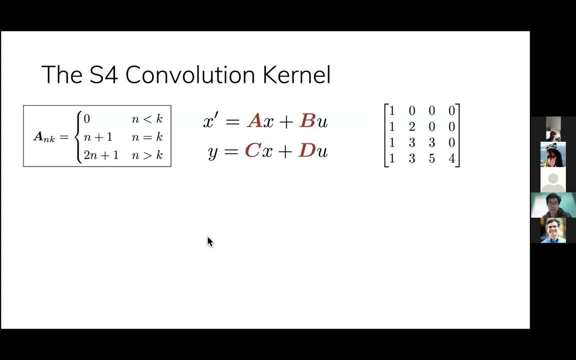 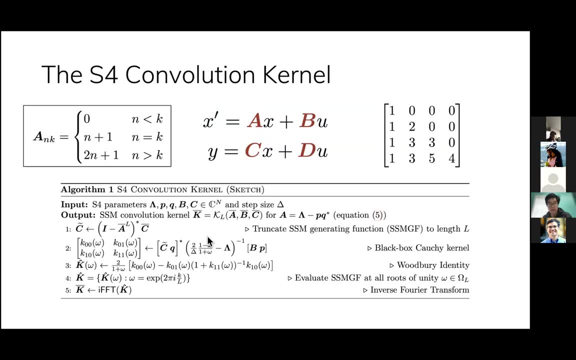 But we only need to work with specific structured cases, such as some particular hippo matrices, And now, using some algorithmic ideas, we can actually compute the state. It turns out there is a way to compute the convolution kernel, which was depicted in green before, very efficiently. 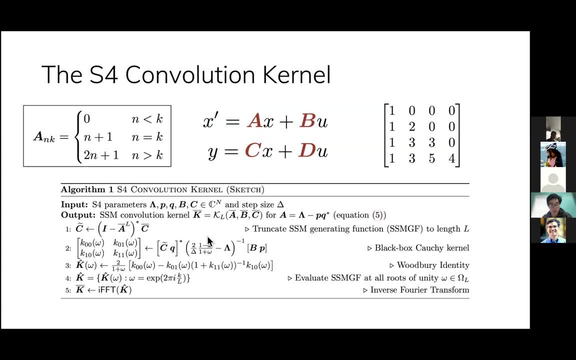 And then compute the whole thing using a convolution. So I won't go into details here, And I will also mention that recently we've been developing simplifications of the model that allow you to bypass all of this and do things much more simply. 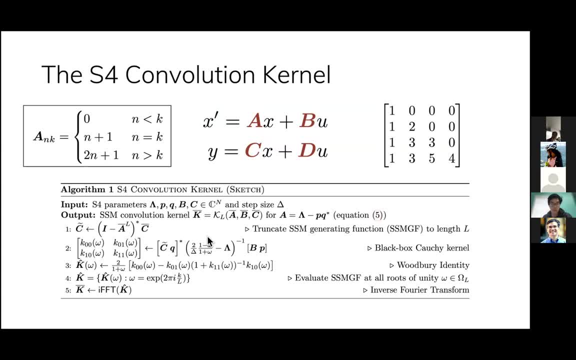 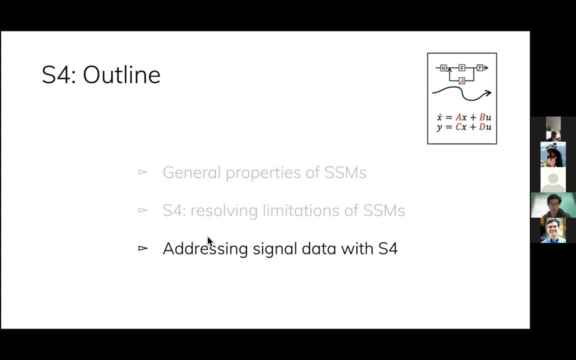 So hopefully in a few weeks we'll have some stuff out. that's where you don't need to worry about this really complicated algorithm. All right, So that was the technical portion that I wanted to mention for S4.. And I'll stop here for questions as well. 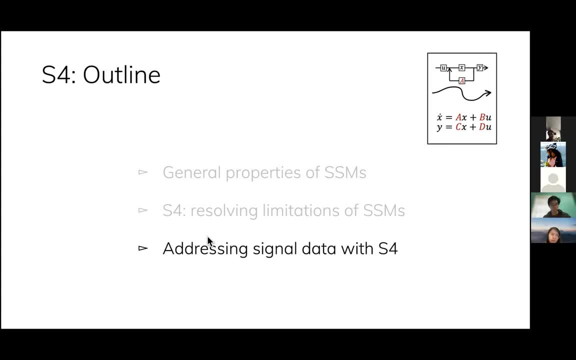 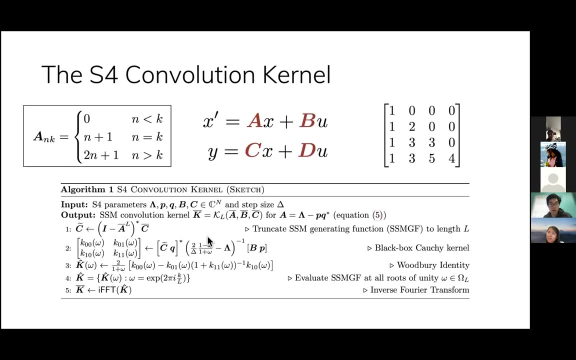 So if, in any case, you want to actually get the state, can S4 actually recover the state? Or is it like yeah, So I don't know if that would be any use case, But like let's see. Oh, so you're saying like, if there's a case where I actually 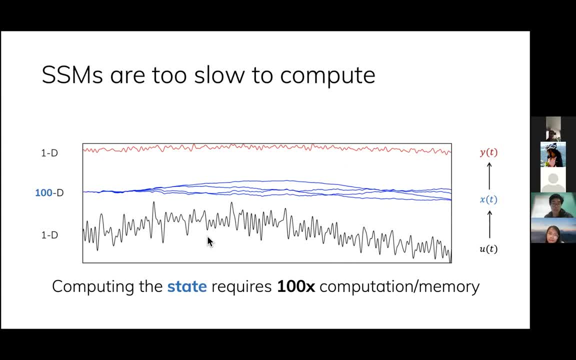 want the state. can I do that in the convolution? Yeah, yeah, Yes, you can, And in fact that will be used in some experiments I guess I didn't mention explicitly. But you can compute it in either way, either through the convolution or through the state. 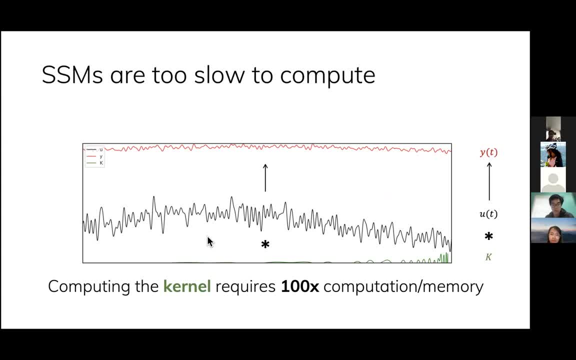 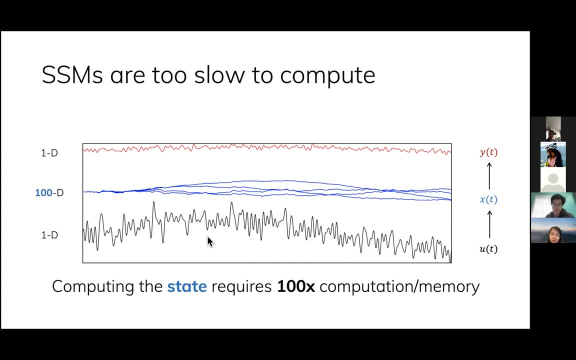 And where the state or the convolution is useful is during training time for parallelizability. But where the state is useful is at some sort of inference or deployment settings where perhaps you might be online And then you would actually be going through the state. 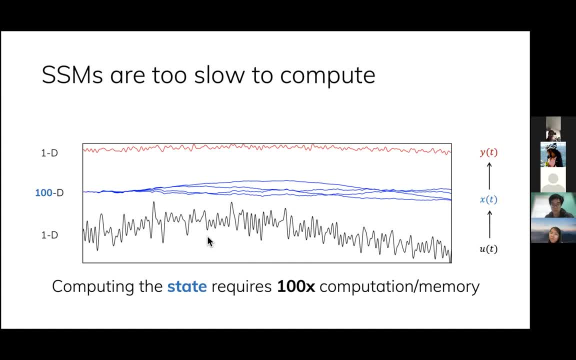 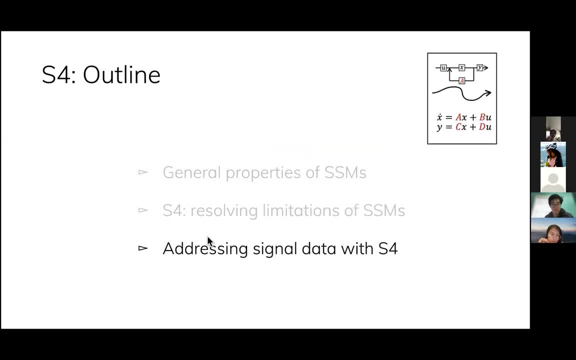 Mm-hmm, Instead of the convolution and unrolling things one step at a time, Right Makes sense, So you can do it either way, which is pretty cool. Thanks, I had more of a thought question. Let's say I'm interested in two different measures. 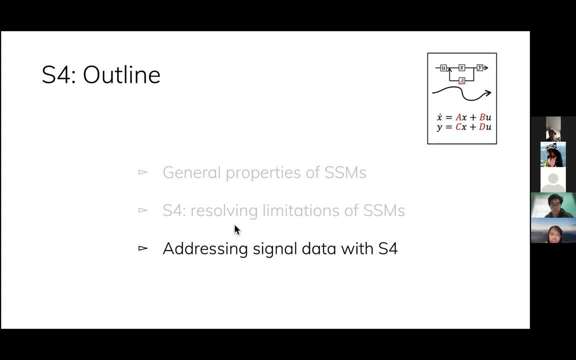 Like I want to see how the exponential average works, But I also want, like, so does it basically mean that I just have to create a new measure that combines this efficiently before this, Before I plug it into SSM, Or can S4 basically kind of pick out the two independent blocks? 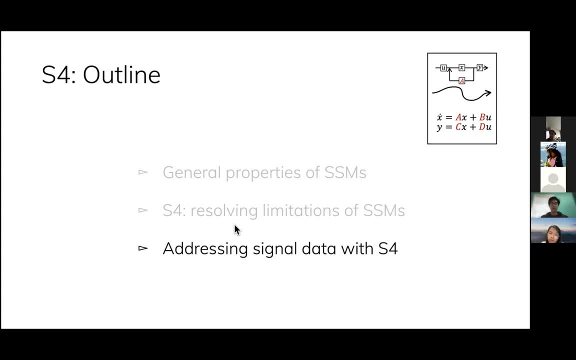 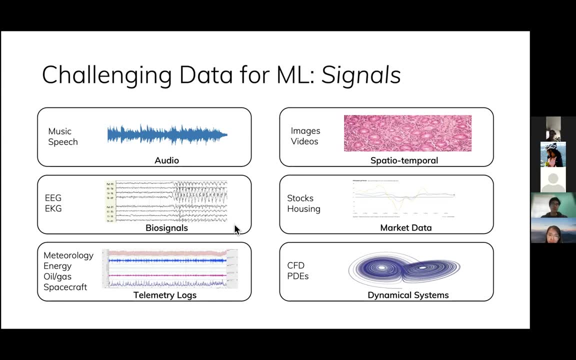 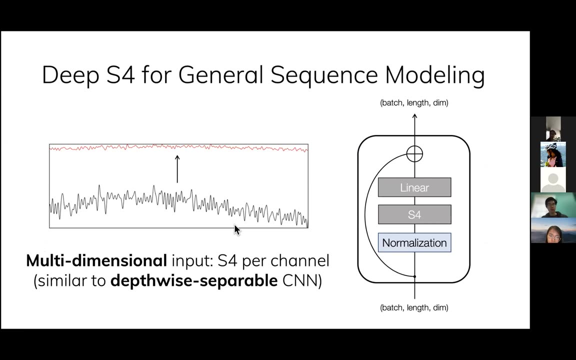 that I can basically Yeah, So I'm just about to get to the experiments And actually I'll get to that slide right now. So, first of all, the experiments will be on this type of signal data And, as I mentioned a couple of times, what we actually do. 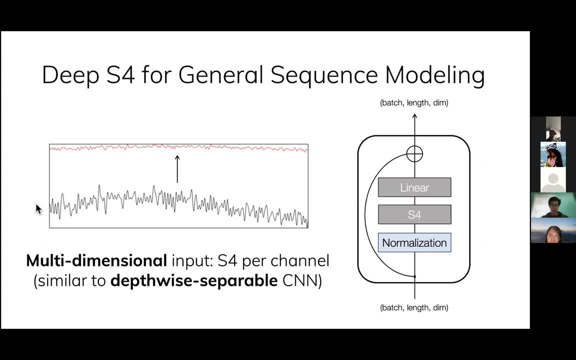 is that I've defined this 1D to 1D map, But I'm actually going to just like, given a multidimensional input, I'm just going to stack a bunch of copies of this And now, as a parallel to that, you. 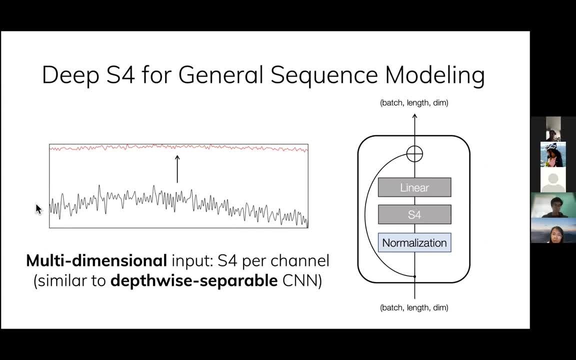 can do many things with these copies. So, to answer your question, one thing that I've been starting to experiment with is just using different measures or essentially different A and B matrices for every copy, And that sort of has an interpretation of using multiple measures. 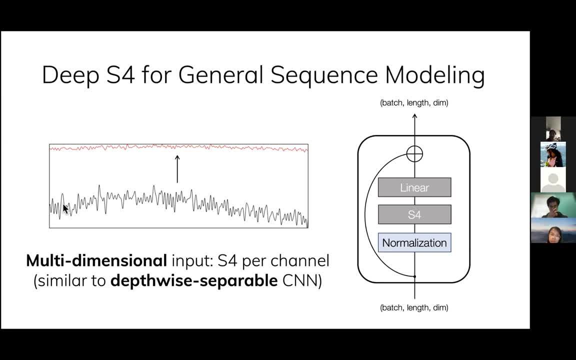 I see, Because when Iman actually did that, I was like, oh, I'm going to do this, I'm going to do this, And Iman actually talked about the correlations between different dimensions. Let's say, you have an image. 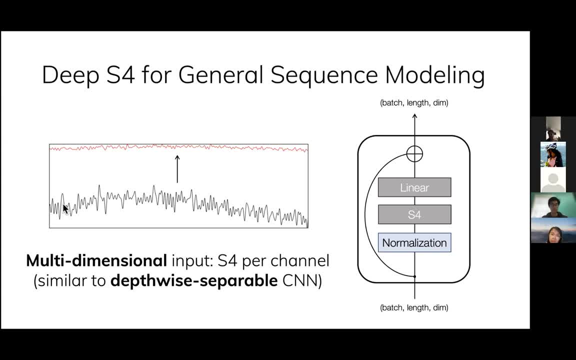 Two different pixels are actually correlated, So I was thinking you can have a measure that captures this correlation, but you can have another measure that captures it over time. Yeah, Another thing actually, since you mentioned that- I don't know if you tried that on image space. 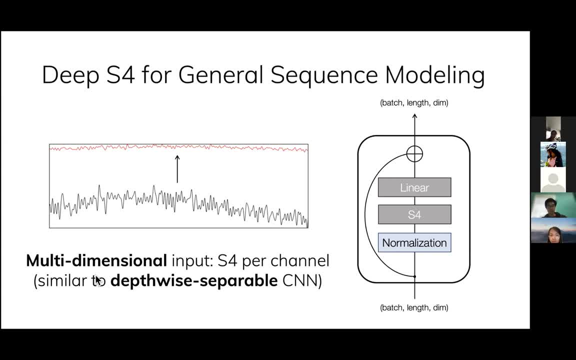 I would be curious if this kind of long convolution actually makes any difference with the image space, Because image usually- like when we do the image analysis, like theoretically, when we start thinking about it, it seems that also the local feature, as well as, of course, 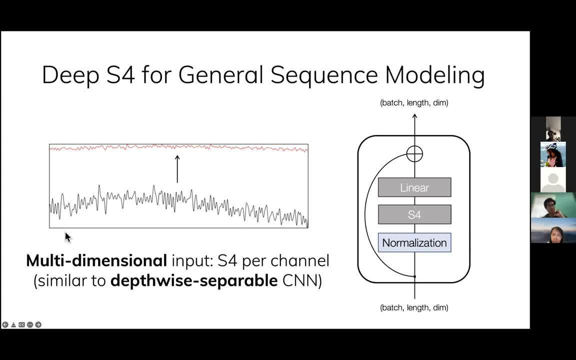 the global feature is important, But I don't know if we are missing any local features by just using this kind of long representation. That's a good question. Actually, we have started doing more experiments on images, which I didn't include in this talk. 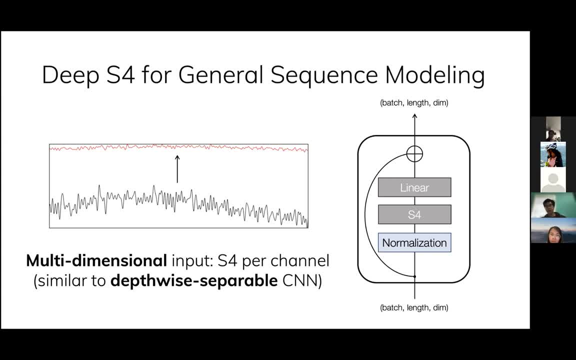 But colloquially we do find that the local bias of convolutions does seem pretty good. I don't know, It's hard to quantify if we're missing features, But I think there are settings where we're only on par or not. 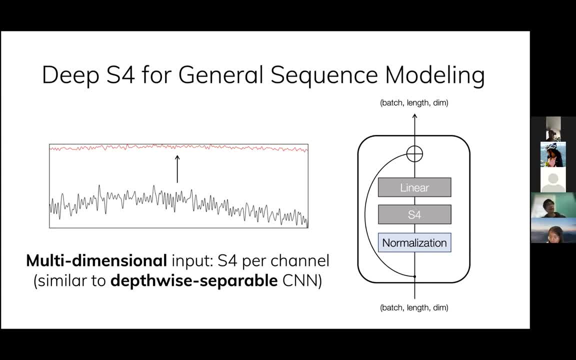 or maybe a little bit worse than a standard local CNN. It is hard to say. I will mention, though, that you can forcibly incorporate locality into this just by changing the measure, For example, if you choose a uniform measure that has a short window. that's the same as saying: 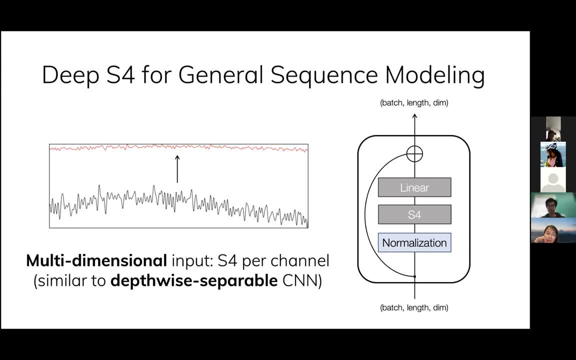 I just want a local convolution kernel Because I would imagine, like for this particular thing, the use case where we have to have to work with a very high resolution image data- for example, imagine a mammogram- We have to go with 1,000 by 1,000 minimum dimension. 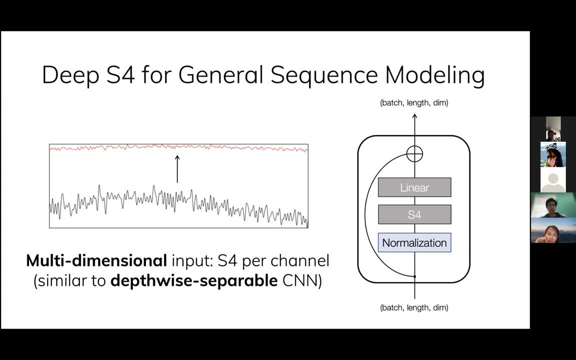 So these probably would be useful because they are actually. we want to do the rescaling but we cannot because we'll lose probably a lot of features in the middle, But this kind of long convolution could prove it. This is a perfect problem that I will. actually I wasn't going to. 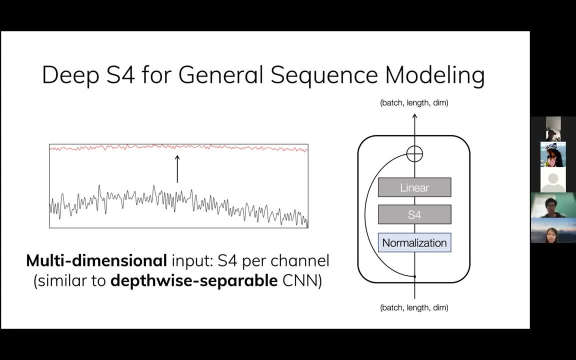 but now I will mention this in the experiments as well. It's actually something that we have thought about, basically rescaling of convolutions and using global set. I'll get to that Before that. so I want to get to experiments And basically I just wanted to find: 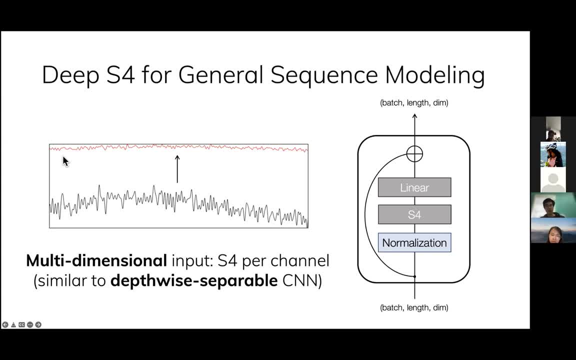 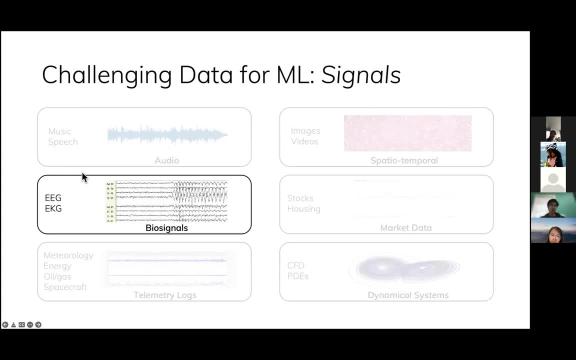 I've only defined this simple linear 1D to 1D map but you can just do it in parallel across a lot of features and then plug it into a standard neural network to do sequence modeling. So the first type of data I'll see is 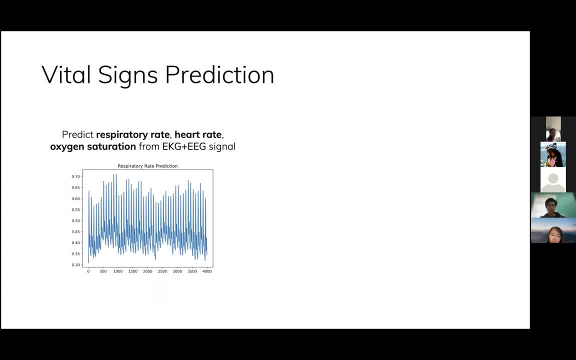 is a biosignal data, So here is a. there's a real world data set of trying to predict vital signs such as heart rate from raw biosignal data, such as. I wrote EKG and EEG here, but I think it's actually EKG and PPG. 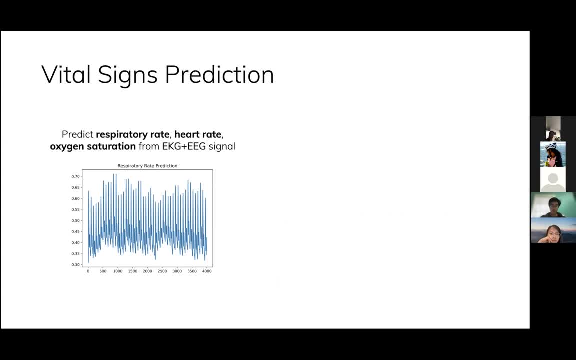 And so that's visualized here. And this data is pretty challenging for deep learning models because you can see that it's very long. This is a sequence of length 4,000.. If you zoom in a lot it would be pretty smooth actually. 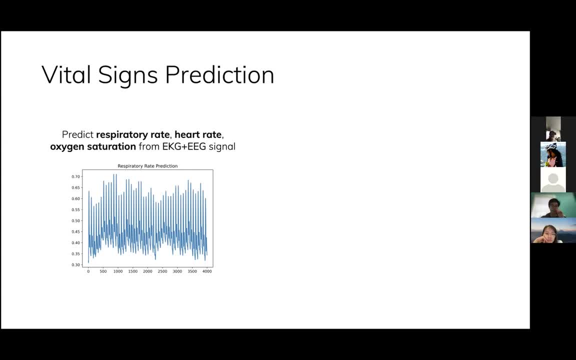 But if you zoom out it displays a lot of periodicity and spikes and other things, And so a lot of methods have been tried on this data set, which include kind of standard machine learning techniques like XGBoost, as well as many very modern. 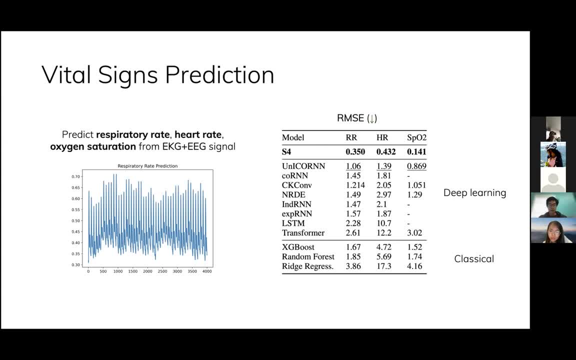 deep learning sequence models And S4 substantially improves over all of these in. I think, cutting the root mean squared error by at least two thirds on all of these targets, Just with that generic deep learning model, that deep model that I showed. Actually these were like older numbers. 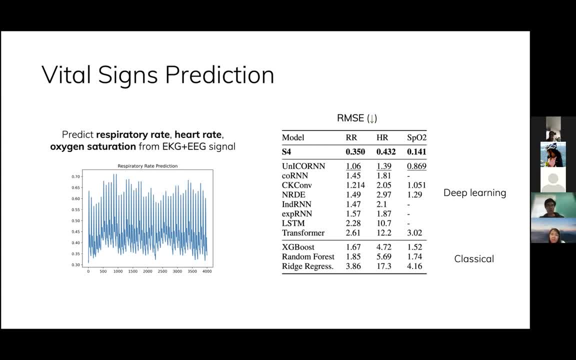 and recently I've been re-running these again and actually you can drop this down even more. One thing I will note is that Attention and Transformers does really poorly on this type of data, And that's something that I think I found pretty consistently. 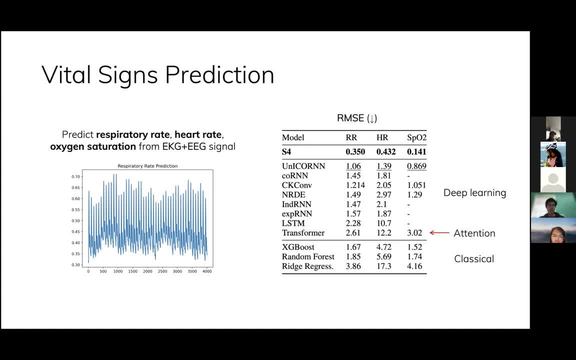 So there's some sort of bias for what type of data you have. and S4 is really good at signals and attention is not. Conversely, attention is good at some other types of discrete data that S4 is not as good at. Okay, so that was one experiment. 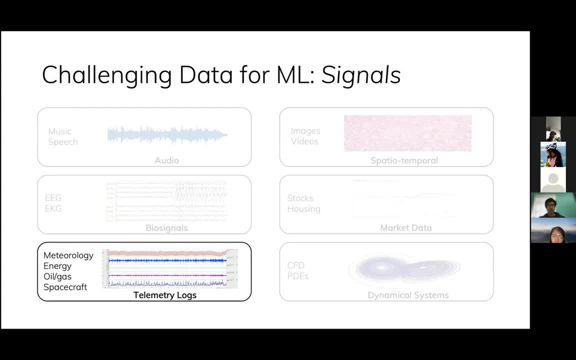 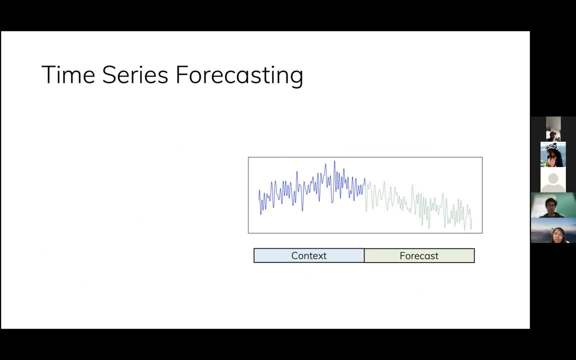 The next one is to time series data, where we did a forecasting task, where you're given a context window and you wanna predict future values. Actually, I'm gonna go through this kind of fast because I don't have that much time and I wanna get through some more of the bio applications. 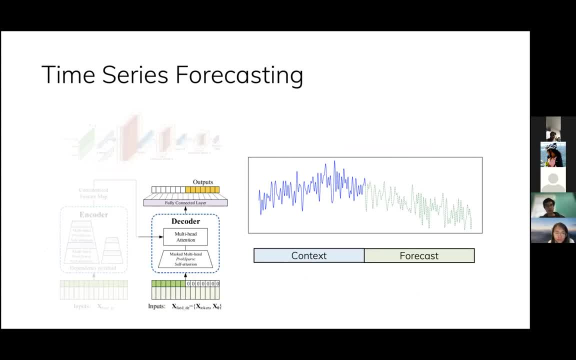 and the things that you guys brought up. So the models here are very complicated, Whereas for S4, we're actually doing an extremely simple setup which is just a mask prediction We're just gonna give you, we're gonna take the entire sequence. 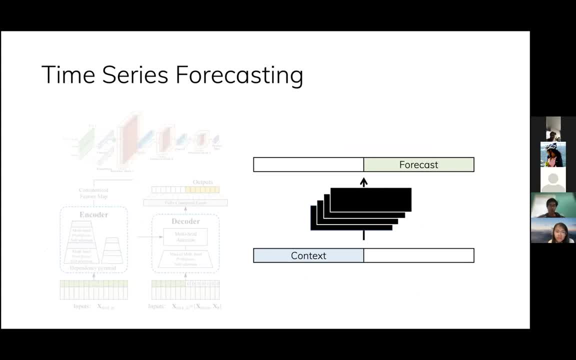 and mask out the desired forecast range and then just predict what's in the mask by passing it through this generic deep model. So this is really it's like a extremely simple application. I won't unpack the numbers too much, but there's a lot of baselines here. 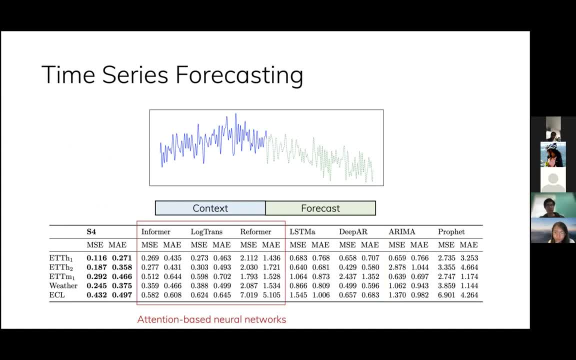 including time series models. LSTMs lots of transformers and S4 does better than all of them on these real time series data sets, including weather and energy data with much less specialization. These models were all designed for time series and we were just using our generic model. 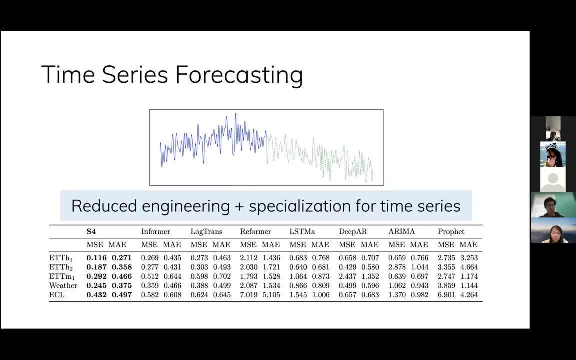 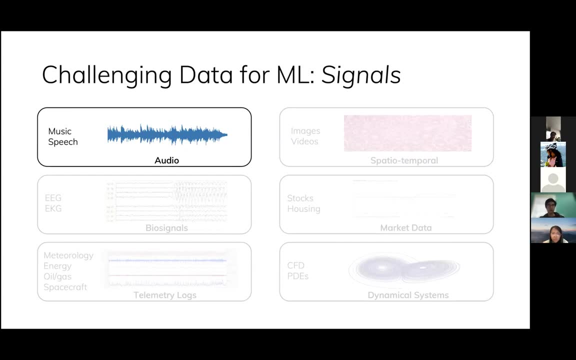 And you didn't even tune the window size right? We did not for this one. Actually, by tuning the window size you can get the numbers down even more, Okay, Okay. the next one here points to Iman's question about rescaling. 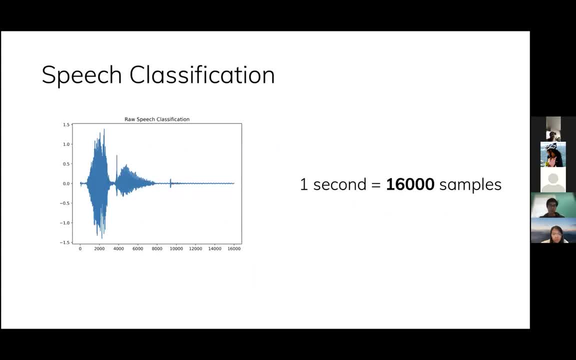 So it's actually. I'm gonna display this to audio, but essentially I've used audio a few times in a running sample. It's sampled at an extremely high rate and it's extremely long, So this is a dataset of classifying one second speech clips. 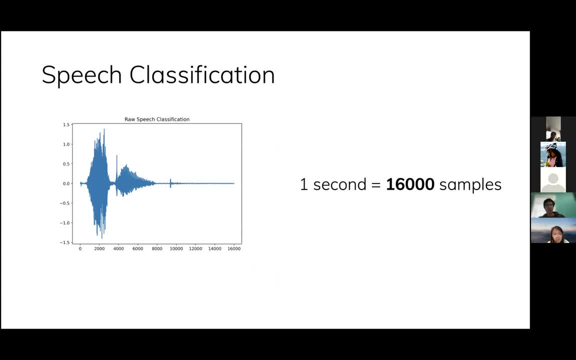 which were linked to 16,000, into classifying the words And most sequence models like transformers and RNNs are really bad here. The only thing that works is CNNs, which the red line is pointing to a speech. CNN baseline. 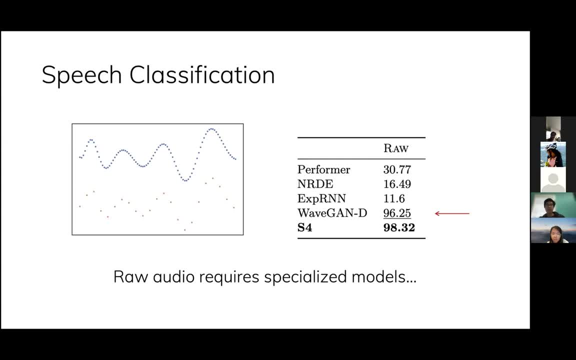 And these work okay. but what happens if you are resampling the signal at different frequencies? And this happens commonly in audio, because your signal can be sampled at any rate and sound more or less the same. So, for example, this orange sequence is a sequence of samples. 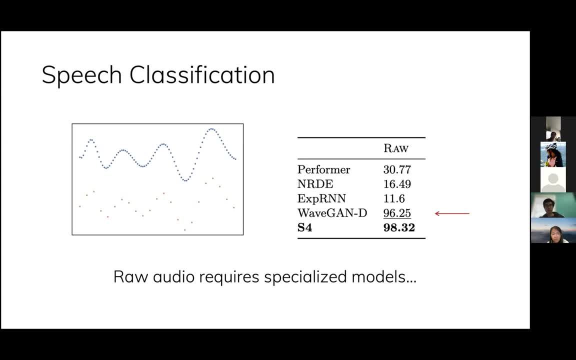 but it's actually the same underlying signal as the original blue sequence of samples, just at a different frequency, And so it's ideal if the same model works on both of them, But standard models like CNNs cannot do this, essentially because of the local bias. 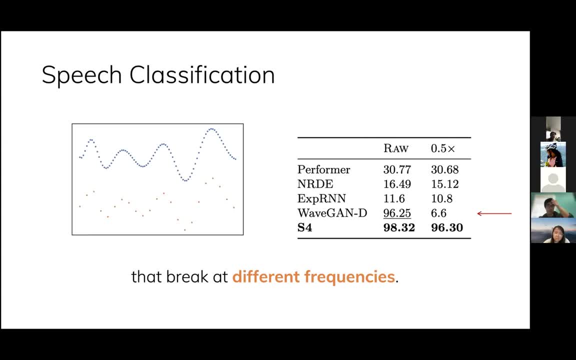 that was brought up earlier. I won't unpack this here, but if you use like a standard local CNN, it will break at a different frequency. However, by using a signal model such as S4, which is actually understanding the underlying continuous domain, 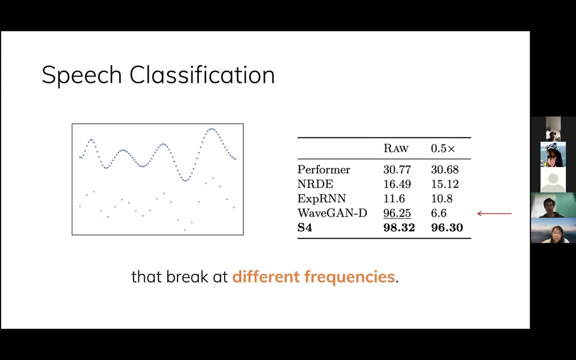 or the underlying continuous function. it can work here without modification. So this is all in the same way. So this is all in the same way. So this is all in a zero-shot setting, where it's trained at one resolution and tested on a different resolution. 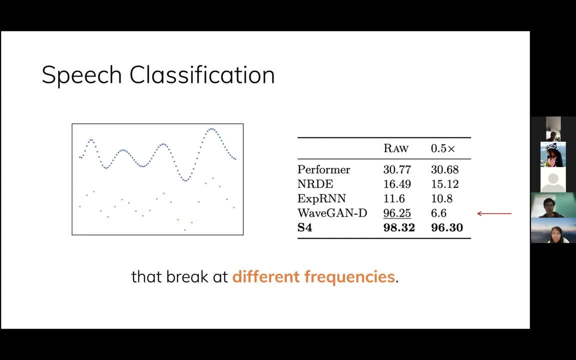 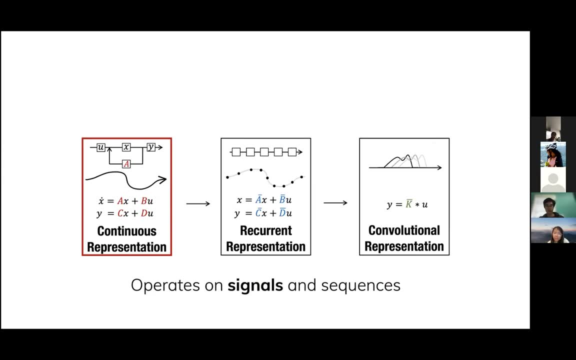 And this breaks a CNN. but S4 can do it out of the box, And that's because of this first property of being a continuous time model. And now the last two things I'll show are just calling back to the experiments at very beginning. 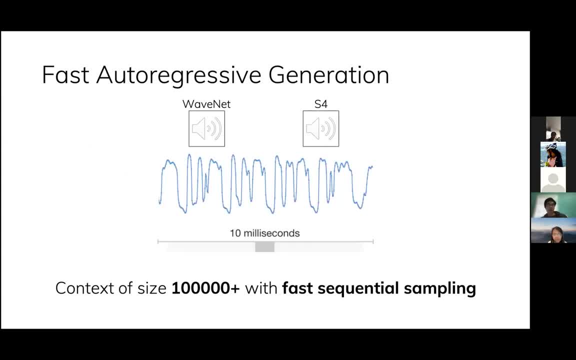 I showed some audio generation clips and that was an auto-regressive setting where we're generating things one sample at a time And, despite having an extremely large context window, which made it do better and more coherent, we could still sample things auto-regressively. 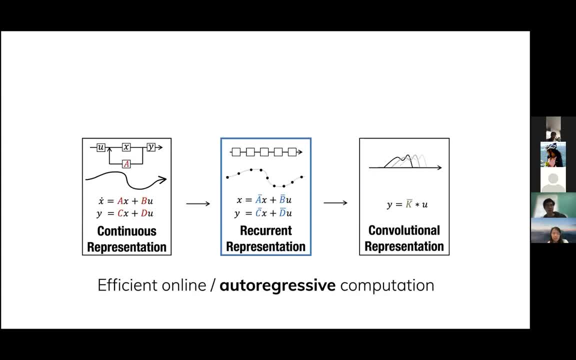 just as fast as other auto-regressive models, And that's because of the fast online or auto-regressive representation, where you're computing the state and updating it every time. And finally, I showed this benchmark of long range modeling, where S4 substantially outperforms other models. 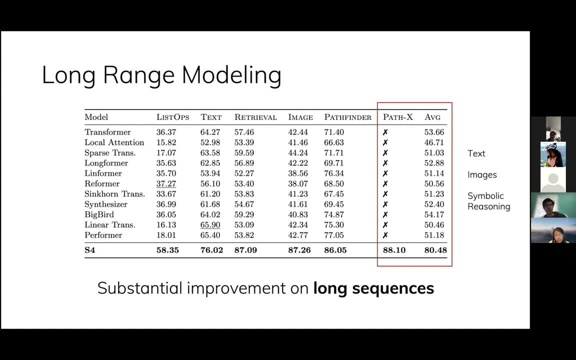 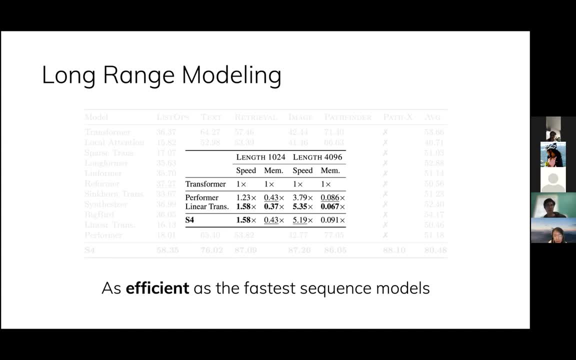 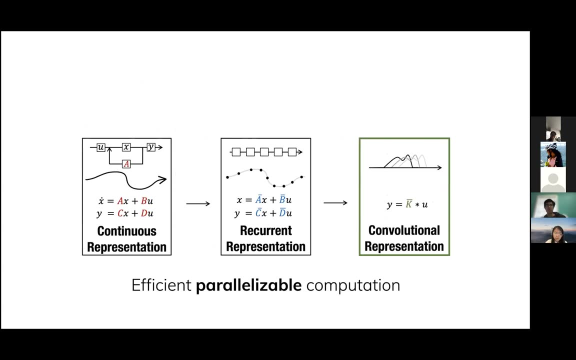 on a range of different tasks, And this benchmark was also used to benchmark the speed of models during training, where S4 is just as fast as all of these efficient transformer variants, And that's because of the efficient paralyzable view, along with the new algorithms we introduced. 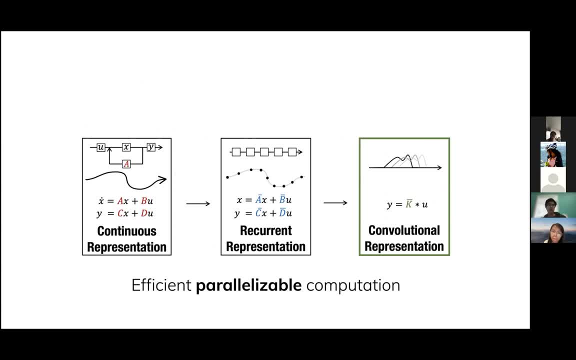 And so all these properties, as I promised, have concrete empirical benefits. Now, for I'm running out of time, so I just want to get to a couple more things For the last part. I just wanted to for this audience. 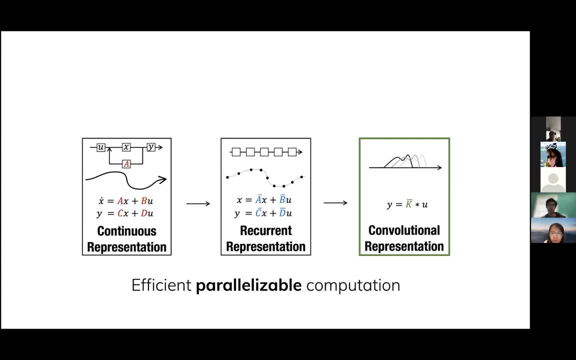 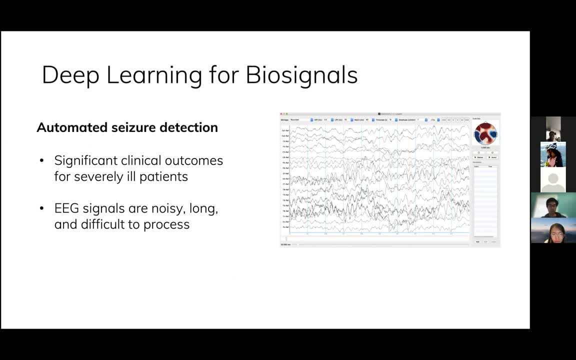 I wanted to point to where I hope that this model, where I hope that this model, where I hope that this model will be useful, which is as a general tool for deep learning, for biosignals, And I've pointed out one example of a data set already. 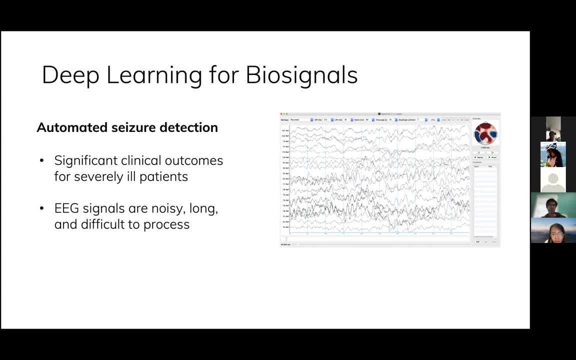 where we were predicting, like heart rate, from EKG signals, but this was another one that CE was working on, actually, and her and another lab mate have been trying to test S4 here, where this is a data set of raw EEG signals that are difficult to process. 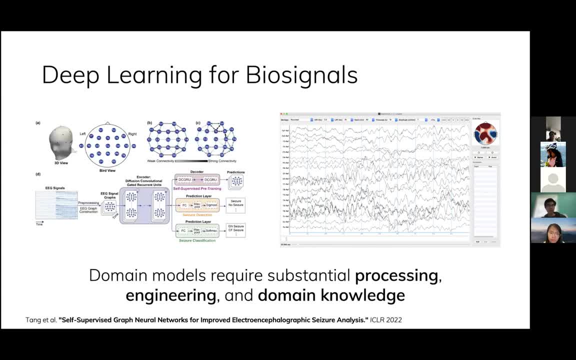 because they're so noisy and long And and the state-of-the-art models are very recent. CE's model from a couple months ago was state-of-the-art on one of these EEG data sets, but it was quite involved and involved a lot of domain knowledge. 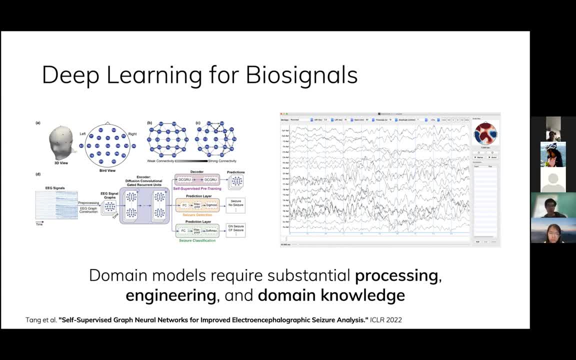 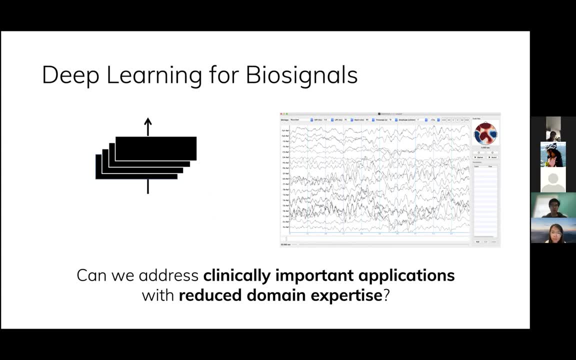 such as even like the placement of the electrodes and a lot of different parts, components of the model. And so where I hope that S4 could be useful is as a generic tool or building block for addressing these types of signal data without as much domain expertise. 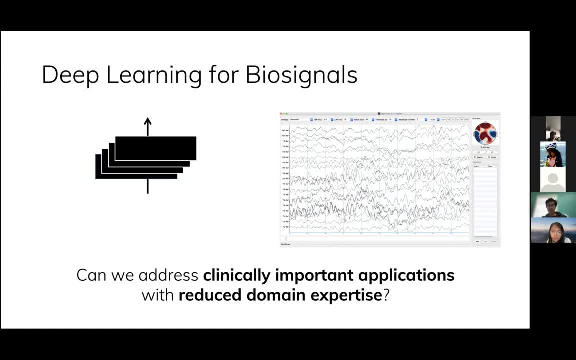 in how to design the model, And so CE and Khalid have been running some preliminary experiments using S4 on this data, where we don't even need to process the- you don't need to pre-process it with FFT features, You don't need to do a lot of these other things. 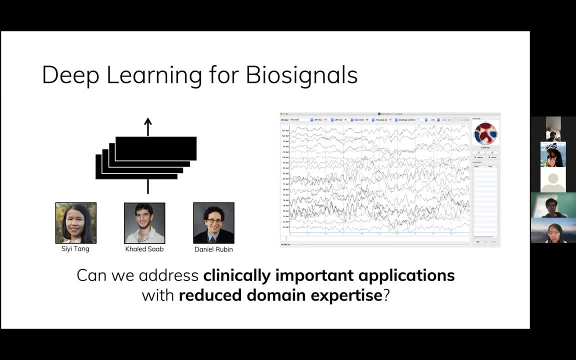 and just run it through these- a generic deep model composed of S4 layers- And Khalid found some very preliminary results where it is improving over the baselines in some settings. This is still very preliminary, So it's not. there's other settings that we care about. 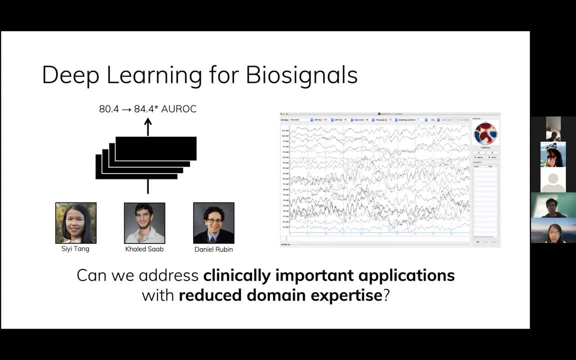 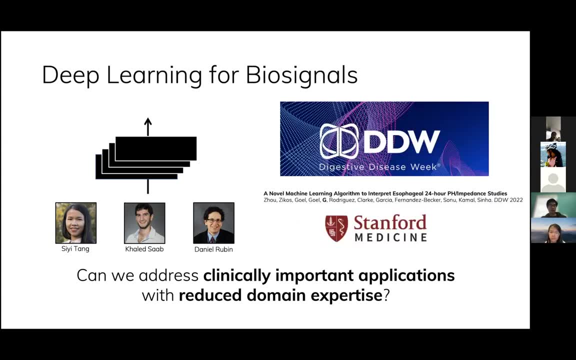 such as incorporating self-supervision and so on, where it's not quite there, but I do think it has a lot of potential in this type of domain. Another example actually that was published was another recent collaboration with Stanford Medicine that was submitted to a gastroenterology journal. 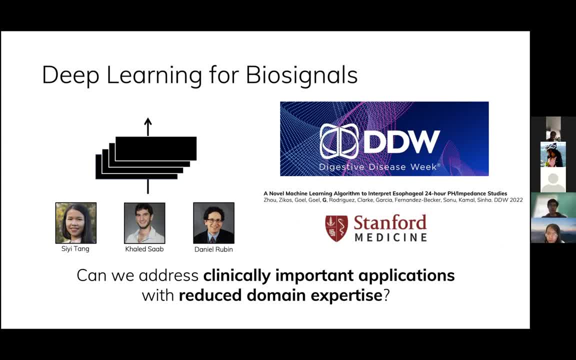 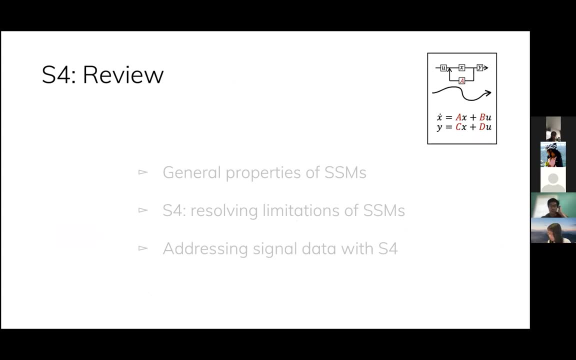 on detecting acid reflux from impotence sensor data, And so, again, S4 was really good on that type of prediction task. So that is all I was going to talk about for this. So just to review, S4 is a, it's an SSM. which are these two equations? 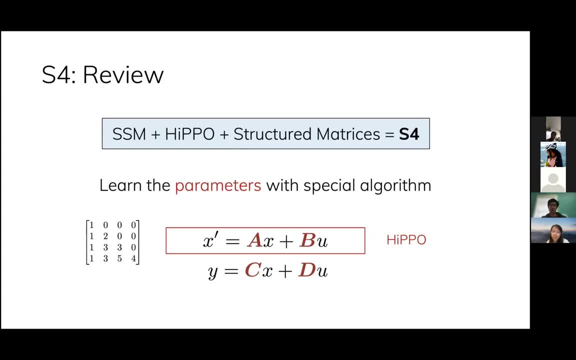 where we plug in certain formulas and have special algorithms to compute the model And overall SSMs and, in particular, S4, have a number of and, in particular, S4, have a number of and, in particular, S4, have a number of. 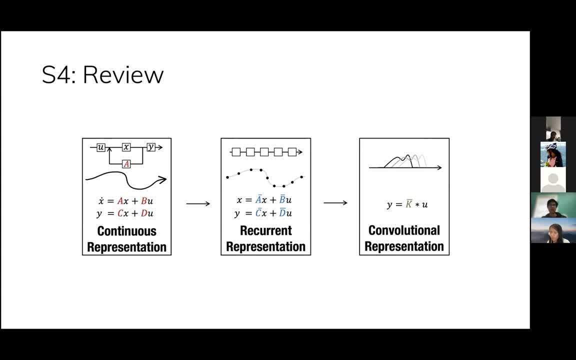 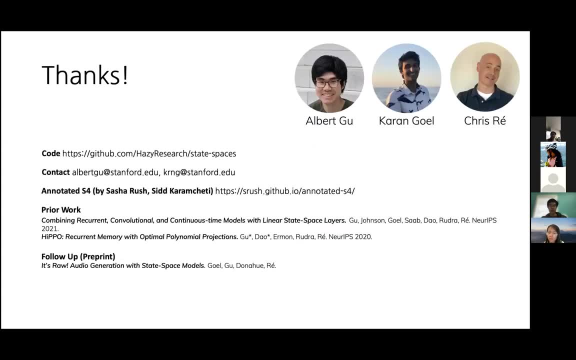 a number of very nice properties with concrete empirical benefits, as we saw, and I think can become a very effective building block for modeling many types of sequential data in the future. Thanks for listening and thanks for all the collaborators for the hard work. 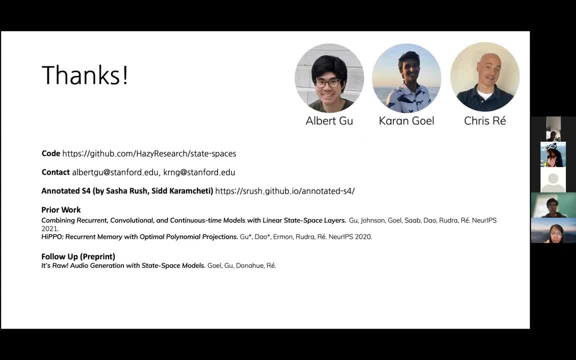 This slide lists a couple of resources, such as blog posts and related papers, as well as the audio results from an ongoing a paper that's under submission right now. Feel free to reach out if you have questions. and thanks, This was my last slide, but because I want to ask. 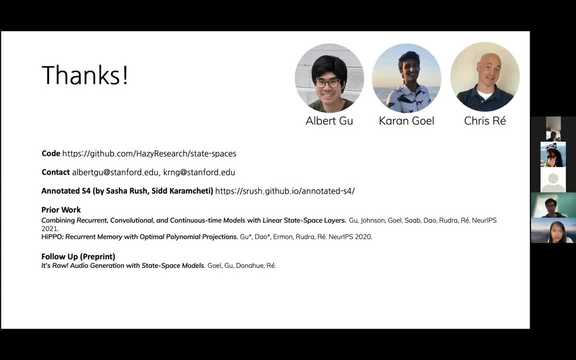 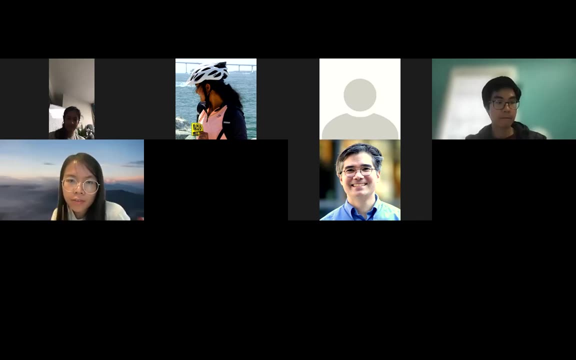 I will. I guess I'm technically out of time. so of course people feel free to leave. but if you want to stay, I can show one thing about the high resolution images that was brought up. Let me find that slide. Yeah, if people have conflicts, feel free to leave. 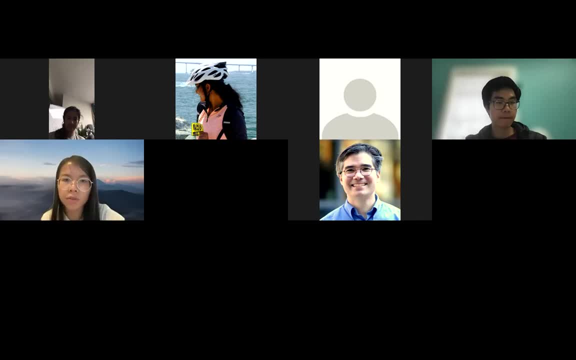 and we will put up the recording of the talk later in our YouTube channel. Otherwise, if you would like to stay, then yeah, I'll be happy to share. Share the slide. So yeah, I'll just really quickly go over this. 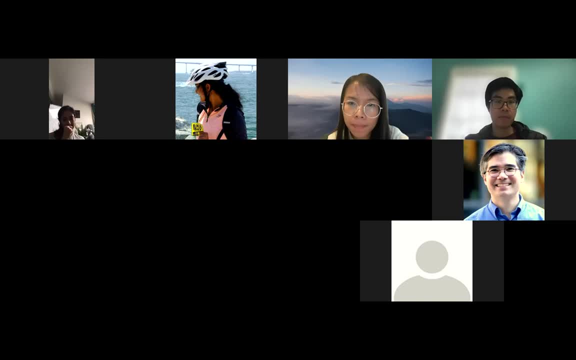 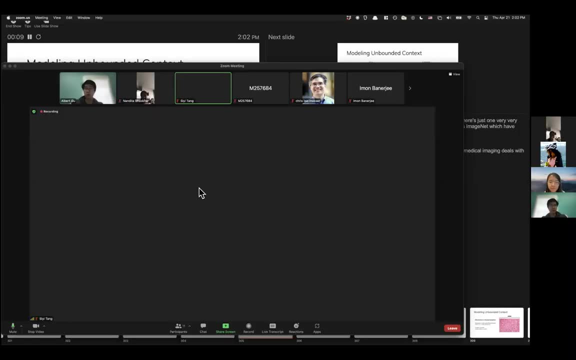 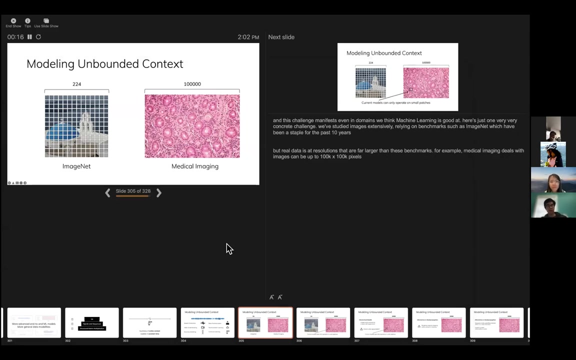 where medical imaging is something that we think could be a potential strong use case for S4 because of this high resolution feature. where so this slide was about? I was moving in a different way, but the point I wanted to make was that- Can you go to presentation mode? 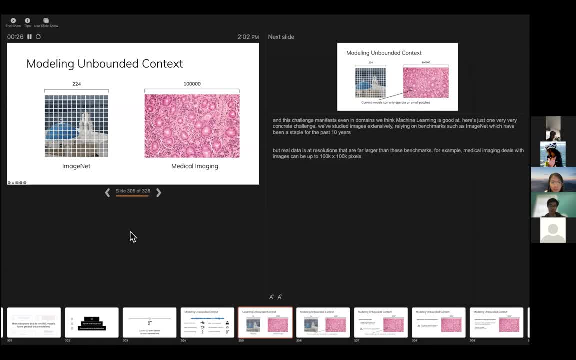 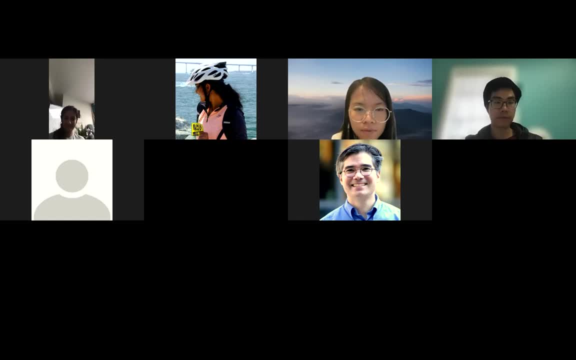 I think-. Yes, yes, I'm still seeing your screen notes. Yeah, sorry, Oops, Am I sharing my whole screen? No, we are seeing your screen rather than the presentation. Okay, I thought I had it on the-. You can just swap the view, you know. 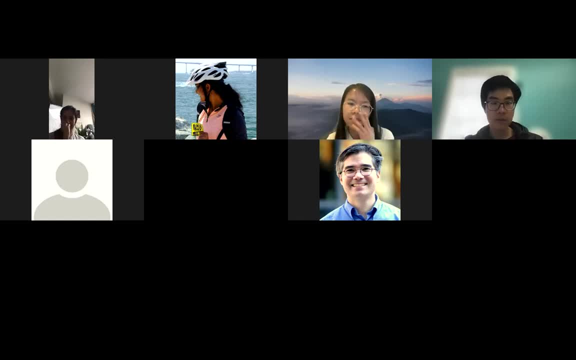 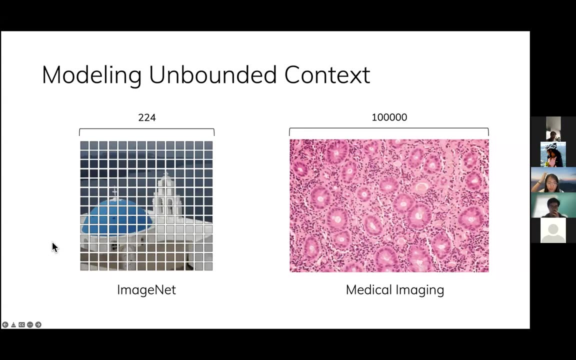 I thought I had it on the right view. Is this one still show the oops? Yeah, I can see that It has your presentation view. Okay, great So. yeah. so the point I was making is that normally image data sets are things like ImageNet. 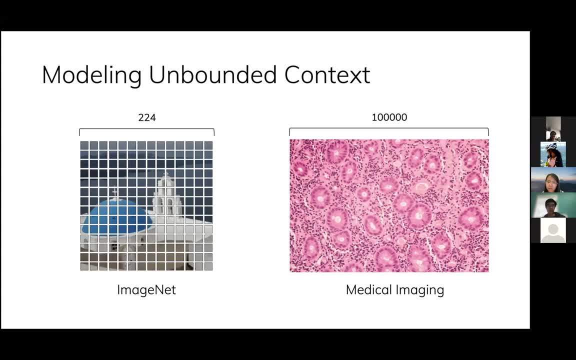 which are actually extremely low resolution compared to other data that we might find, such as medical imaging, where apparently the images can be up to 100,000 by 100,000 pixels, And this is obviously like way too big for current models. 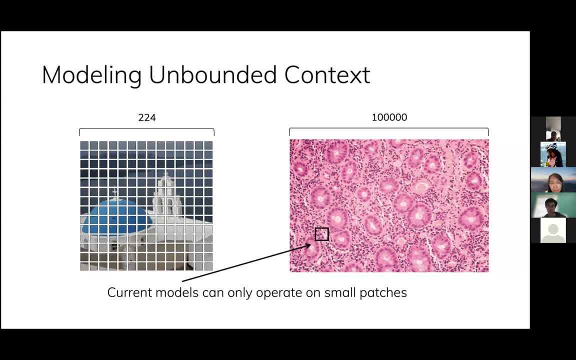 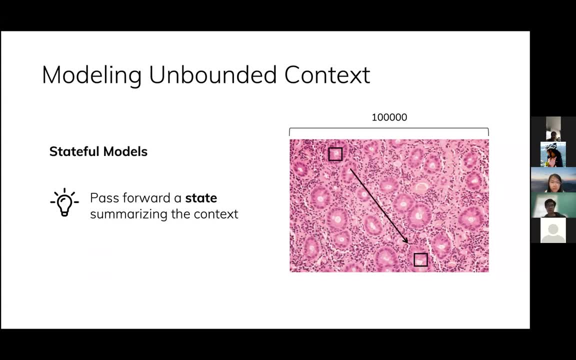 which can only operate on small patches at a time. So I don't know how to address this really, but it's something that fascinates me. But just to point to this is part of a longer job talk where I point to some potential future directions. 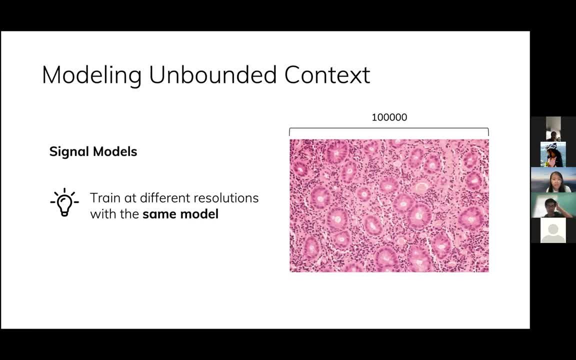 The one that I'll mention here relates to some things that we brought up, which is that, just like the speech experiment that I showed, I believe that S4 should work- training on images at different resolutions- And so what you can do is essentially try to train. 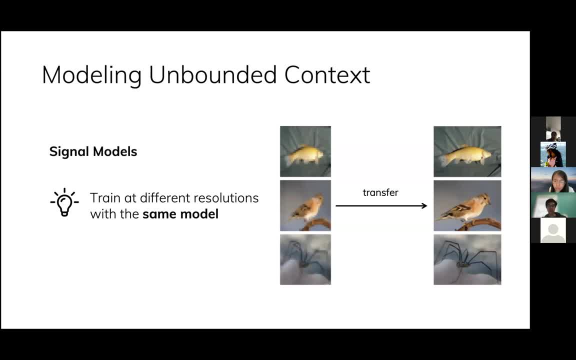 on lower dimensional versions of the image, lower resolution versions, and then transfer the same model to work on high dimensions, which is a very similar thing that I showed for the audio of the speech example. So yeah, I think that's potentially something. 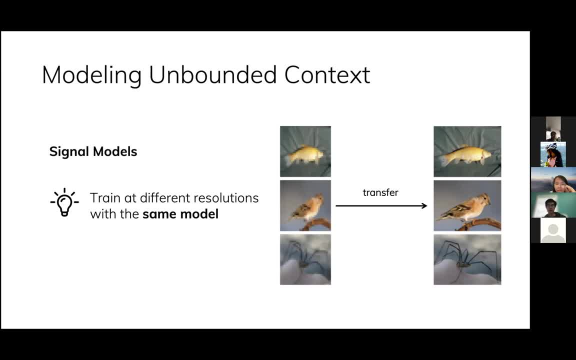 that could work, And the point is that a signal model like S4 will work at different resolutions because you can sample at different rates. essentially, And yeah, so what you need is a signal model that understands the continuous domain, just like the example I showed. 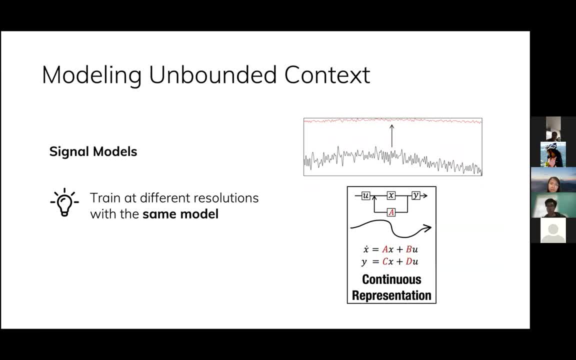 And that points to this property again. so this is something where we haven't tried it and I don't know if it works, but some part of me feels like it might be the right way to, or one potential good way to approach this type of problem. 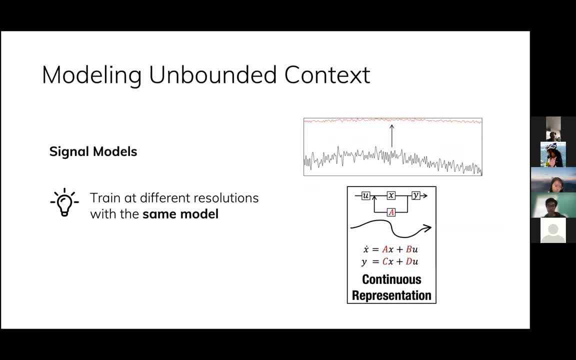 But I would think in the opposite way. you know it's not really we want to generate the high resolution from the low resolution, but I would imagine, since you have this kind of like state based representation and finally you're getting this signal, 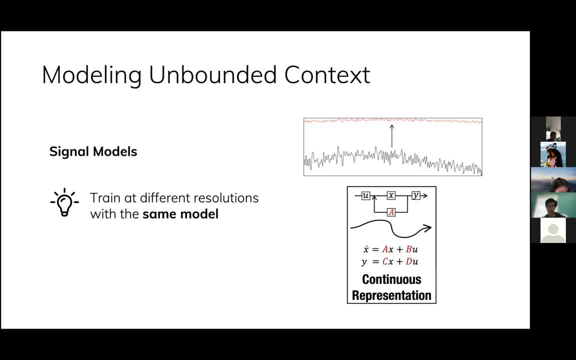 I would imagine, like in some case, always, like we had to deal with this kind of situation, that we had a very high resolution image and before running through the convolution because of the, you know, like the memory computations, like computational complexity, memory complexity, 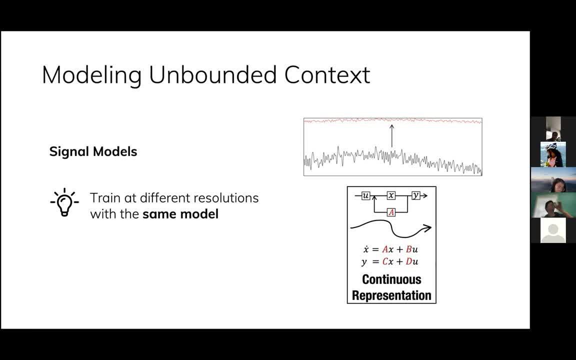 and all this kind of thing. So you have to rescale the image into a much lower dimension. Yeah, And we had a chance of losing a lot of features, specifically histopathology- exactly the example that you showed- or the mammogram, those kinds of images, you know. 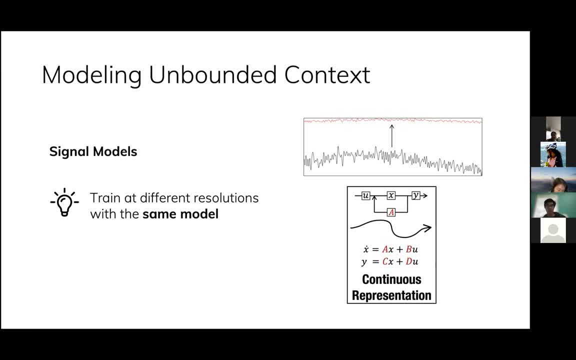 Yeah, I see. So I was thinking that perhaps, like what you can do is kind of like iteratively increase the resolution and pick up higher and higher resolution features as you go. But the benefit is that perhaps you can pick up the coarser grain things. 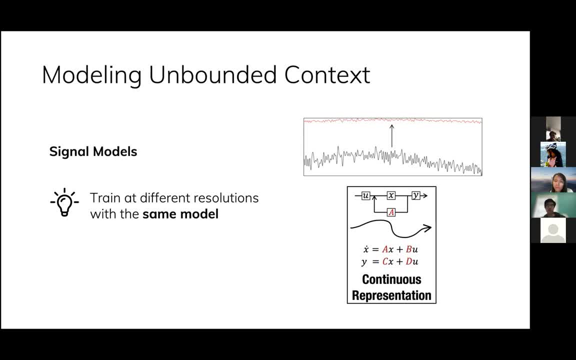 and then as you upsize the image then and you rescale your kernel, essentially then it's already going to be doing. everybody knows the coarse grain features, but then it, as you keep training, it only has to learn the higher frequency features as you go. 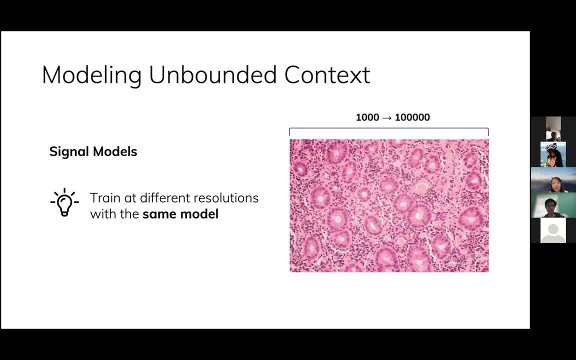 And again, I have no idea if this is, if this makes sense or it's promising, but it's just a goal. It sounds pretty interesting, I think. I think Elbow's idea, you know, is like Elbow's idea, is actually very similar. 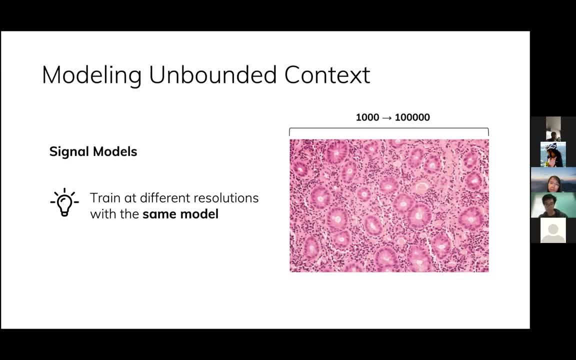 to how pathologists analyze a whole set of images. So they usually look at, Define zoom, define zoom resolution. They usually look at low resolution image first and localize, like the potential areas where the tumor are, and then they zoom in to higher resolution. 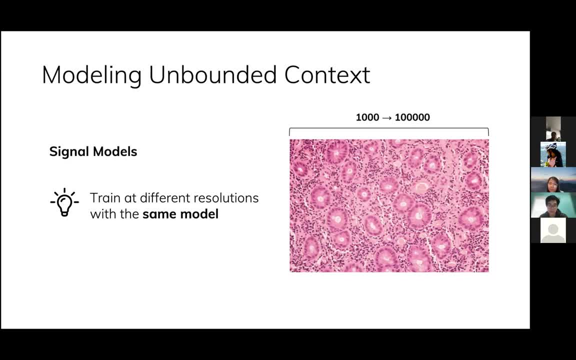 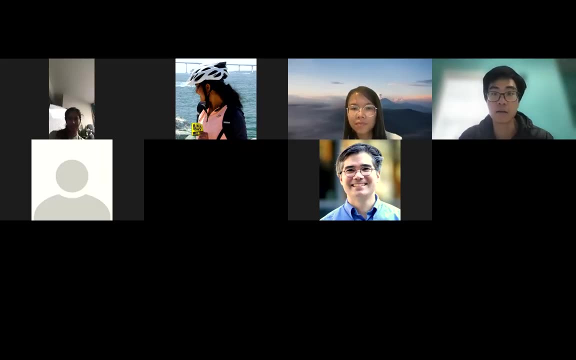 Right, Yeah, I see yeah, And so, yeah, I don't know if this will be better than CNN or other things, but it definitely has different and interesting properties. Okay, So that was yeah. I think that's the end of the material I have. 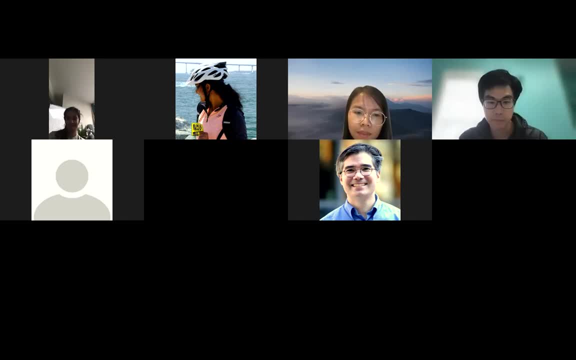 I can stay around a few more minutes. if people still have questions, All right, Great. Thanks so much, Albert. I have just one question. Sure, Yeah, Thank you for the presentation. That was awesome. Did you find any scenario where it's better? 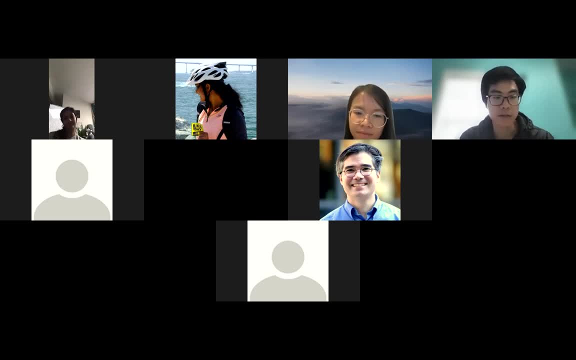 to use transformer than S4?? Yes, Another great question. So let me just share my screen again. I have one slide prepared for that. Basically, at the beginning I drew this distinction between continuous time- kind of continuous- and discreet data, And I think that S4 will be the best. 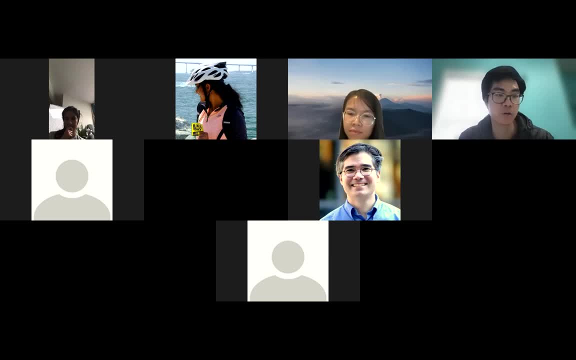 or like the ideas involved are potentially going to gonna be the best thing to do for signals, but for kind of higher level concepts or more discreet concepts such as language or some other things transformers. I think that's what S4 will do best, or potentially going to be the best thing to do for signals, but for kind of higher level concepts or more discrete concepts such as language or some other things transformers. I think that's good. 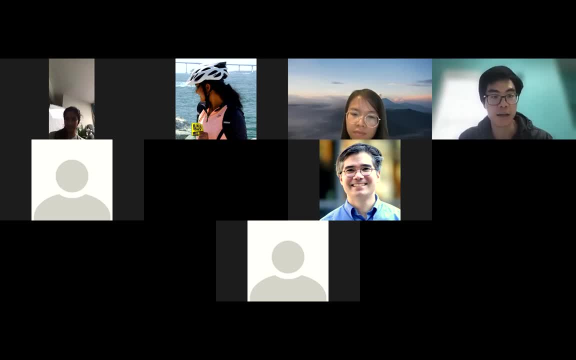 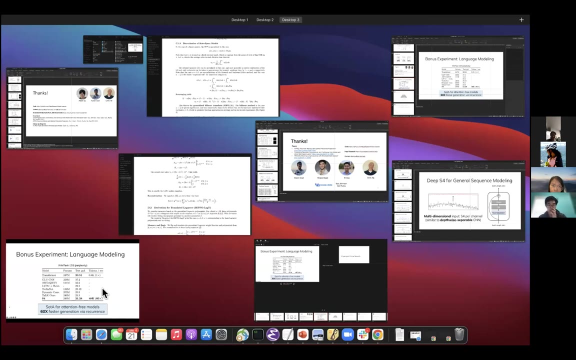 I think that's where transformers really shine and are probably going to be better. So here's a. I don't know if this is the right screen again, Sorry. Anyways, here's the one slide on language modeling where we took a transformer which. 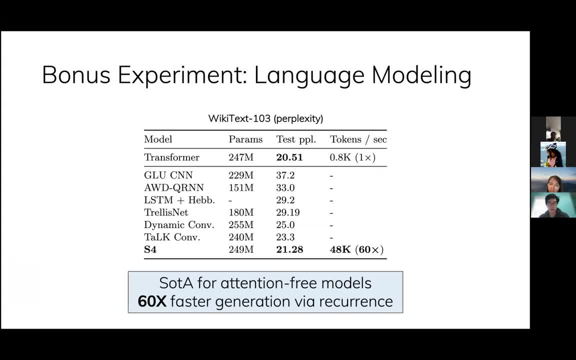 are currently, of course, the best models for Vortex and NLP, and we replaced the attention with S4 and found that it doesn't do quite as well, but it is still significantly better than all non-transformer models And it also has some other benefits. like you can do language generation much faster. 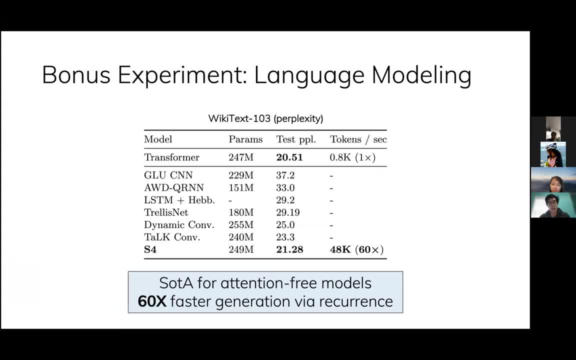 because of the fast recurrent view. That was the main point of this, But this also does kind of point to the fact that, personally, my intuition is that transformers are really good for dense and discrete data, whereas S4 is really good for more like noisy and raw data. 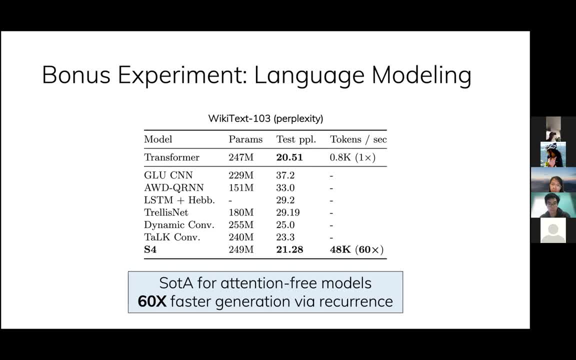 Yeah, And I mean the speed up here, I think is very interesting. Do you know what was the window you would take for language modeling, Like how many token, or words rather, did you consider? Yeah, this one. this experiment was done using a pretty standard length of either 512. 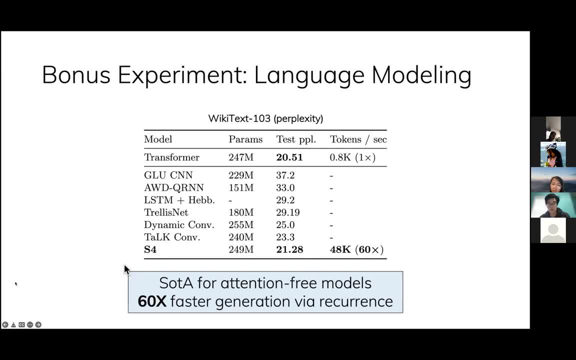 or 1024 tokens. You actually can keep increasing the window length for S4, which only slows it down a little bit and actually improves the performance a little bit as well. But I found that out after the fact and I didn't feel like retraining. 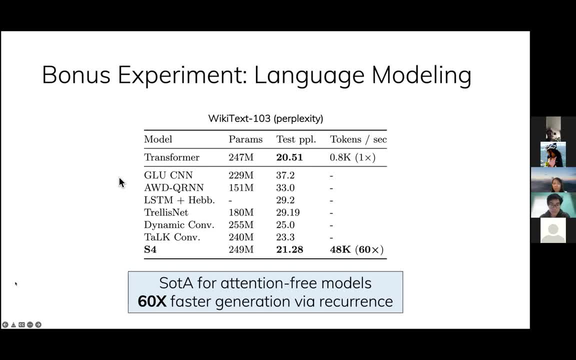 This Okay, cool, Thanks So, but yeah, but the sort of findings of this slide is the speed up. right, It's massive. That was the point that we did this experiment for, but yeah, so there's a lot of the speed.